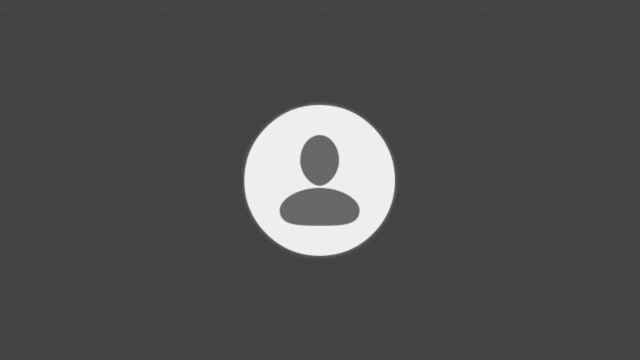 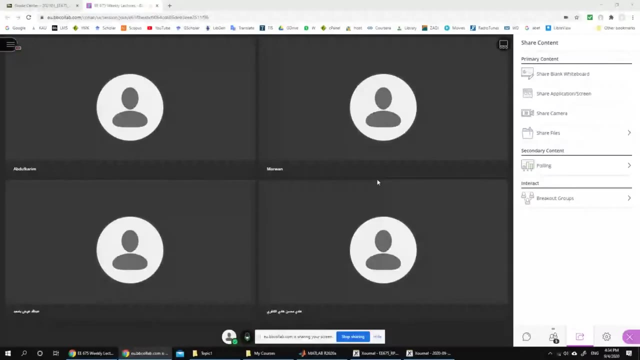 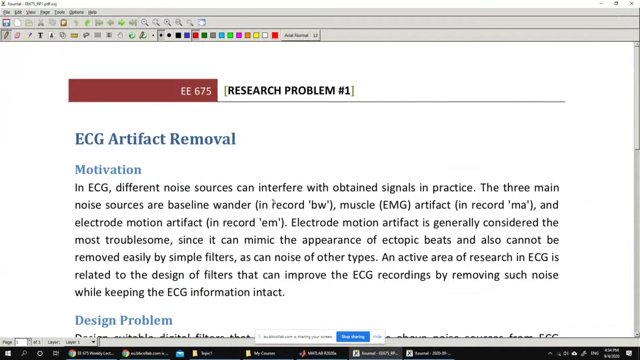 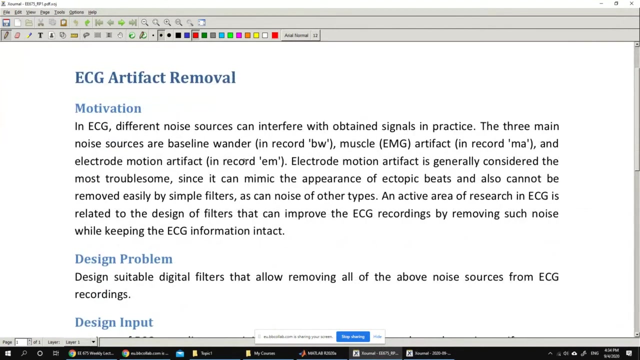 So basically, I hope that by the end of this lecture you will be able to get started on some of the MATLAB experiments so that you can basically at least get in the mood for the next lectures. So basically, we're going to go over the artifact removal research problem and then we're going to try to look at what we're going to do. 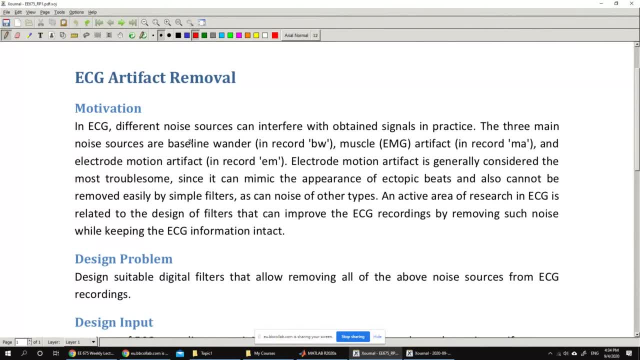 We have the design input for this research problem and then we're going to take whatever we understood from all these and basically get started on one point that would help us or build the ground for us to get started on solving this research problem. First of all, is my voice clear? 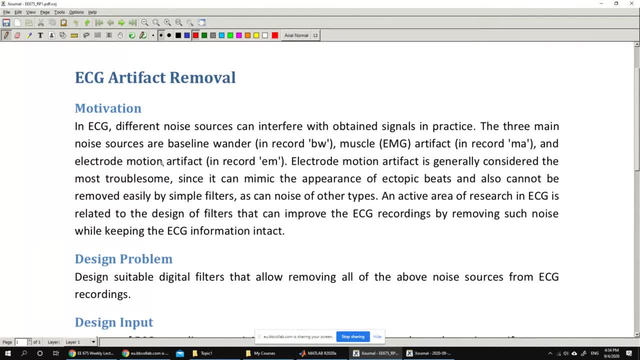 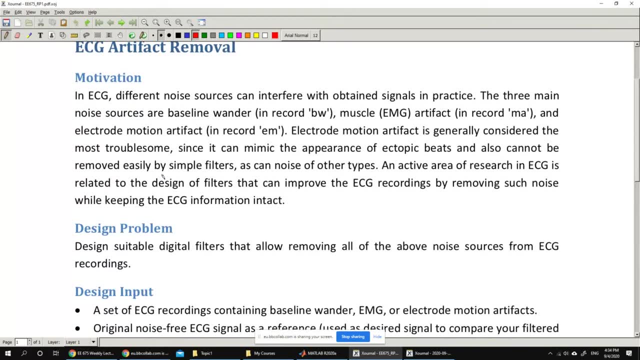 Yes, it's clear, Okay, Okay. So basically, the ECG artifact removal. First of all, does any one of you know how to read ECG? As an engineer, do you know how to read an ECG? So if you look at an ECG signal, would you be able to know if it has an artifact or not? 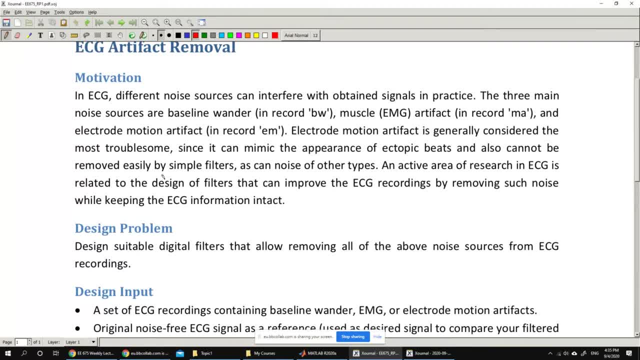 Before doctor. So you learned how to read ECG. I read it- This program- When we are on job. After that we forget it. Okay, so basically you got some experience with ECG from your job. Okay, But most of the graduates. if you have a graduate of biomedical engineering, do you expect the graduate of biomedical engineering to know how to read ECG or basically detect a problem in an ECG signal? 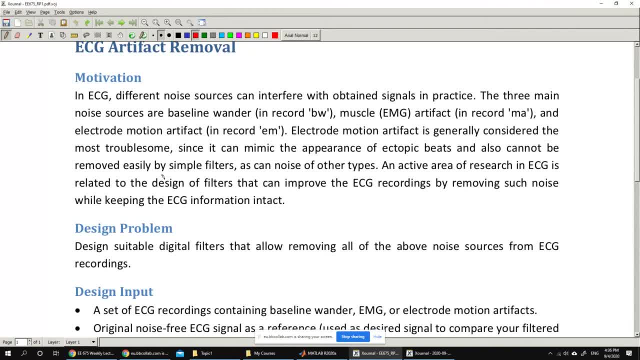 No, sir, I don't think so. yes, That's true. It's very difficult for us because actually we're not medical doctors. Usually, what we know about is how to design an ECG, how to basically build an amplifier that would take an ECG signal from a patient. 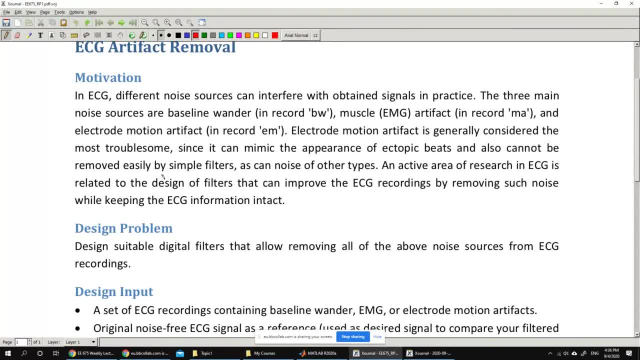 and basically filter it and amplify it to a particular level so that you can either print it or acquire it inside a computer and display it. And other than that, we don't really know what ECG should look like, apart from the very famous drawing of the ECG. 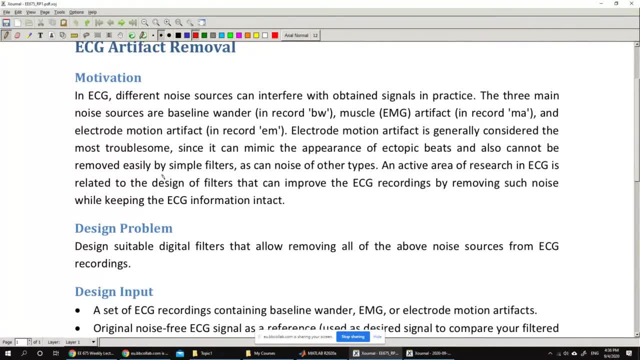 which is actually not exactly how it should look like in all the channels. So basically, we don't really know how to basically at least describe how the artifacts would look like. So basically, we have ECG signals with artifacts and we would like to remove these artifacts. 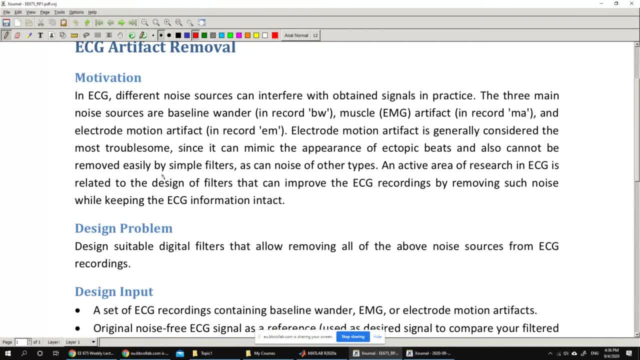 So the logical thing to start with is to know what these artifacts look like. okay, And in order for us to be able to do that, we have to use the services of a medical doctor, who would look at ECG signals and let us know which part is real and which part is an artifact. okay, 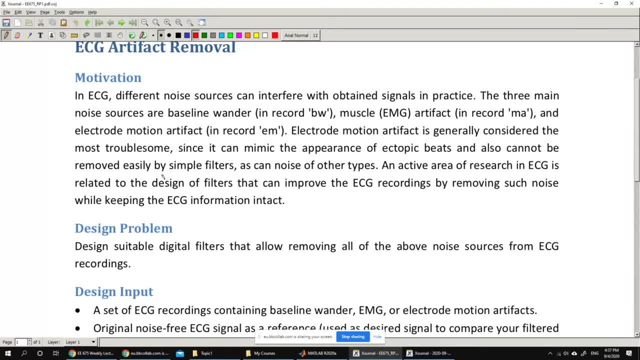 So basically, to start with, the origin of these artifacts is the ECG signal, Basically just noise? okay, We have noise from different sources while acquiring ECG And usually these noise sources will be additive. So basically, when you acquire the ECG from the patient, 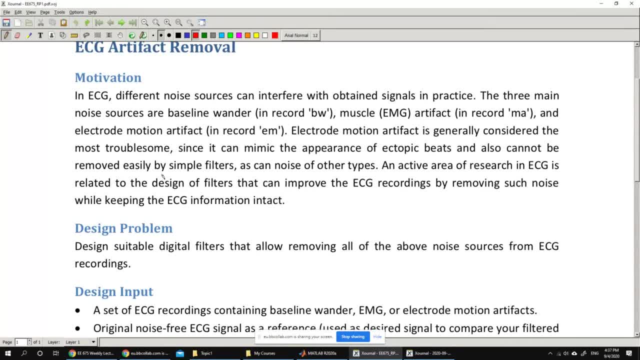 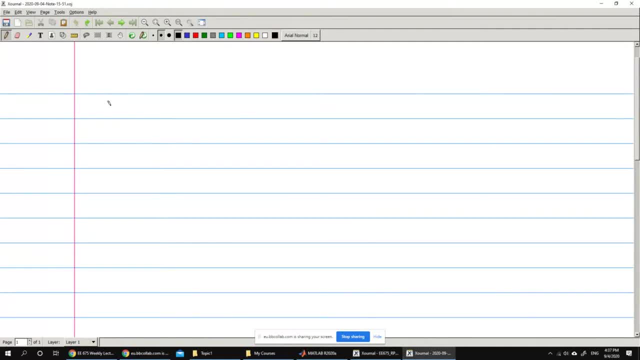 you're acquiring this ECG plus another one, another signal. So basically maybe we can just write the equation for it so that we can understand it better. So basically we have the original ECG signal. Let's just call it X of T. 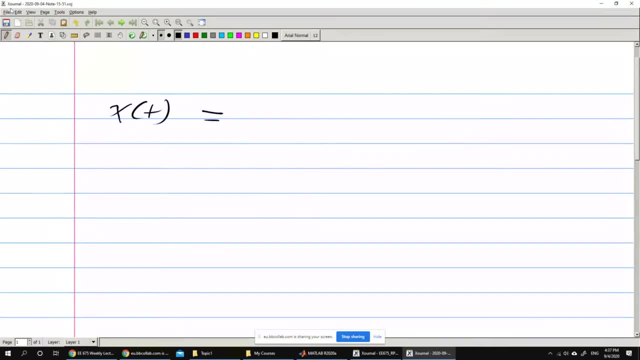 Okay, And this X of T maybe, or basically, this is the acquired signal, is basically ECG signal of T plus noise signal of T. okay, And this noise has many sources. It can be random, random noise, It can be physiological noise. 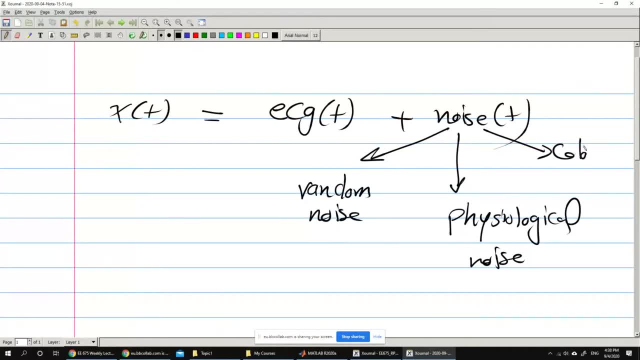 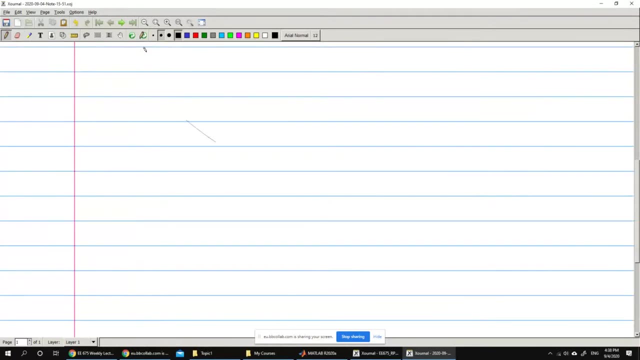 And it can be colored noise from the environment. Let me explain a little bit about each one of these. First of all, the random noise. if you took random noise, basically random noise, Does any one of you know how to describe random noise? 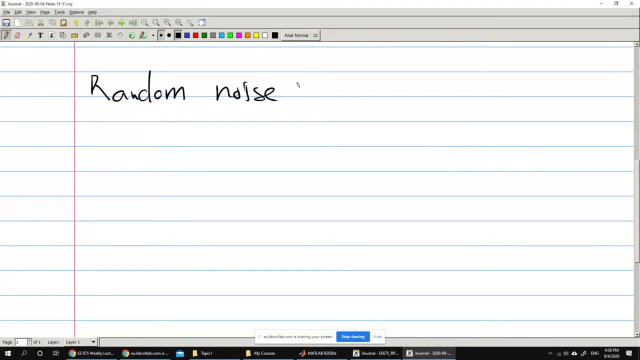 Or where it comes from, Basically the random noise. if you have an electronic circuit, okay at temperature above zero degrees, Kelvin- Sorry, Kelvin actually doesn't have degree, It doesn't have the degree, So it's zero Kelvin- You will have noise. 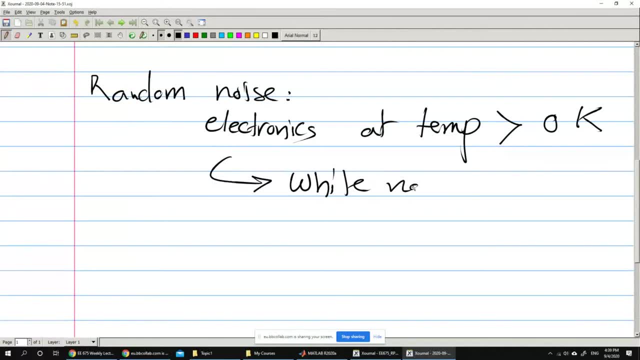 What's called white noise And its origin is called thermal noise. Sometimes it's described as thermal noise. Basically the electrons inside the conductors of any electronic circuit basically have a certain you can describe it as activity, Or basically they do not really conform to basically just conducting electricity. 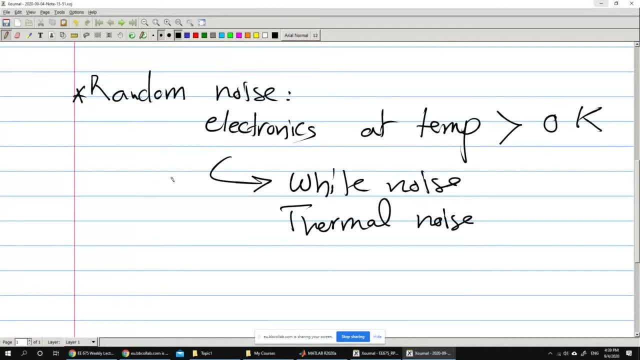 Actually they have. they add some randomness, Random variations to basically the signal that they are conducting And basically this looks like random noise. Unless you have the conductors working at zero Kelvin, you're gonna have random noise. So basically whenever you have a signal and basically 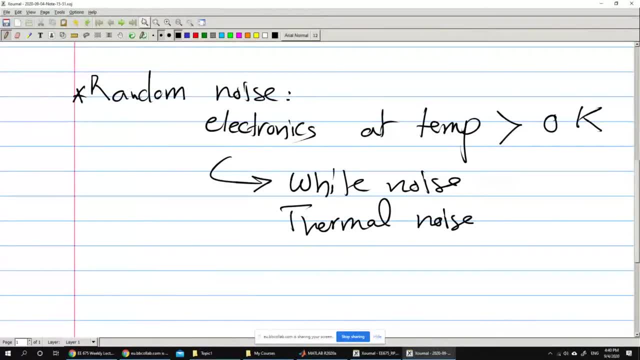 let me draw it as an amplifier so that you understand a bit better. Basically, if you have a signal, an ECG signal, for example, okay, And you enter that Okay, Okay, Okay into an amplifier, whatever this amplifier does, okay. so basically, if you 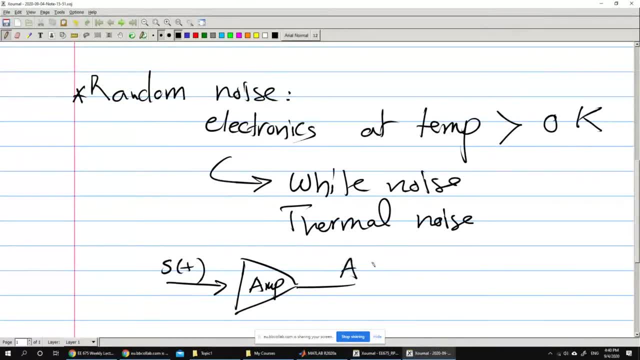 have s of T here. whatever comes out of here will be a s of T, where a is the gain plus noise. okay, you cannot avoid it, you cannot. you cannot do anything to prevent an electronic circuit from adding noise, a signal. so the best thing you can do is basically when you do, when you basically try to choose an. 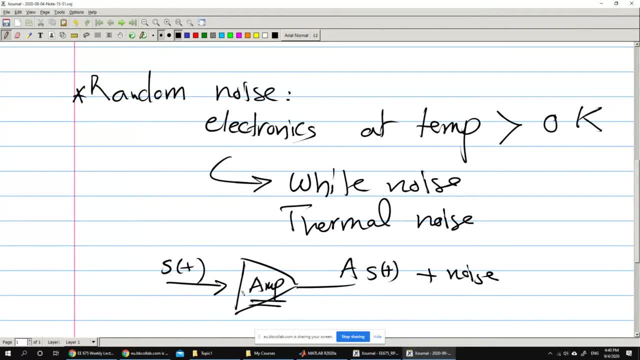 amplifier with low noise. so basically any amplifier will add noise, but certain class of amplifiers would be basically adding the minimum amount of noise. so basically, if you buy what's called linear noise amplifiers, low noise amplifier, okay, then basically you will be doing the best job you can do, actually in order for you to maintain the what's. 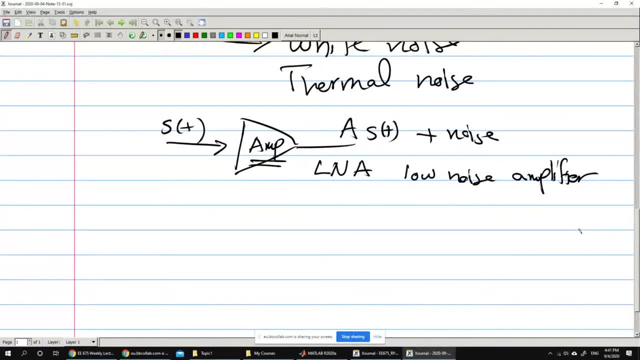 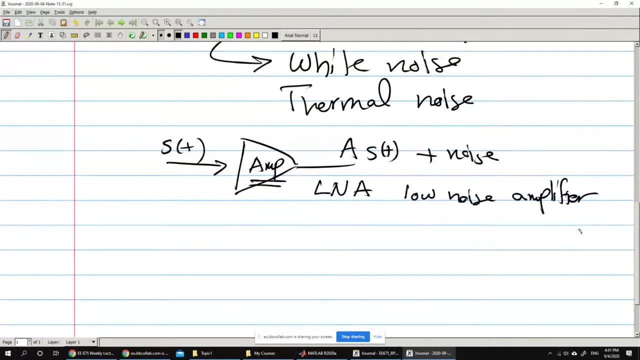 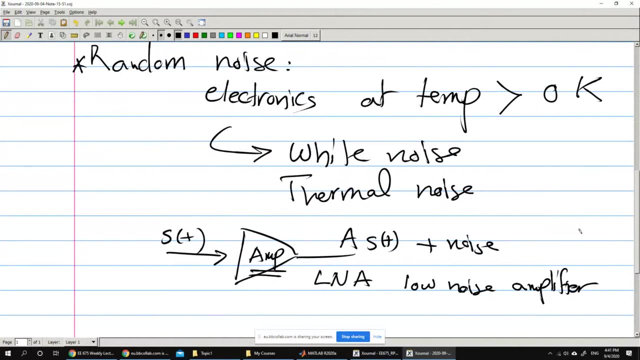 called the signal-to-noise ratio of your signal. okay, but actually it's gonna be there nobody can do anything about. okay, are we dealing with random noise in ECG? definitely we do that. but for random noise you usually have either very basic amplifiers, very basic filters, like we're going to talk about them in a 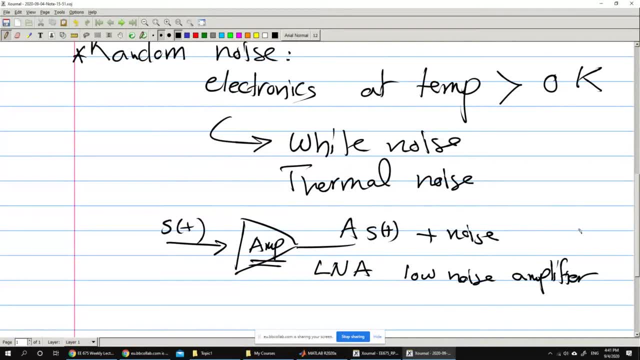 second, we can have them as analog signals in the acquisition and basically in designing the amplifiers with the lowest noise amplifier that we can get. so basically for random noise, the best thing we can do is basically design the design the circuit carefully. so basically this the solution for random. 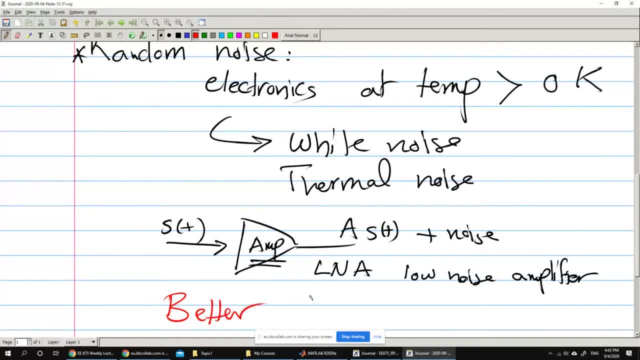 noise is basically better circuit design and basically this is done in all ECG systems that you can find in the market. so basically this is not an issue because we all know that it's present and basically there's not much we can do about it beyond what we can do in the 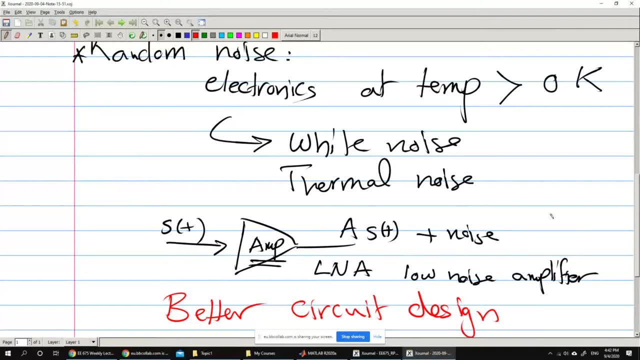 circuit design. so if you have an easy system and this ECG system is already designed, of course, basically you can't really improve the random noise beyond what was done in that design. so basically we're not dealing with that in this problem. we're not dealing with the artifacts from 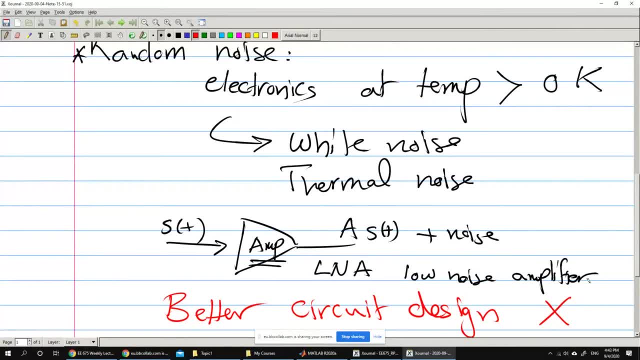 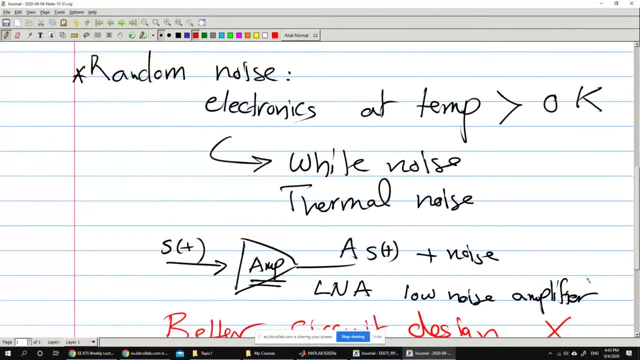 random noise in our problem here, because this is basically. this was already too late. you're having a signal from an already built ECG system and basically you have nothing to do about the circuit that it contains. so we're not talking about random noise. the other class, which is basically 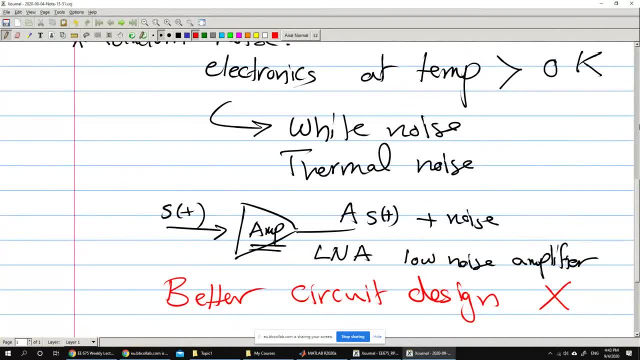 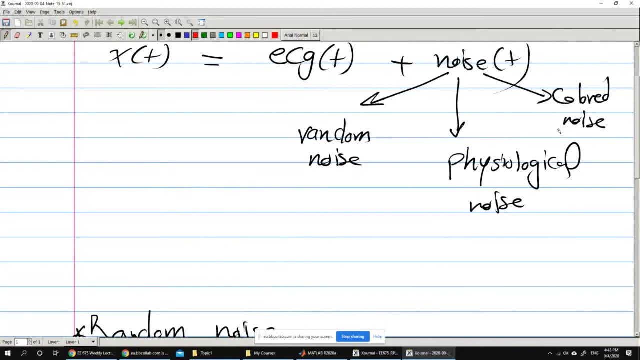 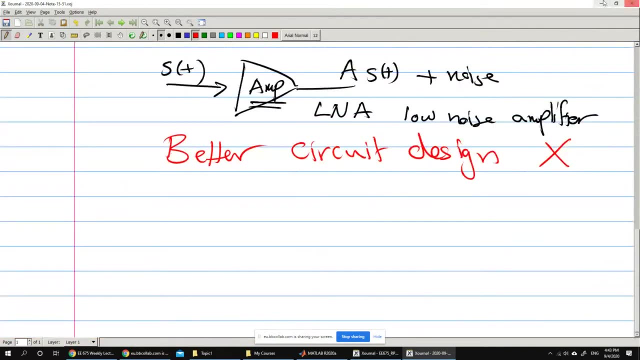 let's consider first maybe the colored noise first, because actually the colored noise is basically some of the thing that you find in the environment. so basically the colored noise. let's write it in a color so that you can remember it. this depends on the environment, meaning that if you have AC and this EC is at 60, 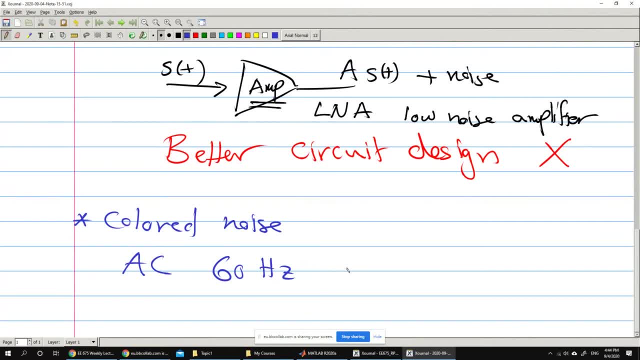 Hertz. basically, somehow you're gonna get your signal, your ECG signal, plus a signal that is 60 Hertz superimposed on it. okay, basically, if you remember at the lab, if you, if you were before in the lab with the oscilloscope, if you don't really put any signal, if you just get the resistance across the 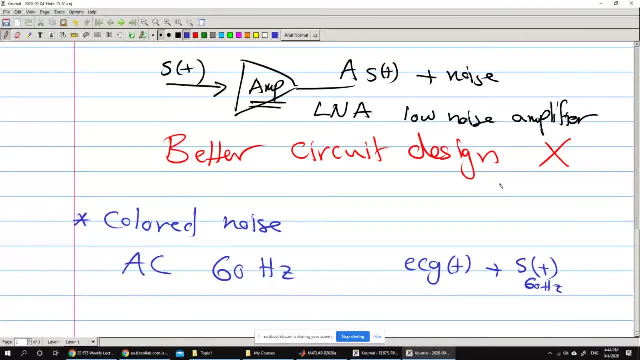 terminals of the oscilloscope. you're gonna see the AC right in front of you and on the source code. this is because, basically, you have wires everywhere in the lab and these wires carry the 60 Hertz signal and basically by basically emission, basically, and basically you're gonna get some component of the 60 Hertz in a. 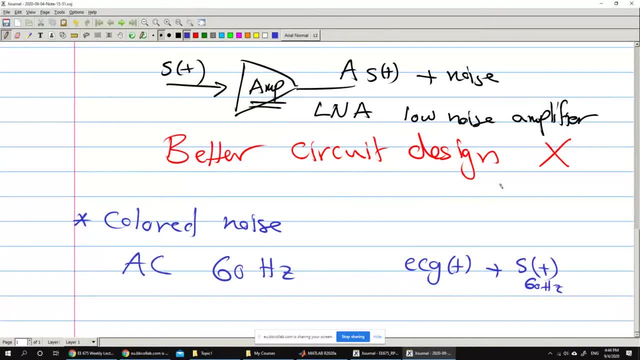 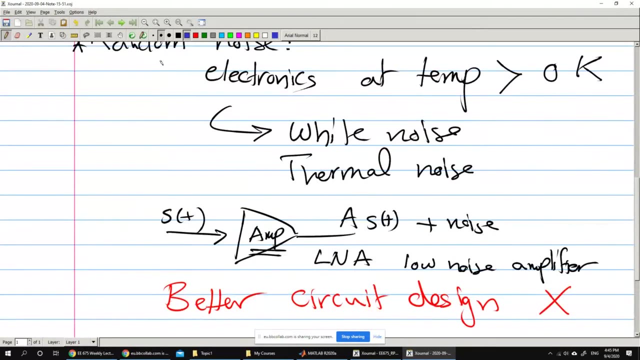 any signal or any circuit that is not shielded enough from the 60 Hertz. okay, so basically this is color noise. why? because basically, when we talk about white noise in the above, in the example above, basically when we talk about white noise, white noise here means that if you look at the frequency spectrum, if you 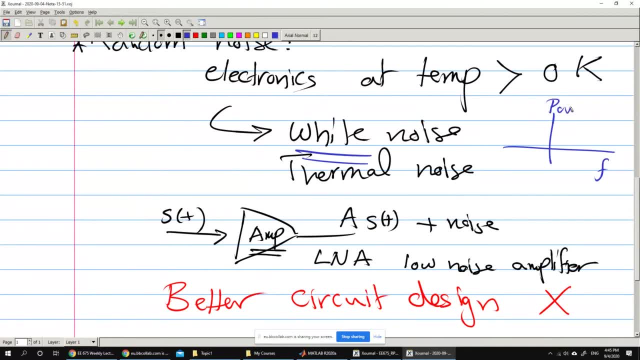 take this frequency and the power of the noise, you're gonna find basically it contains all frequencies. that's why we call it white noise, like the white color, the white light, white light has all colors, okay. so basically white noise comes at all frequencies. okay. for the colored noise, we call it colored because 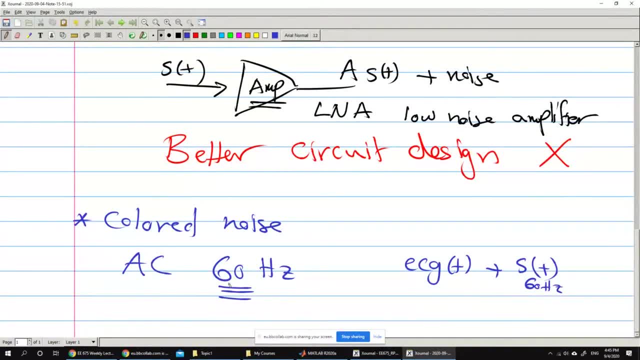 basically it's concentrated at a certain frequency, so it has a certain color. it's not really a color, but actually you just look at the similarities between the lights and the signals, that the frequency, because the red and the blue and green all have different frequencies. okay, so basically it's exactly the same here. when you have AC, we have 60 Hertz. 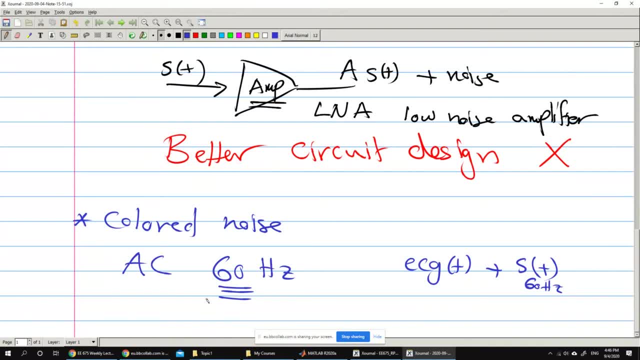 then you know that you have color noise because it has certain frequency, so it's concentrated in a particular frequency, not all the spectrum, like the like, the other, like the like the white noise, for example. so basically, for color noise, this is basically a problem of the environment. okay, and basically, if 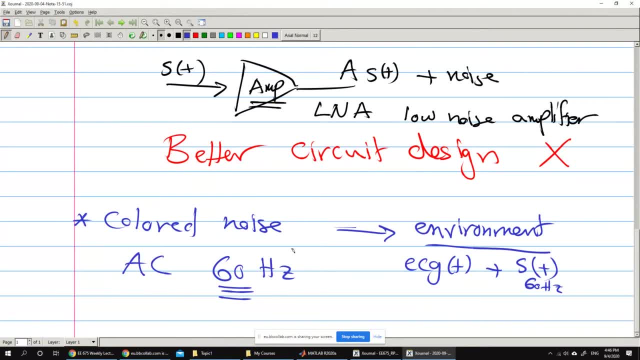 you know that you have 60 Hertz. you have to make sure that the environment is shielded so that when you put an ECG signal there or ECG system there, it doesn't get contaminated with the 60 Hertz that is present, for example, if you 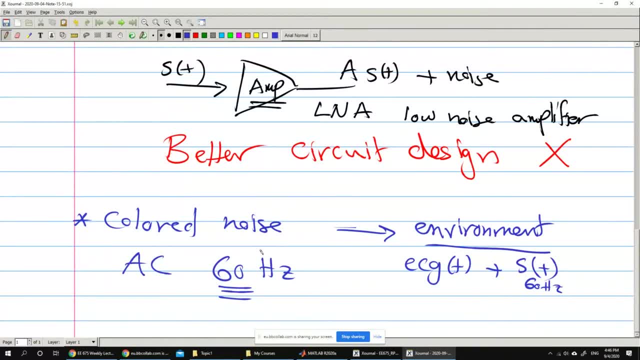 forget about the ECG. if you worked in hospital, if you look at something like the EEG, if you have an EEG in your hospital, you know that the room where the EEG is located must be shielded, because EEG signals are very low and if you have contamination from the 60 Hertz you're going to have a big 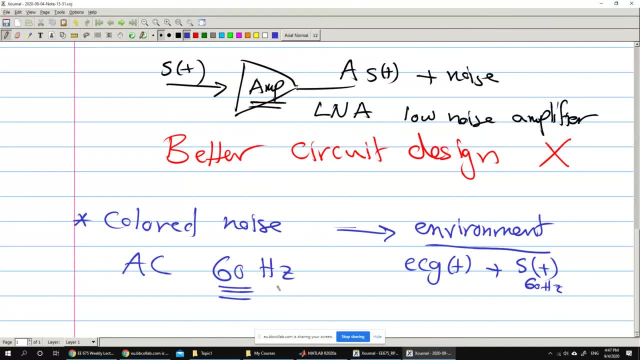 problem. so the colored noise is basically a problem of the environment. usually, when you know that you're going to work with 60 Hertz, you add to your system also, you add a filter that allows you to remove the 60 Hertz. okay, so basically, the environment, you. 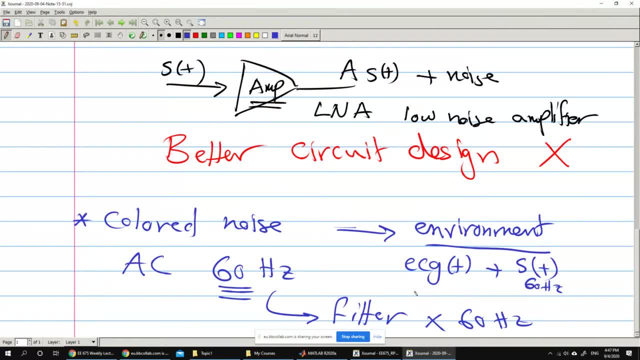 can put shielding there and filter. you can put a filter inside the, the ECG system, or basically, when you buy an EEG system or an EEG system or whatever, you make sure that it contains a filter for the, the AC mains frequency that you have. okay, so basically, 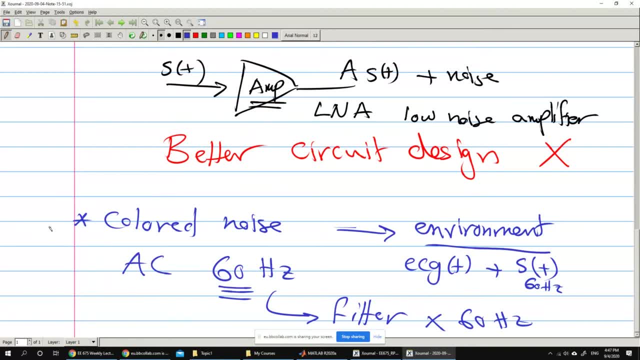 these two types- the white noise and the colored noise- we have a particular characteristics that is different from physiological noise is that they are present all the time. so, basically, this will be present all the time. 100 percent of the time will be there and this also will be 100. 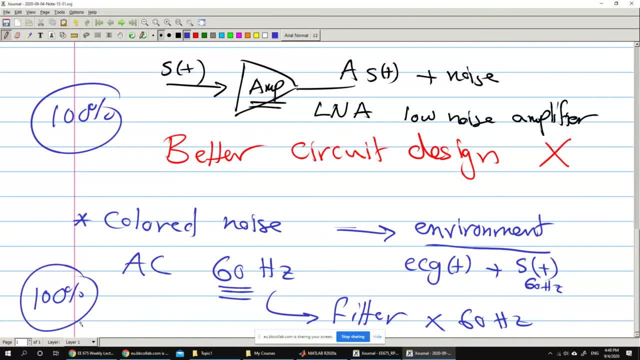 percent of the time it will be there because basically for the white noise, you're using electronics at a temperature of above zero degrees Kelvin. zero degrees Kelvin Kelvin is minus 273 degrees Celsius, so basically you'll never be able to work with or get anything basically even near that temperature. okay for the color noise, as long as you have wires running in. 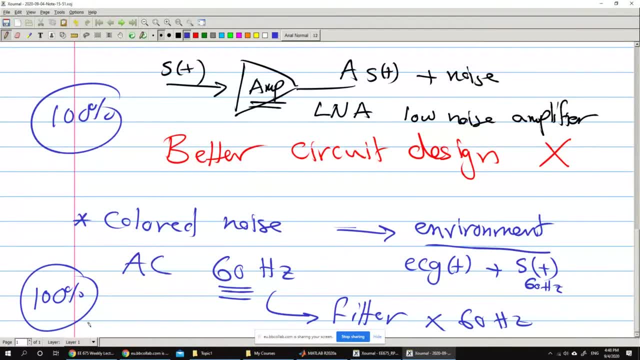 the room where the ECG is located and basically, uh, you're going to definitely have color noise, basically of 60 Hertz. the level of that noise will depend on how the environment is shielded and and how effective the filter inside the ECG system is designed. okay, but they are both basically. 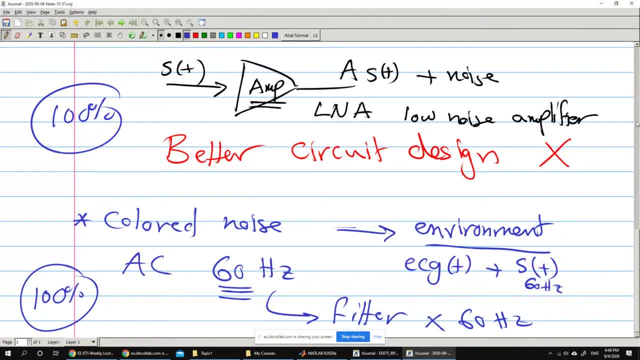 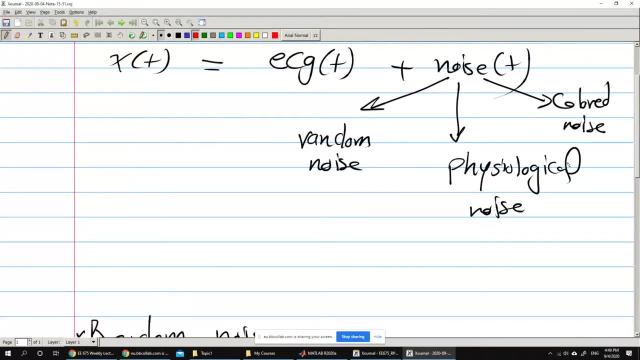 um, they are both basically present all the time. uh, the physiological noise is a little bit different and basically the physiological noise is basically what we're going to be dealing with in this project, because the physiological noise has the characteristic of being, um, let's say uh, basically intermittent. sometimes it's there. 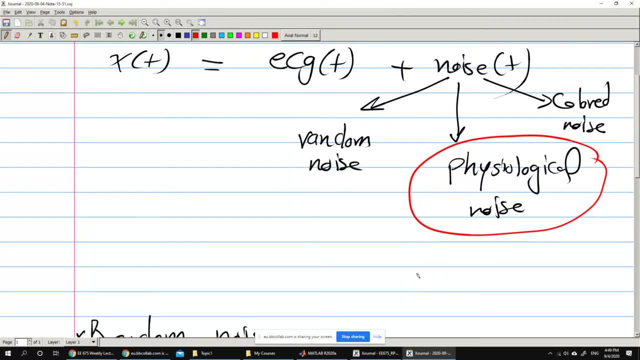 sometimes it's not so it depends on the patient, it depends on the connection to the patient, things of that sort. okay, so all kinds of problems can happen between one patient, another, another, and they are very tricky because imagine that the doctor complains about the ECG having an artifact. 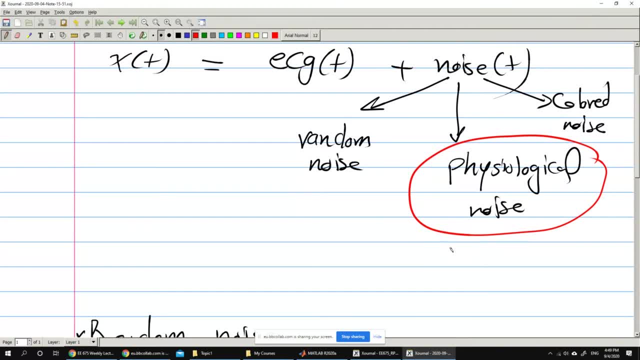 and you go and basically test the same system on a different patient. you don't see anything and the doctor has that. basically I saw an artifact, but I don't see it now. okay. so it's kind of very tricky because basically, basically it depends on the patients, okay. so it's kind of difficult to design, uh uh, you know, to have a particular part. 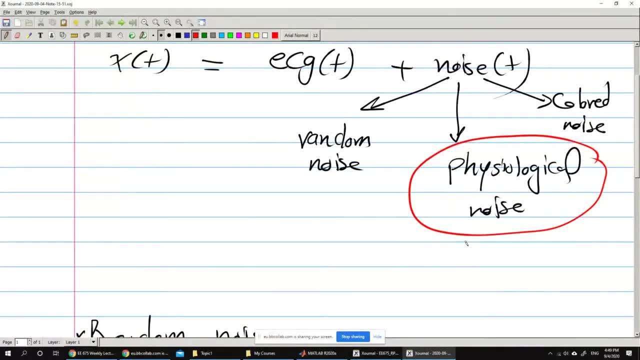 of the design uh uh made, because basically it's, it differs from one patient to another. so basically the physiological noise can come from different things. uh, first of all, the other physiological signals, like, for example, if you have EMG, if you have a diagram, if you put your electrode near a muscle and basically if the patient moves that muscle, you. 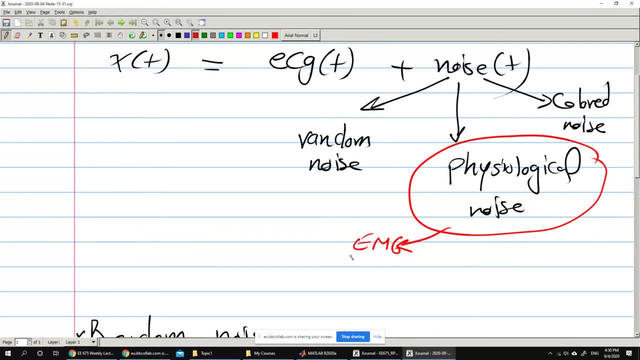 can have- definitely, an EMG artifact- EMG superimposed on your ECG signal. the problem with EMG is that the amplitude of the EMG signal is much larger than the ECG signal. okay, this is a big problem. you can have something. uh, basically you can have other things, like EEG, for example, but actually EEG has. 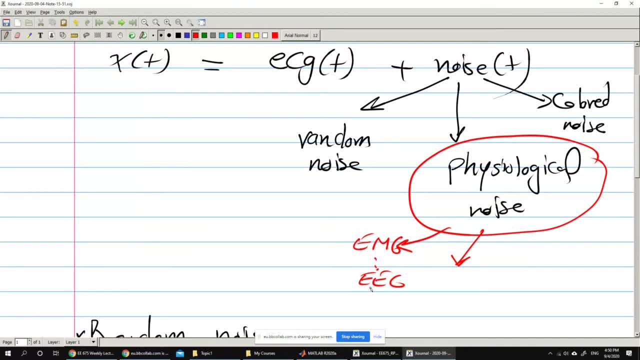 very low intensity. so basically, um, it doesn't worry, it doesn't really cause any problems for us because ECG is much stronger, but the EMG is definitely a problem. another problem for physiological noise is um, basically, if you have motion, the patient motion, basically the electrode interface that takes the signal from the patient. 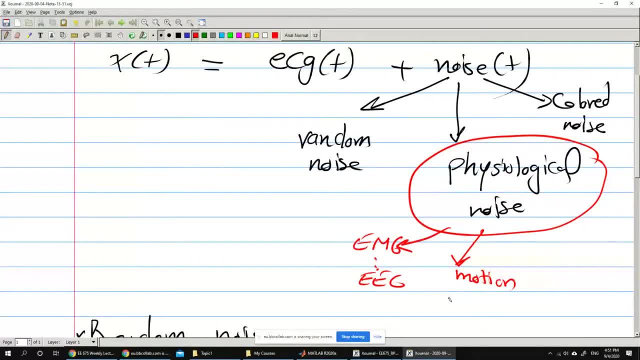 to the ECG system. basically it has a model. this model has a resistance capacitance. when you have motion, this model gets perturbed, it changes, okay. so basically it changes the magnitude of the signal and basically it changes the magnitude depending on the motion which basically causes an artifact to appear where, basically, in certain locations, the intensity is. 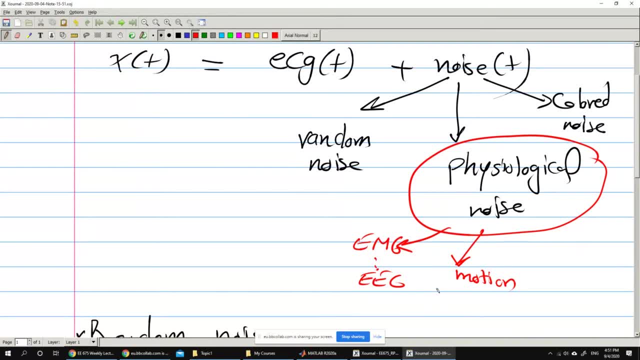 higher. certain location density is lower, so basically it's a problem. so, basically, you make changes to the ECG signals that are not dependent on the actual signal that comes from the patient. so this is a big problem, okay, uh, there's another, uh, another problem that may come from from electronics or may come from the interface itself. uh, it's called. 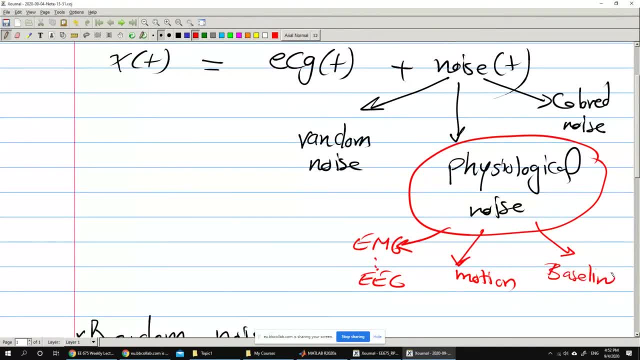 like baseline wonders. uh, if you remember also what you did in in the lab, sometimes you have a signal and this signal appears nicely like this: okay, sometimes you see that you see this signal. you have your own signal, the signal that you want to work with. okay, like, for example, if you have something that would look like that, maybe I should take it somewhere. 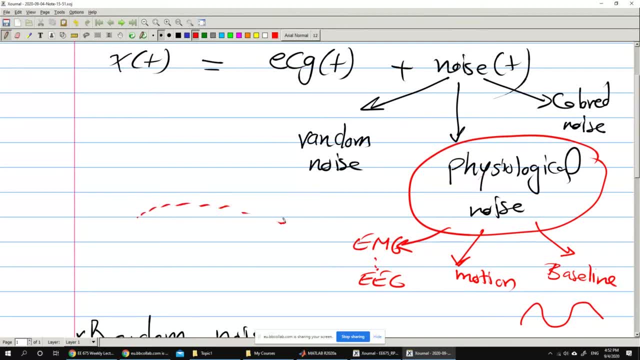 um, that's fine. basically, you're gonna have a very slow moving baseline and basically your signal is superimposed on that baseline. it's basically. it's not superimposed on a baseline, that is fixed, okay. this can happen because of several things actually, but usually you have like a capacitive 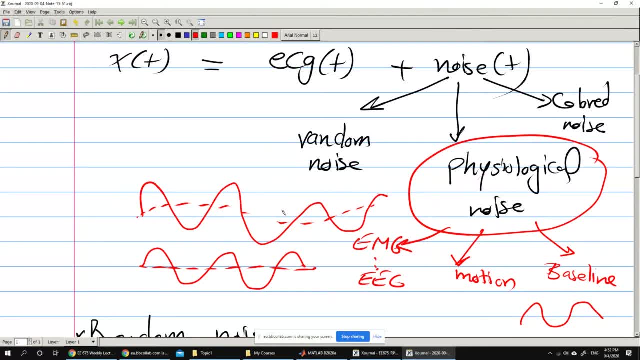 effect somehow and basically it's related to the way the system is designed and the way that could. the electrode is the patient. but the problem with something like this is that we have a problem when we try to interpret the ECG, because sometimes, in order for you to diagnose or for the doctor, 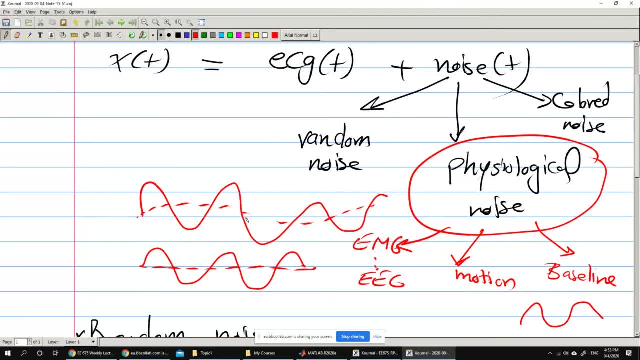 to diagnose the ECG. he looks for the level of particular segments of the ECG signal. so if the level is elevated, it can basically be a certain disease. if it's depressed, then it's another. so when you have a baseline drift like this, this is a big problem. okay, so basically these three. 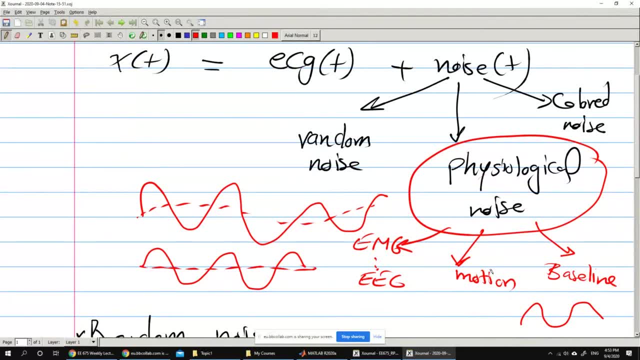 types are the three types we're going to consider? okay, and basically we assume that the model of the noise contamination is linear model like this, like additive noise, like this, and so we are going to try to take care of them. okay, you have any problems about you? understand what I, what I'm saying? 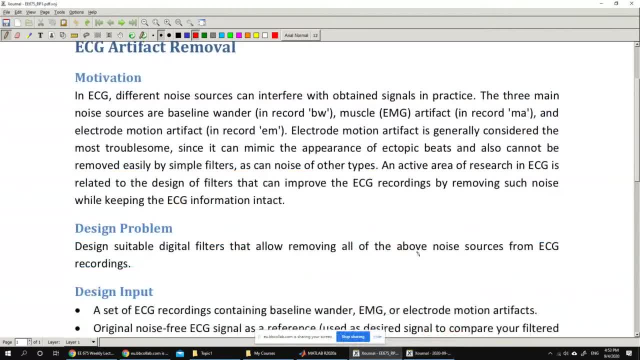 okay. so basically, as you see here what we're going to talk about, we have different noise sources and we talked about. we're talking about, first of all, the baseline wonder we're going to talk. basically we're going to talk about muscle problem, which is EMG, and basically we're going to talk about. 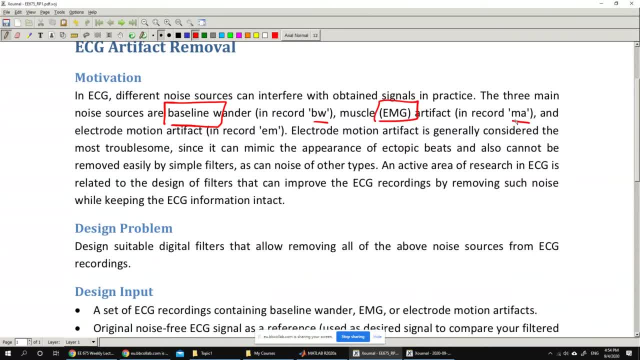 basically, this EMG artifact is basically going to be termed MA muscle artifacts- and you have the electrode motion, which is going to be basically EM, which is electrode motion. so basically these three artifacts are really very tricky. so basically, you have a database, people have a database with signals of each one of these types and they basically in order for people to 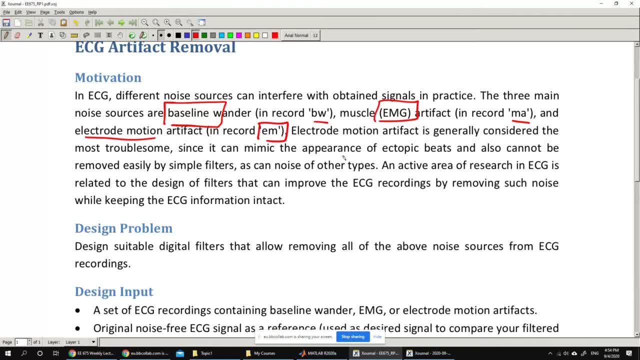 understand how the artifact looks like. they basically give the actual signal, that the true signal and the signal with the artifact, so that you understand the difference between the the signal with the artifact and the signal without the artifact. okay, so basically what we're going to try to do is understand first the type of artifact and then try to get started on filter. 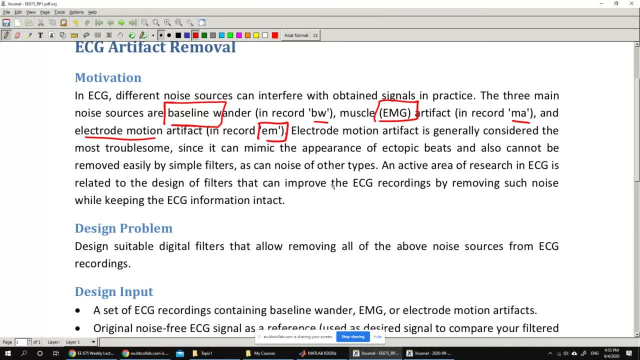 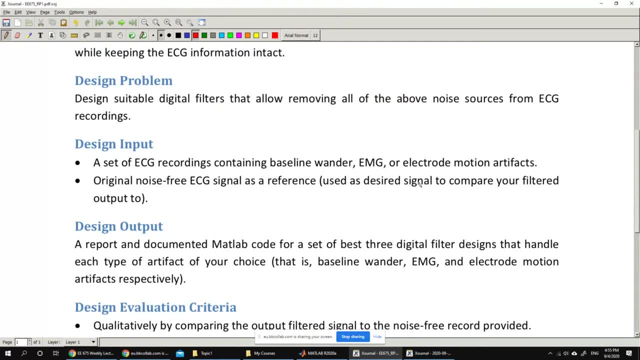 design, digital filter design in order for us to be able to to basically remove this article. okay, so, uh, the design input that I gave you for this problem is just basically a set of ECG recordings containing these types of artifacts and the original noise-free ECG signal. so, basically, 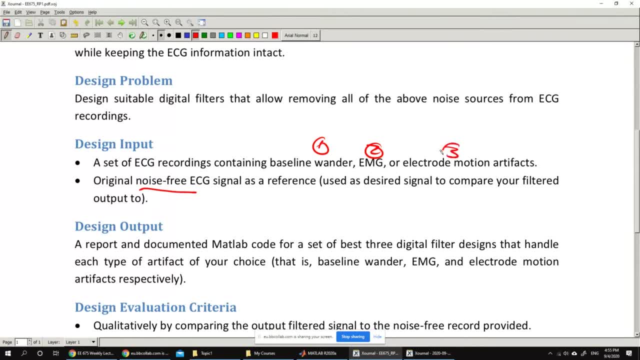 you have the first type, second type, third type and the noise-free ECG signal. okay, and basically, from these two, we're going to try to understand exactly what the artifact looks like. and when we know exactly how it looks like, then we can get started on designing a digital filter that would allow us. 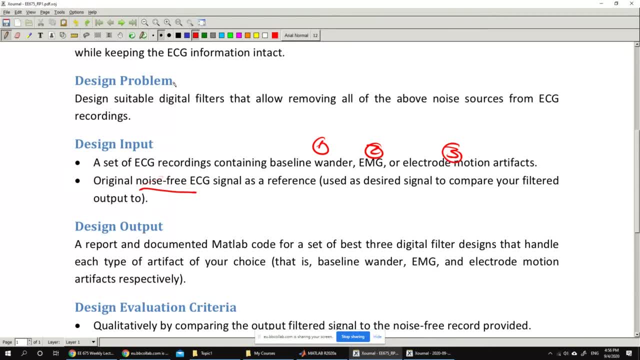 to do that usually? uh, first of all, we, we, we determine that the signal is additive. we're going to need a filter to be able to remove it and basically, this leads us to basically the tool itself. the digital filter design is a tool. okay, how many of you know? 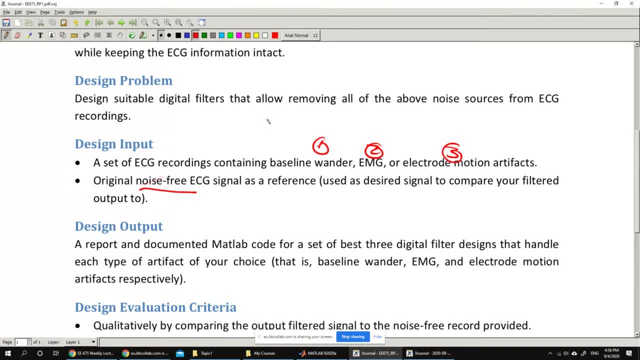 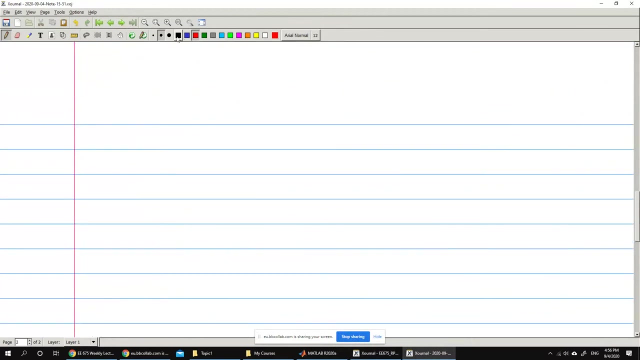 how to design digital filters. anyone knows? if you know, just let me know if you know. if you know how to design digital filters, okay, nobody, none of you know how to do that. so basically, uh, first of all, we determined that we need a filter and since we're going to do it on a computer, 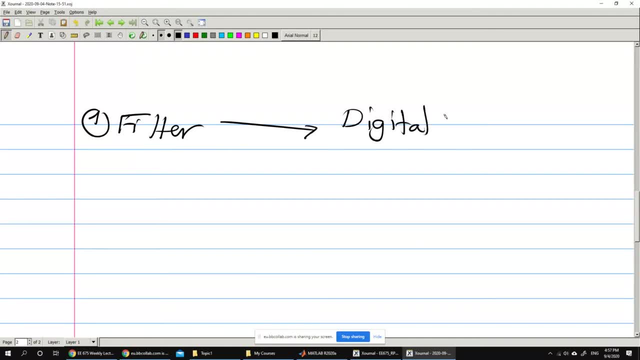 then because your signal is digital, we need digital filter. so basically, we need the theory for this, we need to know how to do that. okay, number two in order for us. if you basically learn how to design digital filters, should you just go ahead and try it on the signals? 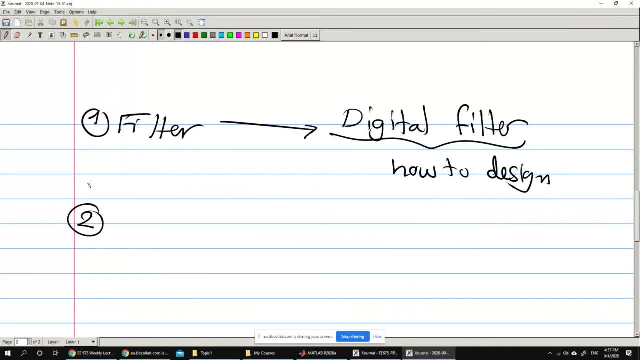 and that's it. actually, in order for us to make sure that we know what we're talking about, know exactly how to design the digital filters, we're going to basically try, try the digital filter on something we know. this is the best way to learn things. so, basically, if I wanted to amplify a 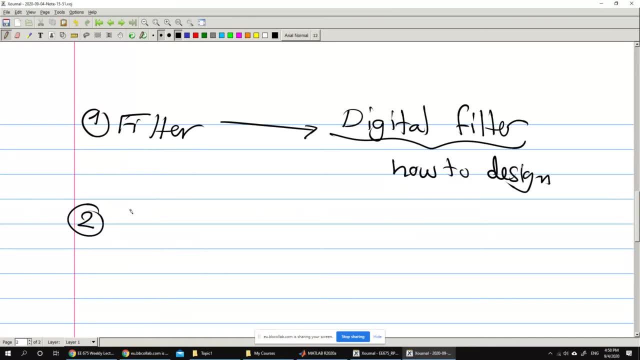 signal: okay, design an amplifier: okay, I basically try or test this amplifier on a sinusoidal signal. okay, why should I do? why do I do that? because basically, I know the sinusoidal signal, how it looks like. I know if, if it gets amplified, I can detect the amplification from the amplitude. 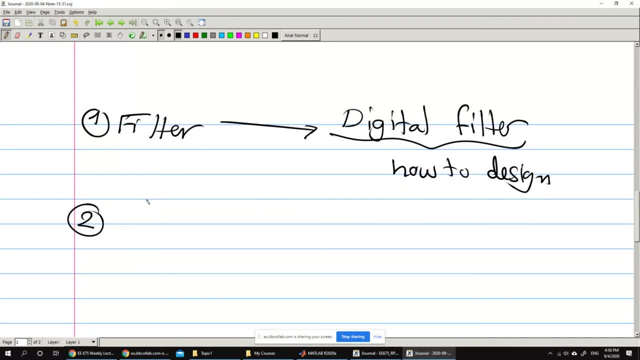 I can actually look at the sinusoidal signal and see if the filter or the amplifier did any modification to the signal or distortion to the signal, because it's actually I know how it looks like. so basically this would lead that to something called simulation. basically we're going to simulate signals and make sure that the digital filter we design works. 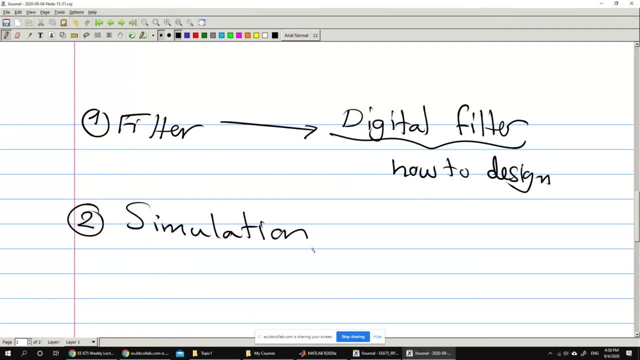 with these signals. for example, if I wanted to design a low-pass filter, you know how the low-pass filters look like. okay, you know low-pass filters. I would assume that all of you know low-pass filters. what does a low-pass filter do, do? basically, it has a cut off at a certain frequency. so basically, you have, for example, you have- cut off. 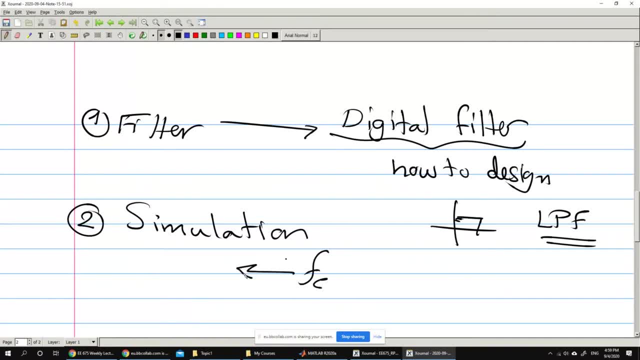 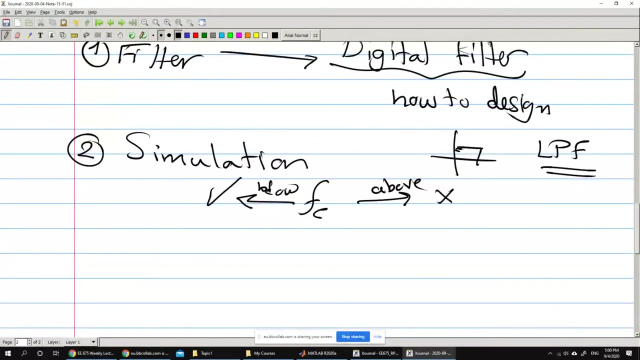 a frequency: FC. if you are below FC, you get cut off. if you are above- sorry, it's exactly the opposite- okay, if you are below that frequency, you get passed, if you are above, you get cut off. okay. so basically, what I can do is basically design or simulate two signals. 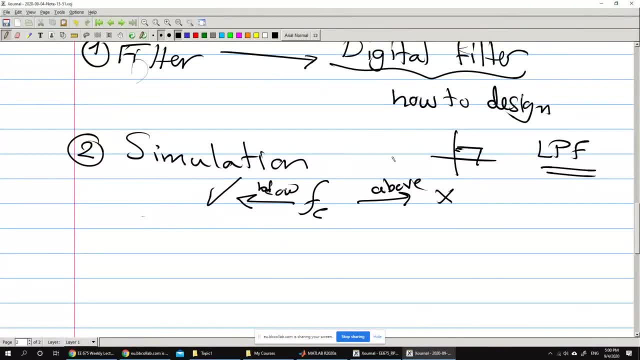 basically, if you have a signal, uh, like a sinusoidal signal with frequency 10 Hertz and another with frequency, for example, 30 Hertz, okay, two signals, the signal one and signal two. okay, and then I design a cut, a filter with the cutoff frequency of, for example, 20.. 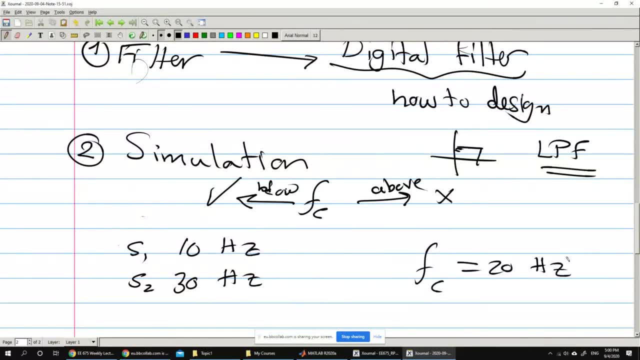 what should I expect if I pass the summation of these two signals to that filter? what would happen if I pass the signal of 10 Hertz? what would happen? don't pass right, yes. and if you, if you pass the 30 Hertz, it should not right. 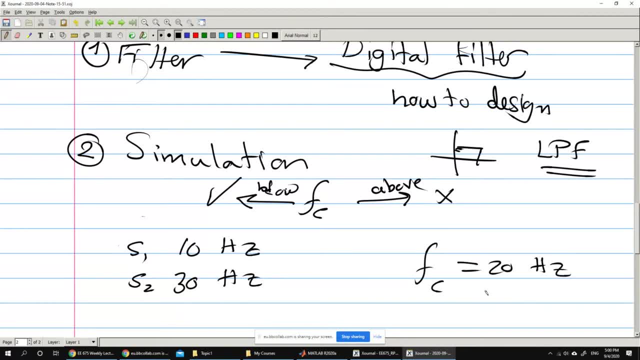 so, basically, if we do that, if we do that and design the low-pass filter with 20 Hertz and it works, then I know how. I know that I actually know how to design a low-pass filter if I want to do the opposite, if I want to pass this one. 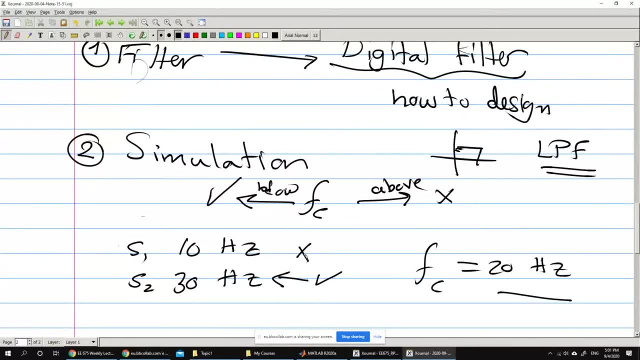 and high-pass filter. we use high-pass filter. so basically this is basically a test of how we design digital filters. if we know how to do that, then basically we can actually proceed to understand the characteristics of the artifacts and see whether they will need a low pass filter. 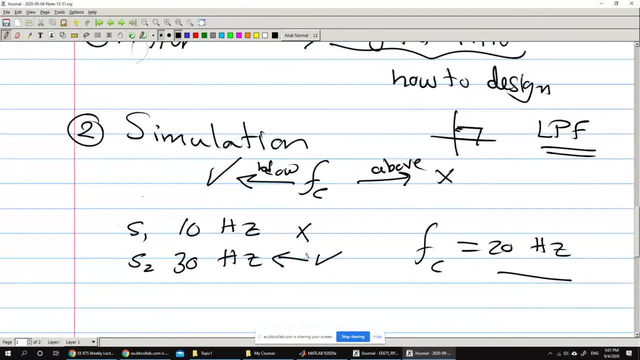 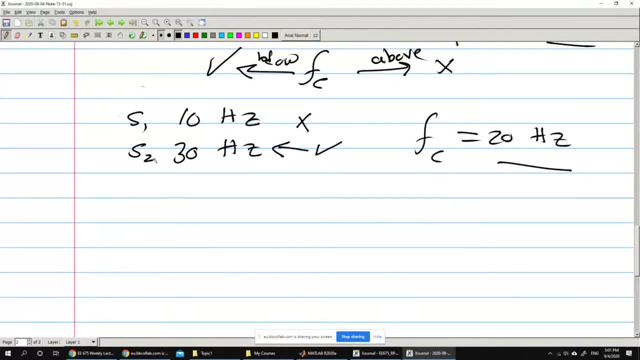 or a high pass filter. so basically, once we get past the simulation step, we here know how to design a digital filter. okay, so basically the third step is to look at the artifact and basically by looking at the artifact I would like to basically estimate the properties of the digital filters, or maybe I should say specs, maybe I could- should write it in color. 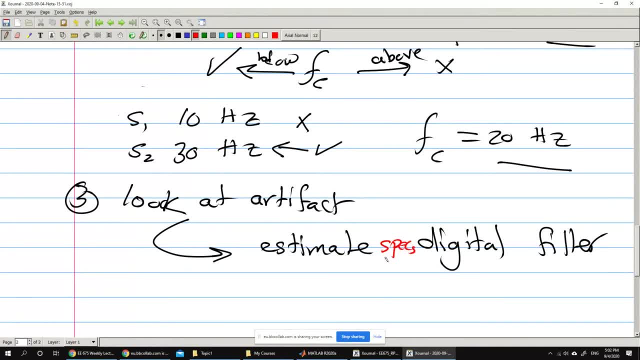 the specs of the digital filter that we need. so, for example, if I have a certain artifact that looks like it has high frequency, okay, then, in order for me to remove the high frequency, I would like to have a low pass filter. if I have an artifact that looks like a low frequency signal. 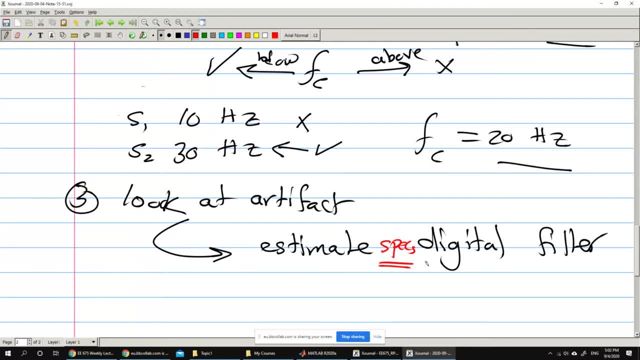 then I would need the opposite. I would need a high pass filter. okay, if there is an artifact that has both characteristics, then I might be basically thinking about a bandpass filter, okay, so basically, we're going to look at the artifact. I'm going to show you how to look at the 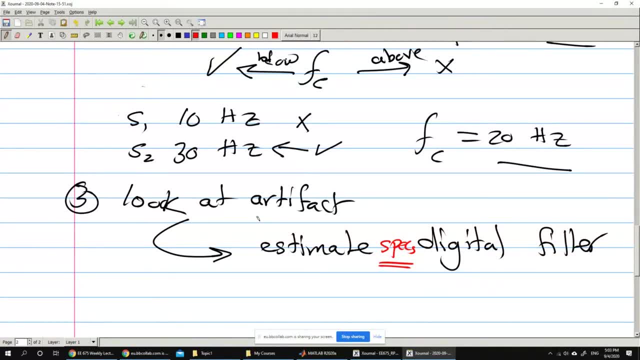 artifact and basically from what you see in the artifact, you try to estimate where you should go with the digital filter. after that you get started with designing or basically applying things to the new filter. so after you finish that step, so basically what you're going to do is- 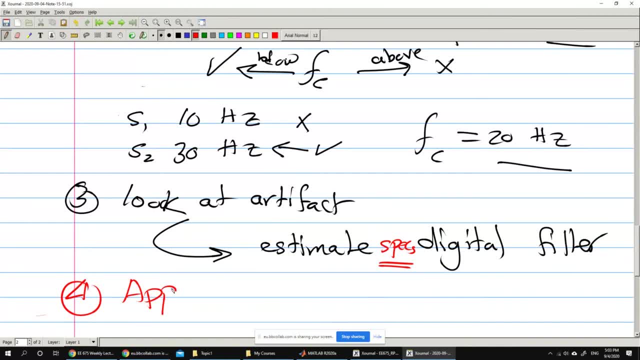 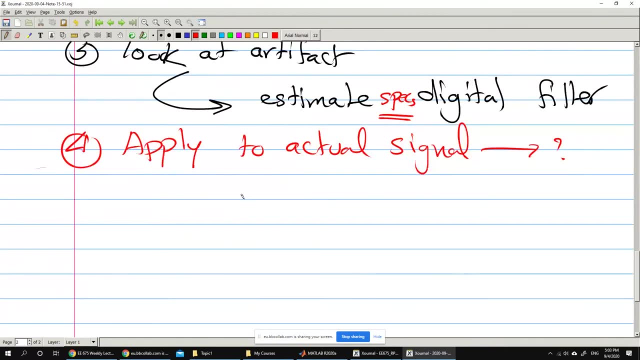 basically, you're going to apply the filter to actual signal and see whether it works or not, and this will likely involve experimentation, meaning that it's not going to work first time, you have to adjust it a little bit, okay, so basically, you have to use experimentation in order for you to be able to optimize the filter. 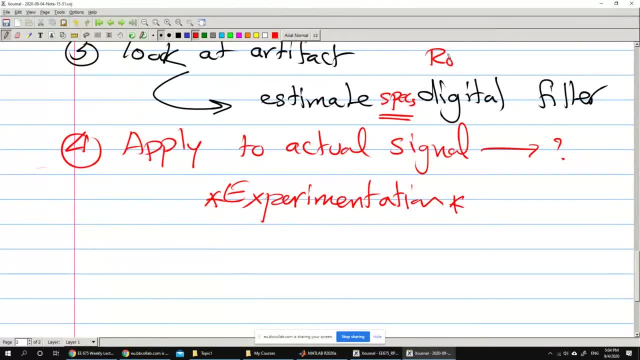 characteristics, you get something that is rough. you need rough estimate here from from this part here, because basically I told you that a low pass filter would work. low pass filter, you can start from 0.001 hertz low pass filter to maybe one giga hertz low pass filter. okay, where exactly do you start? 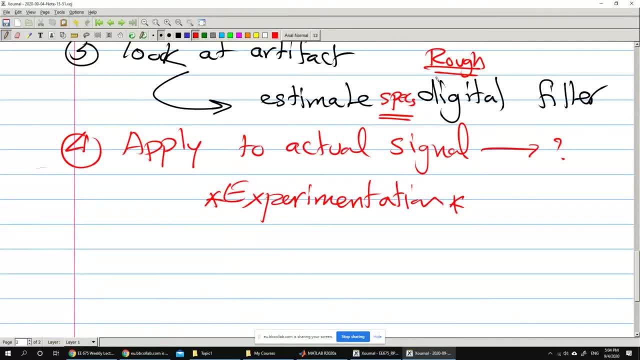 you have to get a starting point. when you look at the artifact, you're trying to get a starting point that is as close as possible to what you would actually end up using. after that, you optimize it using experimentation. after the experimentation. what you need to do is basically: 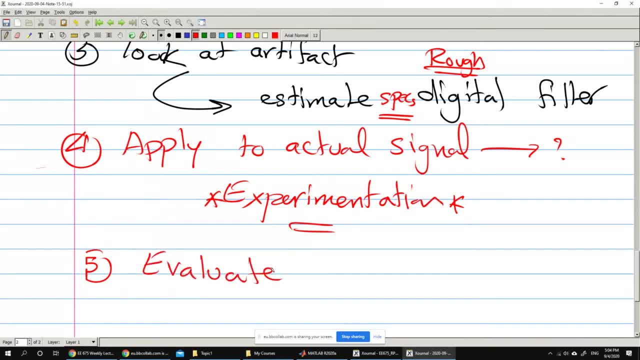 evaluate the experimentations. so basically, you try to basically select or optimize based on certain criteria, so that when I, when I ask you why you designed the filter that way, why you chose the specifications of the filter that way, you tell me that I optimized this particular criteria. okay, and basically this is how people do it: actually research, okay. 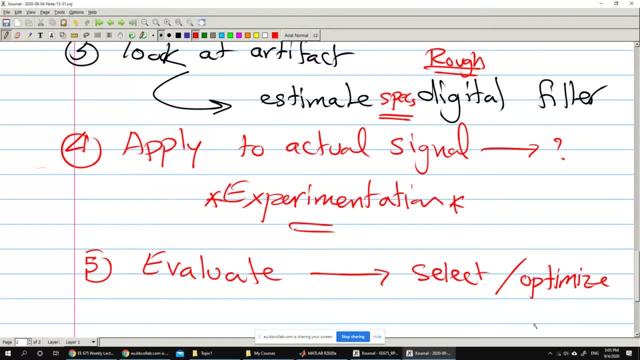 because there are so many different filters. each one of the filters that is available would actually optimize a certain criteria. okay, so basically we're going to talk about how to evaluate these criteria, or basically how to which criteria first of all are important, and how to actually try to implement one of these criteria so that we can evaluate. 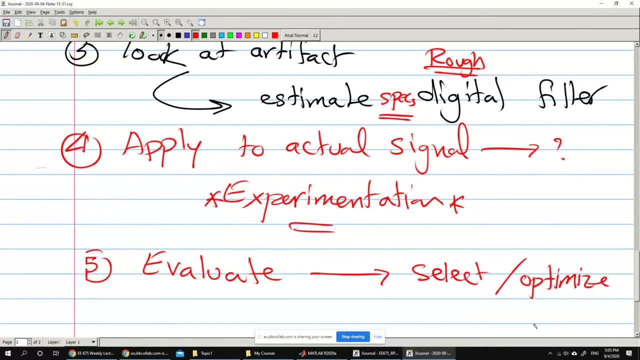 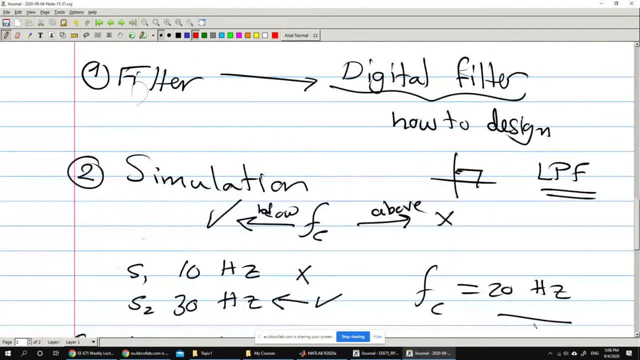 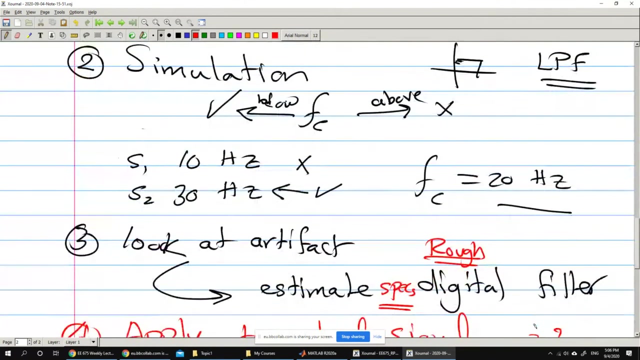 our experiments based on it. okay, so basically this is like the road map. uh, do you have any questions about how to proceed in solving this problem? so basically, as i told you before, we need to learn about digital filters, how to design them, how to apply them. we need to do some simulations in order for us to make sure that. 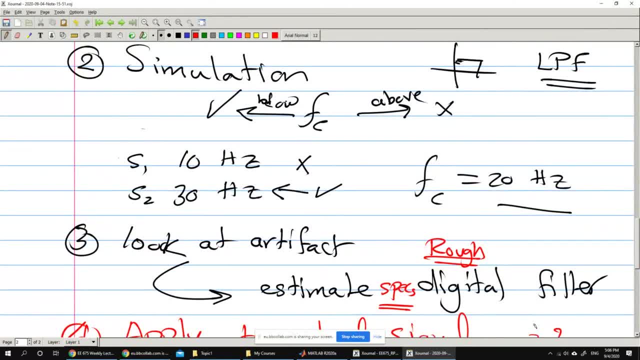 we know how to design digital physics, because this is the main tool we're going to be using to solve this problem. so, basically, we want to make sure that we understand it first before we apply to our problems. if you don't do that, by the way, sometimes you end up with results. 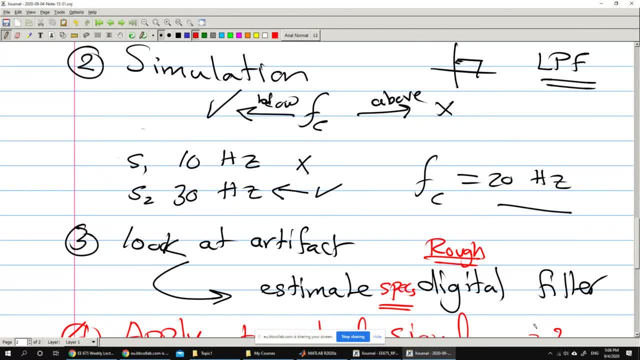 that don't really look good. okay, and the problem is, if you don't really, if you're not confident about your digital filter design skills, then the problem may come from the poorly designed digital filter. you didn't know how to design the filter, or it might be the specifications of the 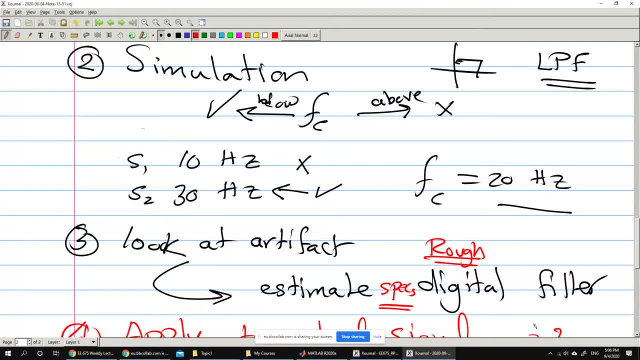 uh, improvement a little bit, okay. so you'll never be able to discriminate between these two. unless you make sure with simulations that you know how to design a filter, you're you're not going to be sure how to evaluate or where the problem that you might end up having. 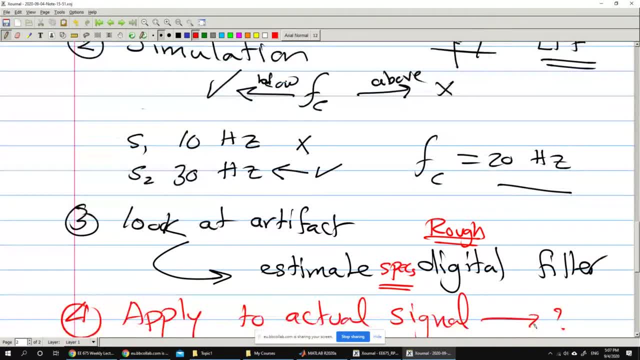 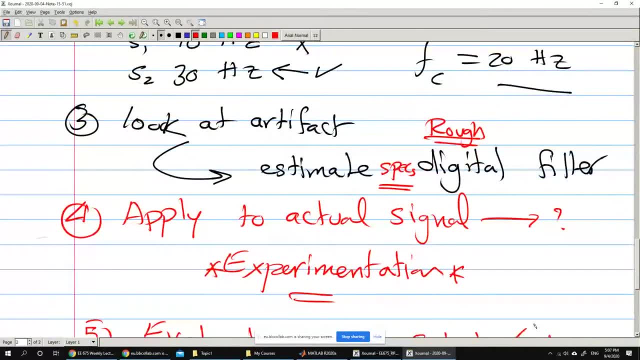 may come from. okay, so we're going to do simulations to be able to uh verify that we know how to design digital filters, and we're going to look at artifacts, the basically the artifacts that are present in the signals, and basically uh try that or basically estimate the specifications of. 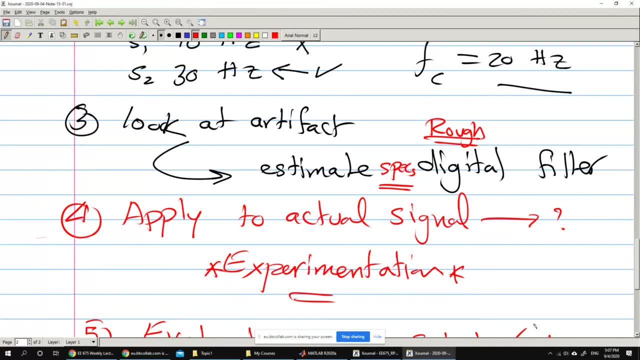 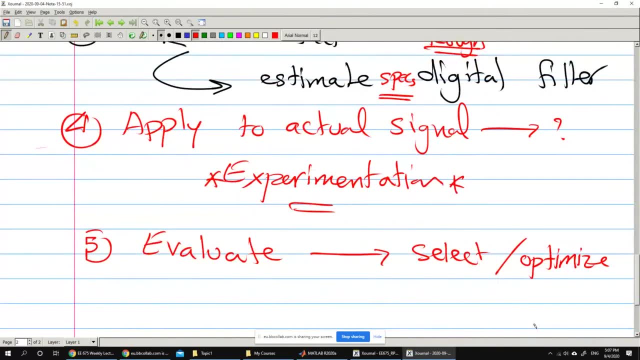 a proper digital filter that would work well to remove the artist, and then we apply to actual signals and evaluate and basically the goal is to optimize. is that clear? yes, clear, okay. so basically let's get started on the code, the matlab codes, okay, first of all, in each one of the research problems that we have, 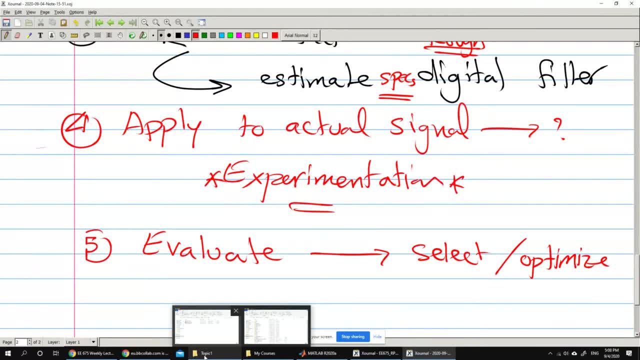 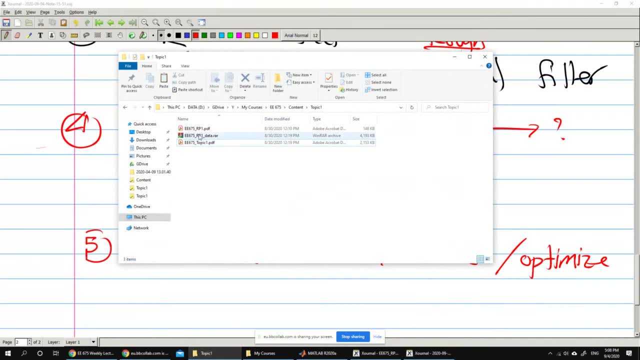 i give you some data and some initial code in order for you to be able to start, or get started with your data. let's get started with that. so basically you have that. basically, all these things are the things that i put in on blackboard for you. so basically the part with the data here. 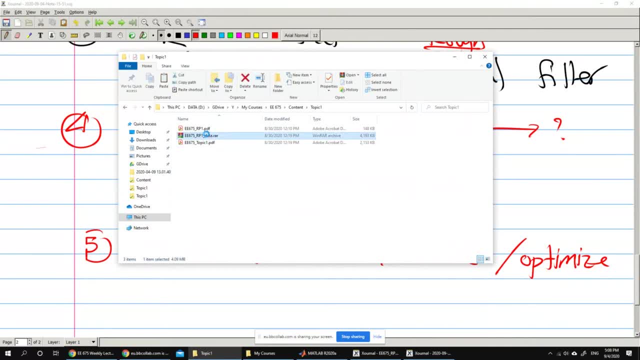 uh, what i'm going to do is just, uh, unzip it, uncompress the file. so basically, i'll extract it here. so basically, uh, you have an ecg signal or ecg folder right there. please do exactly as i'm doing right now. so basically, after this lecture, please try to basically: 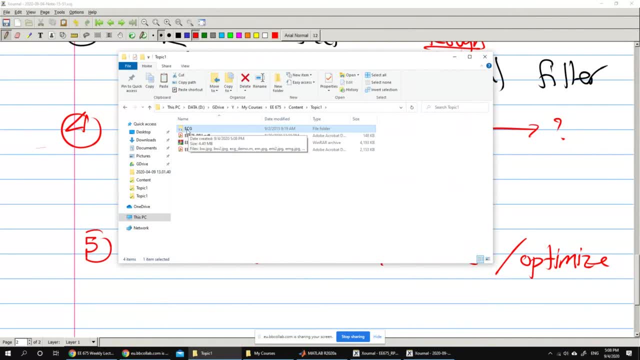 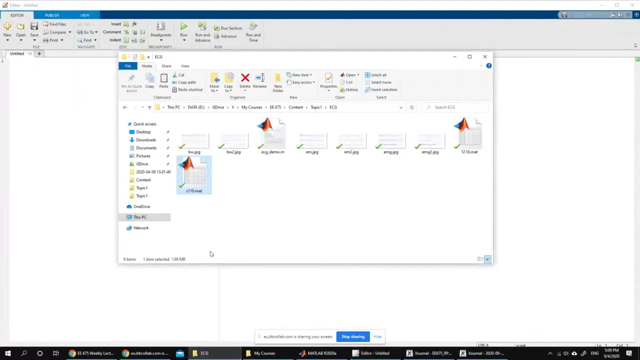 repeat exactly what i did and try to work a little bit more so that you can understand what what we had, and also generate questions, if you have questions. okay, so it has, uh, several images. i don't know if you kept all the funded sources that will see you. um, i can answer them, okay. 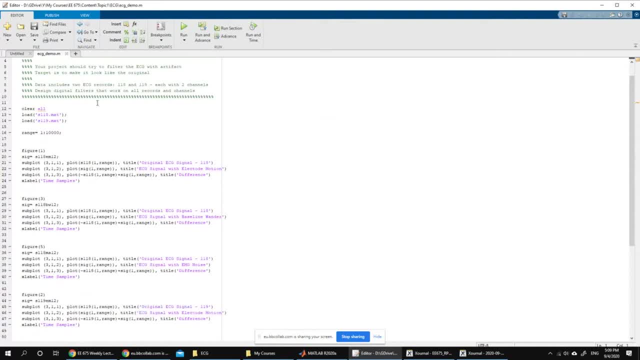 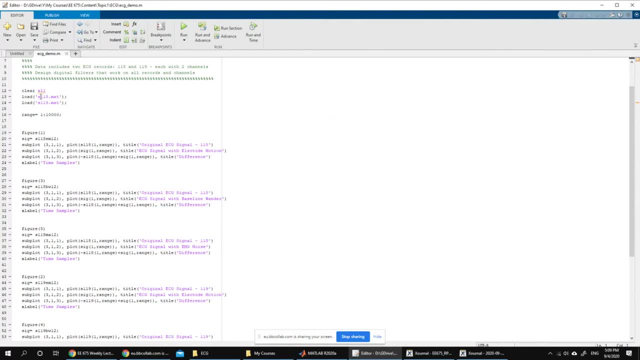 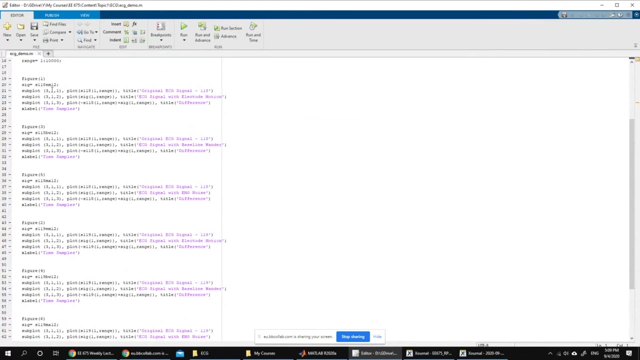 thank you, okay, thank you very much. okay, S118.mat and S119.mat- Load. basically, what it does is just basically loads whatever is in these data files and put them in the workspace, the MATLAB workspace, And then all that happens after that is just basically drawing the signals- different signals that are present in the MATLAB. 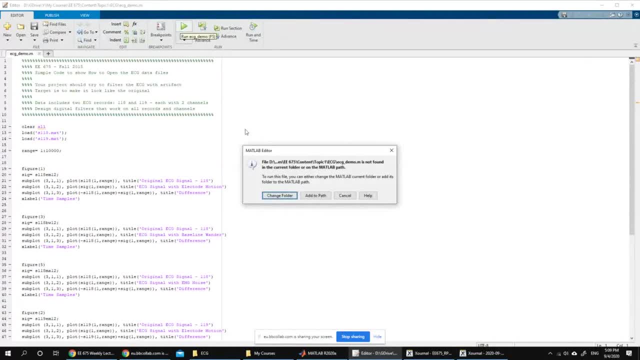 files. Let's just run it first: Change folder. You have to do that because basically, if you don't change the folder, then when it tries to load the data files it's not going to find them. So when you change the folder to where everything is, the data files will be exactly in the same folder as. 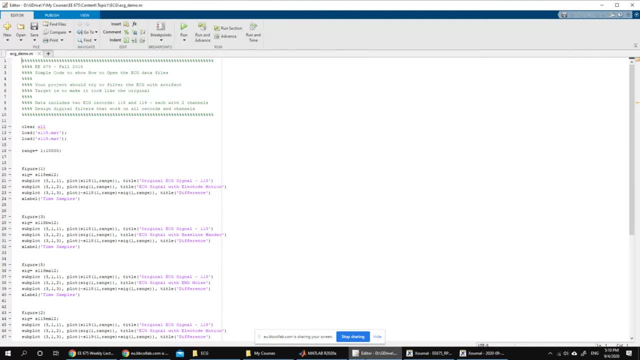 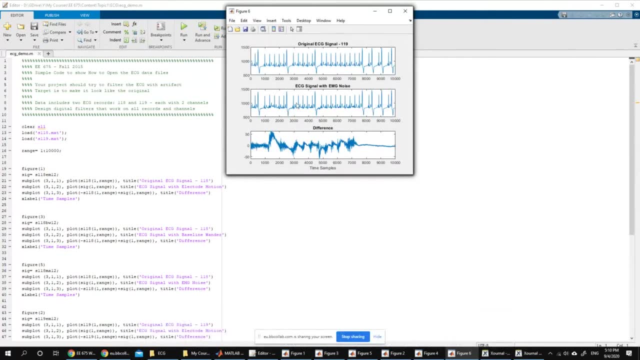 the code. So I changed the folder. So basically it's going to draw the different signals. So basically, here you have. for each one of these you have six figures. For each one of these figures you have basically the original signal, the signal with the EMG noise, for example, and the difference. 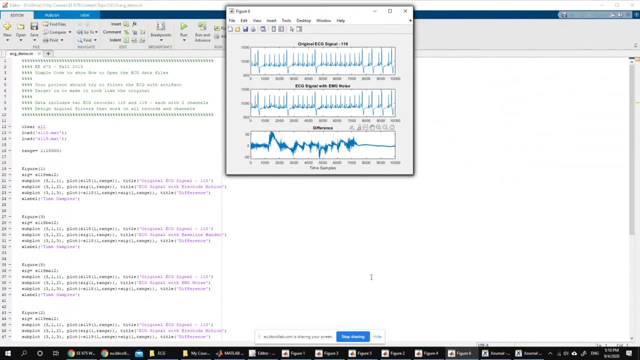 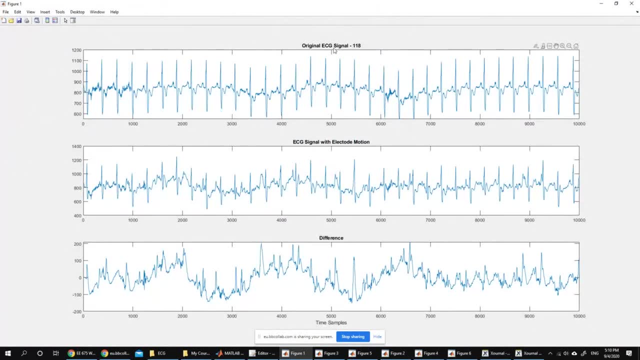 The difference between these two so that you know how the artifact would look like. Let's go for figure one. first, Magnified See here: this is the original ECG signal. So basically, this is. you see, you can see actually for for electrode motion. you basically see here: 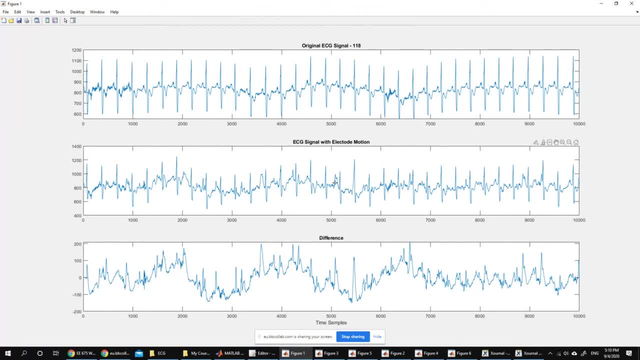 some variation, but actually with electrode motion it's much. basically, sometimes you see things that are not present in the original ECC signal. so basically, look at the difference. basically it looks really bad. okay, so basically this is the original, this is the one with the noise and this is the. 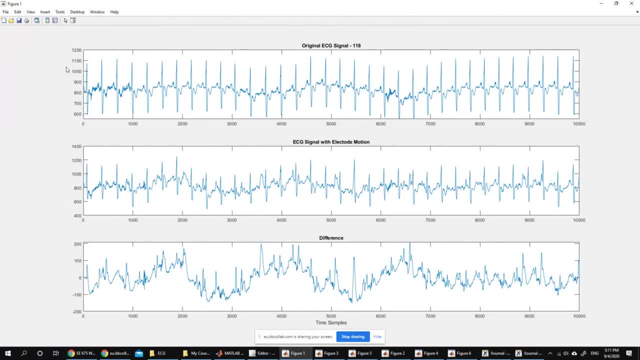 difference. please note the magnitude for each, by the way, so that you don't get confused. so basically, this is not as large as the ECG signals. basically, the small variations that you see here are the ones that are here, so you have noise levels from minus 200 to 200, while the signal itself is between, basically from: 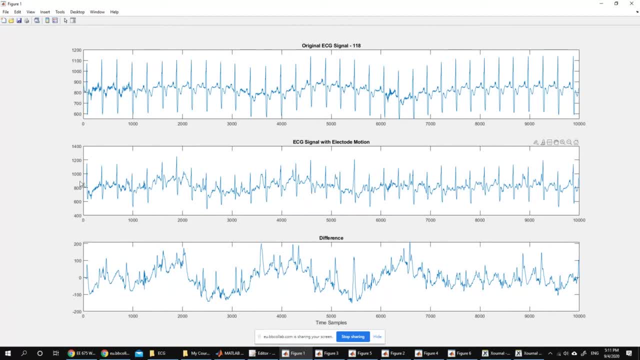 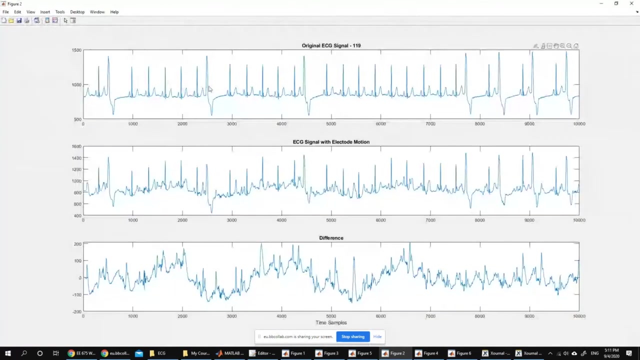 400 to basically, the peak to peak would be 1000. okay, so basically, just to put it in perspective, this is basically: you have two signals, two different signals. you have two signals, two different signals: signal 118 and signal 119. let's get signal two. okay, signal 119 is acquired. 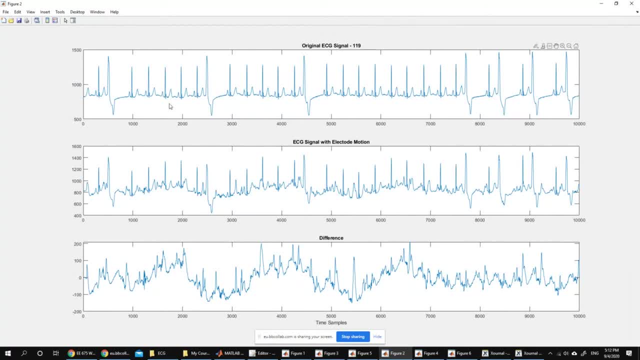 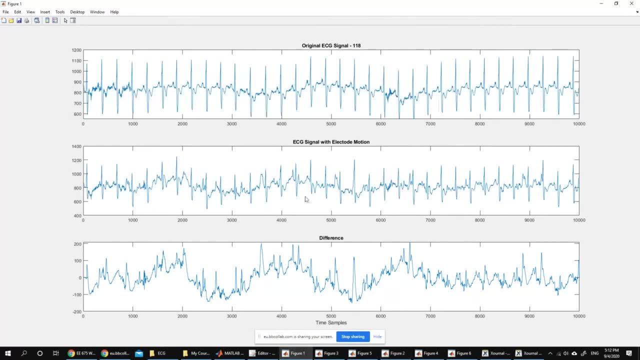 from a different place, so basically looks a little bit different. the ECG signals: they don't really look like ECG, the regular ECG that we know. that basically we saw here in the first one. this is: this: looks like the irregular ECG that we're used to. okay, but actually 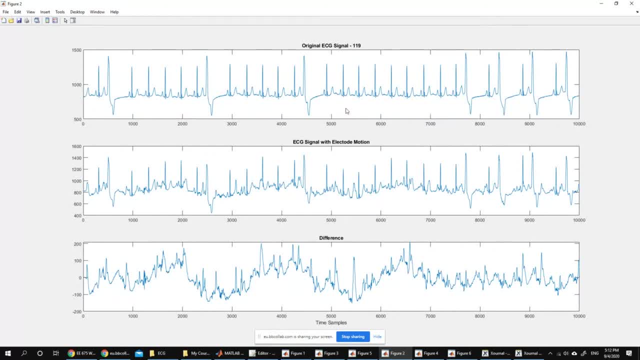 if you take the ECG signal from a different location, you will have a different ecg shape. so basically, this is like a different location, so that you know, or different patient- okay, so that you know how the artifact would look like from basically a different patient or from a different, from a different. 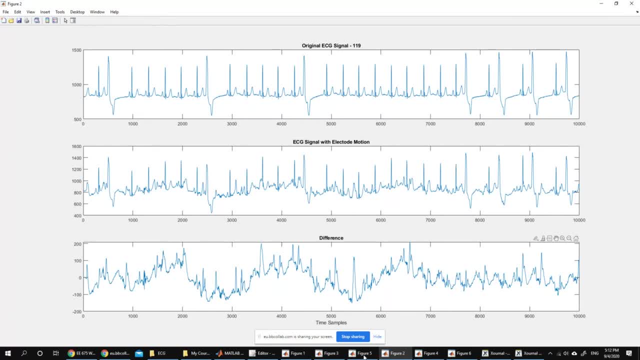 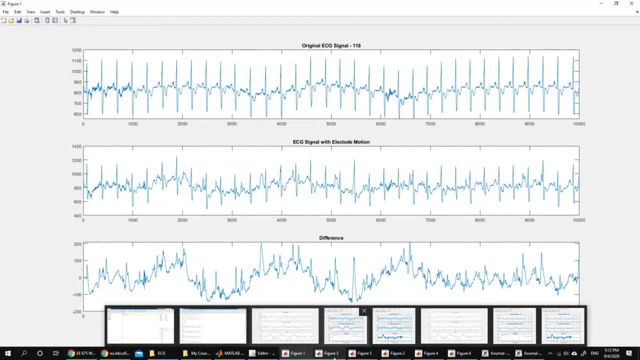 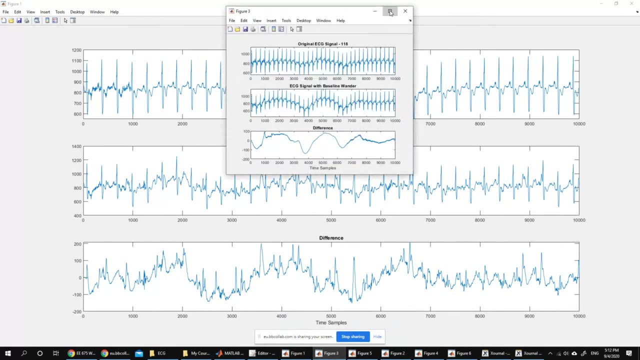 location because basically it's not gonna look the same if you look at this signal here and this other signal here might not look. look exactly the same. so this is a basic electron motion and it looks really difficult if you look at this one here. this is the one that we're going to start. 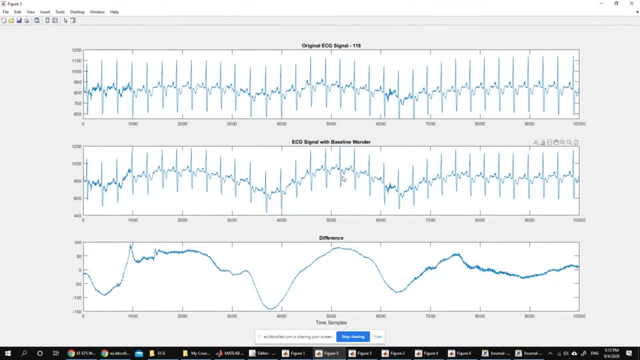 to start with, which basically contains the baseline lambda. so basically, as you see here, the signal basically is the ecg signal- seems to overlap a certain baseline shape. you have a shape that looks like this, basically, and basically your ecg signal is added to that, which is not good. this is the original signal, as you see. it has some variations, but they are. 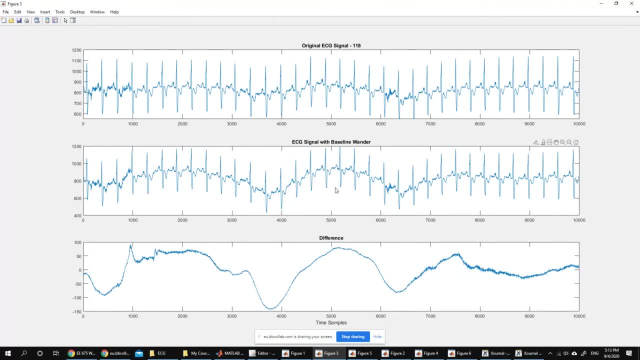 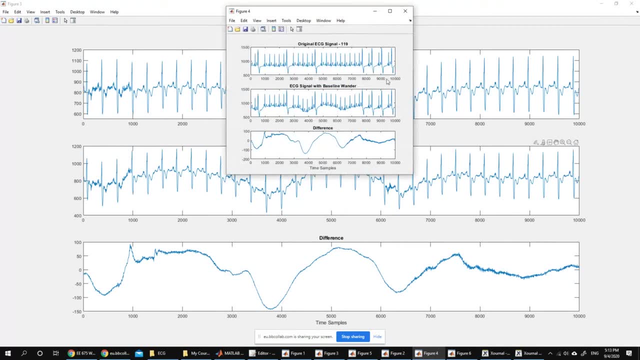 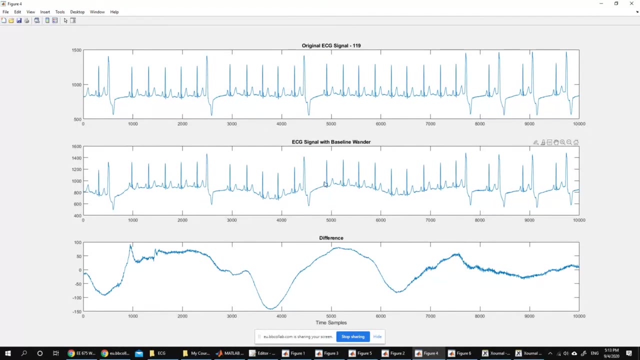 acceptable here. it's not accepted, okay. so basically you should try to get it at least to be like this, okay, if you look at the one from signal 119, it looks like this, okay, so basically it's very obvious that basically it changes things in the ecg signals. 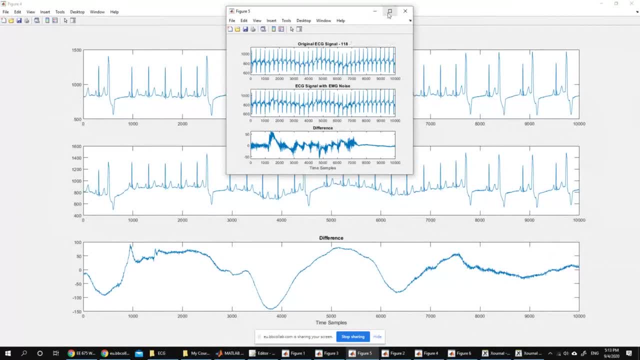 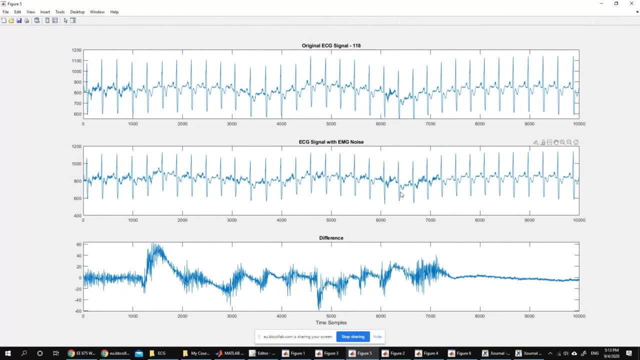 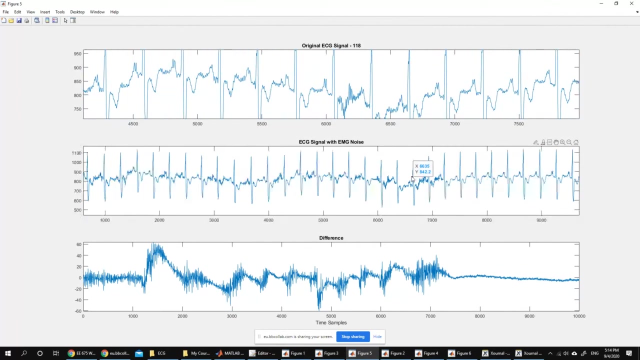 for the third artifact, which is the muscle artifact, looks like this. so, basically, if you look at, if you look at this, basically, in order for you to see that here, look at this one here looks clean, here it doesn't look clean. let me show it to you a little bit. let's just try to. 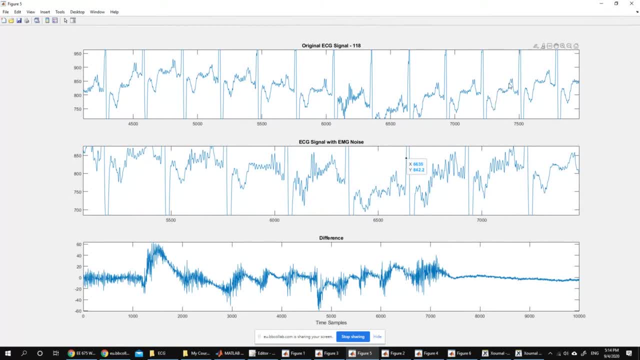 uh see, for example, here it looks much smoother than here. here it has very small variations. here the variations are much lower, okay, so basically this: this is very clear here, actually. okay. so basically, uh, emg is usually: uh, the range of emg signals is usually: uh, basically starts from the: 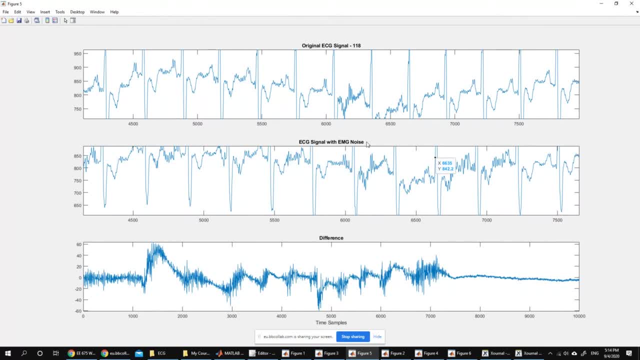 same frequency range of ecg and goes all the way almost one kilohertz or even more. it depends on the frequency range of the emg signal. so basically, if you look at this one here, it looks like a high frequency signal. so basically, if you take this part here, if you magnify it, 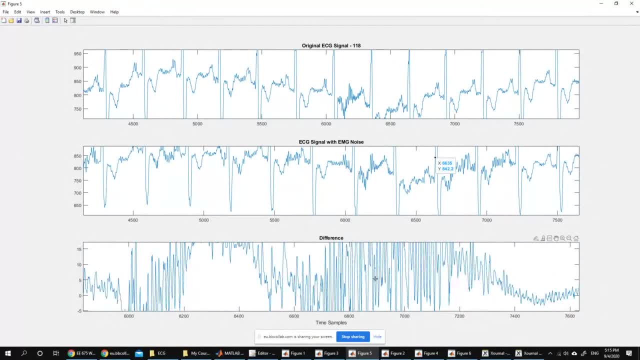 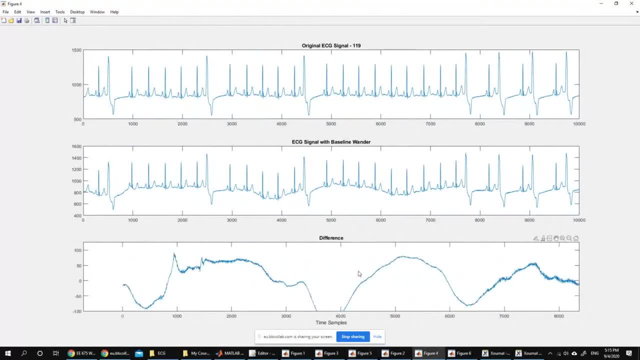 it varies very quickly. so basically this looks like a high frequency signal. if you look at something like, for example, this one here, magnify this actually no, so basically it has very small variations. basically, if you look at the, the, the signal signal itself, it varies, uh yeah, very widely. so basically it varies very slowly. okay, in this. 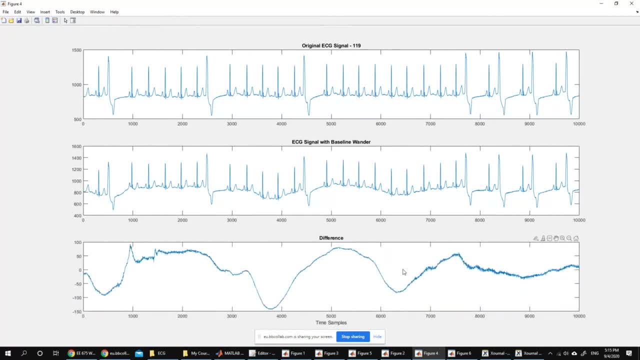 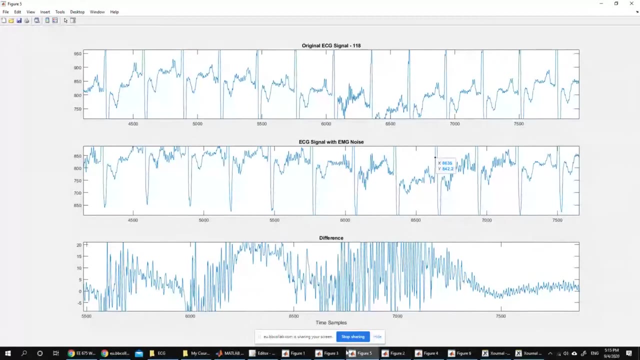 particular artifact. okay, so basically it's very clear that this is a low pass artifact. for the other one, the third one here, sorry, this one here this is a high frequency artifact- and for the other one. for the first one actually, it's complicated, it has both. basically, 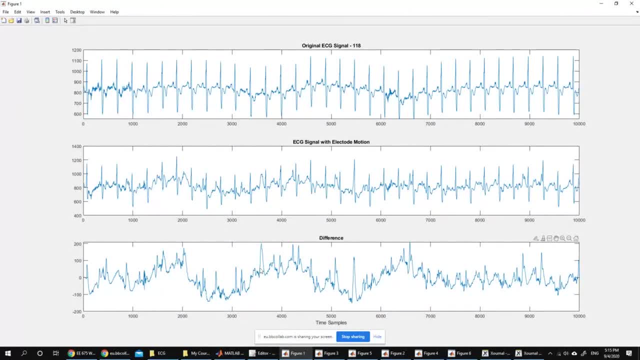 it's obvious that it has baseline variations and also has high frequency variations. so basically we can say that basically this has both. so, in order for us to basically think about that- basically we're going to talk about that in detail in probably next lecture- basically how to 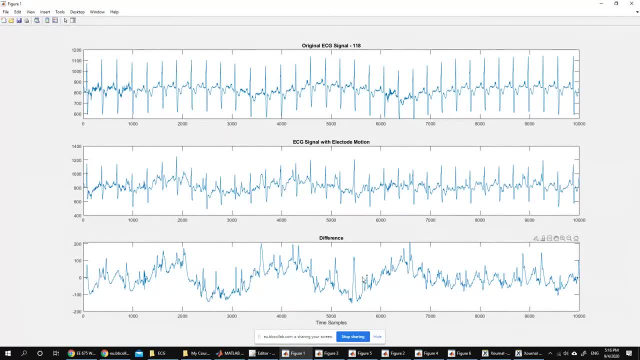 basically try to design a filter or estimate the filter specifications that would allow us to remove each one of these different types. okay, okay, if you could turn off your microphone. is that clear? yes, okay, okay. so basically, what we are going to do now is get started on the design of digital filters. 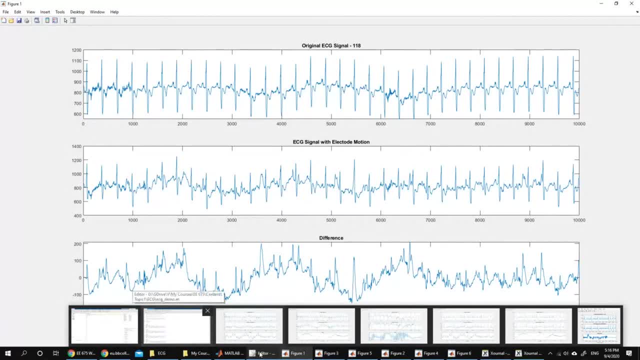 okay, uh, um, you never had any experience with digital filters in your signal systems course. You ever had any experience. none of you had a signal assistance course. Okay, so I assume that none of you had any digital filter design experience? is that correct? 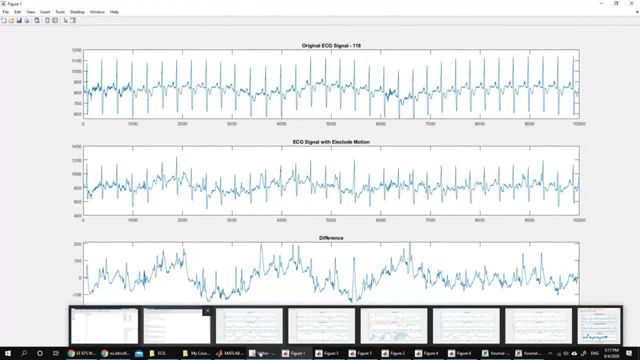 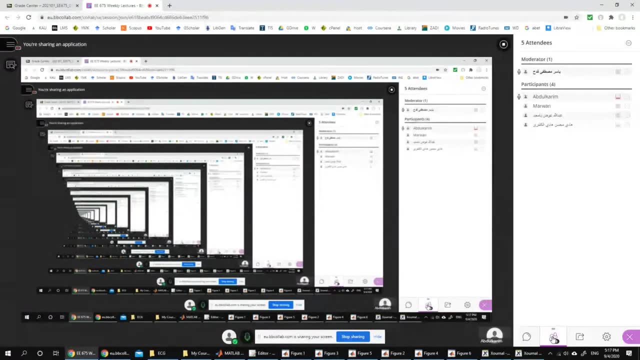 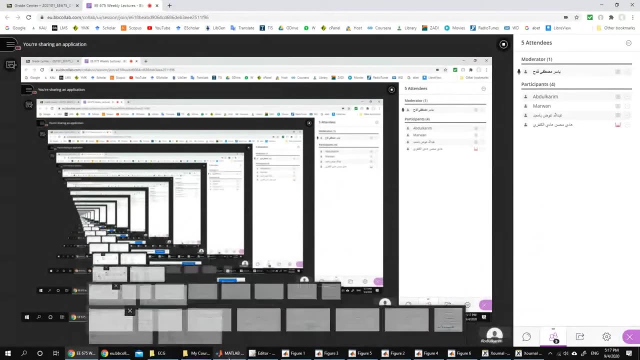 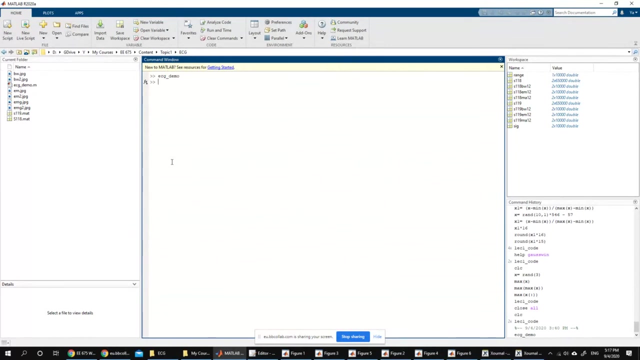 Yes, Okay. So I don't see Reno still. I was hoping that Reno would be here by that time so that we can get started on the digital filter design with him. but it's fine, it's fine. So, basically, what I'm going to do now is get started on the part where we use MATLAB to 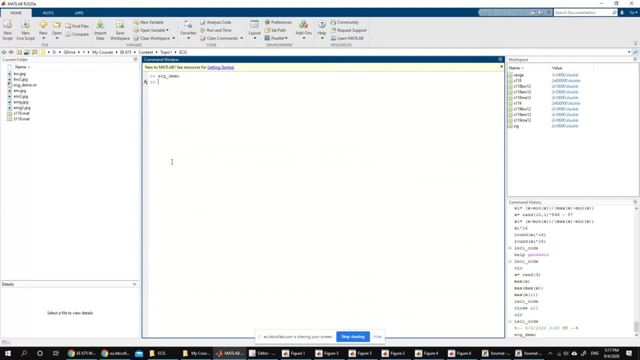 design digital filters. okay, So basically MATLAB has a unique tool for designing filters. basically it's called filter designer. It used to be called FBA tool, filter design and analysis tool. I think in the new version they call it filter designer. 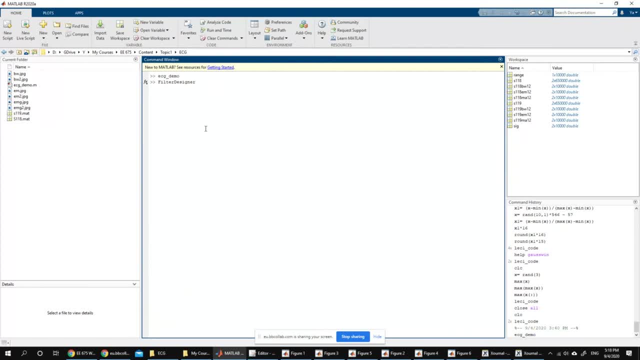 All of you have. does anyone? basically you all have MATLAB by now. right, Yes, You all have MATLAB, or not? Let's just share the lessons, The what It's easy to get it. I can hear you clearly. Lessons. 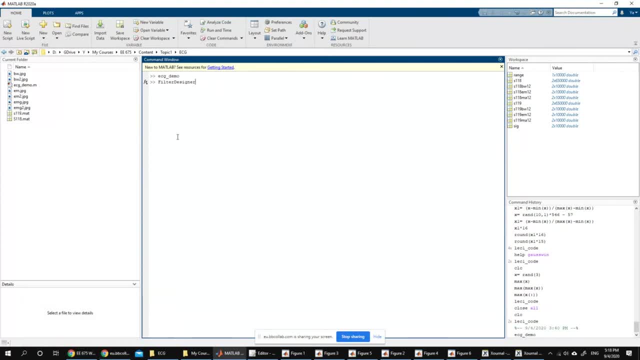 You still have the problem. From last time, I mentioned that if you have a problem with the license, it means that you don't have MATLAB. okay, So this is a problem, okay, Yeah, yeah, So you need to find the what. 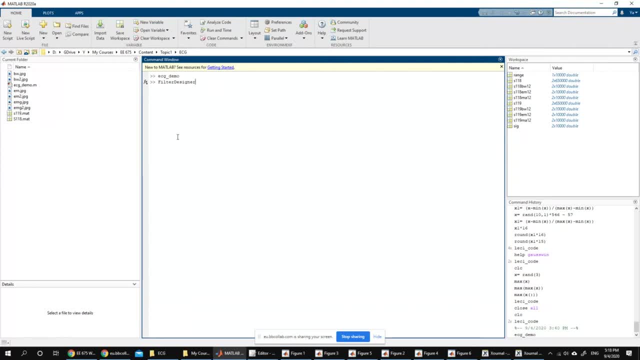 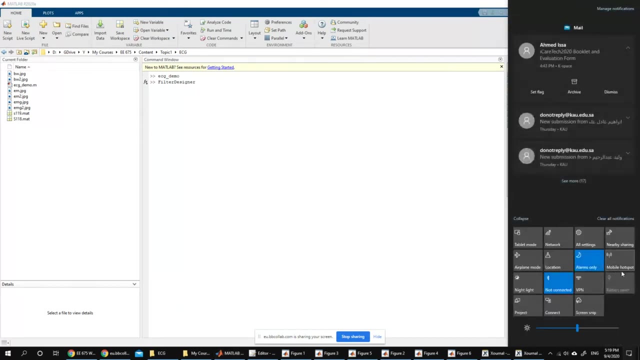 The what You have MATLAB. You have MATLAB. No, no, sir, We try to get it, but the problem with the license that mean we don't have. I'm not sure exactly what to tell you, but actually it's a big problem. 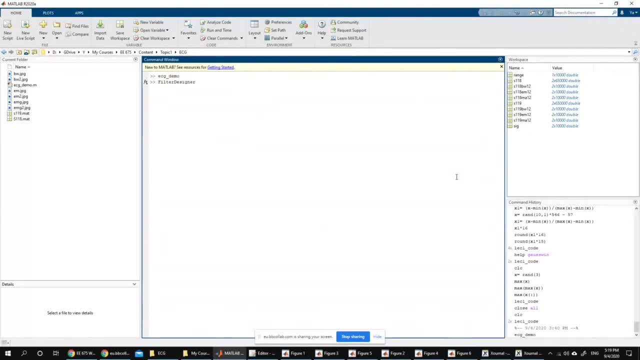 If you don't have the license, then you cannot work with MATLAB, right? so what can we do? I can't you get a copy from someone we won't be try to get you. you still not successful in doing that. I search for it's here in my area. I can't. 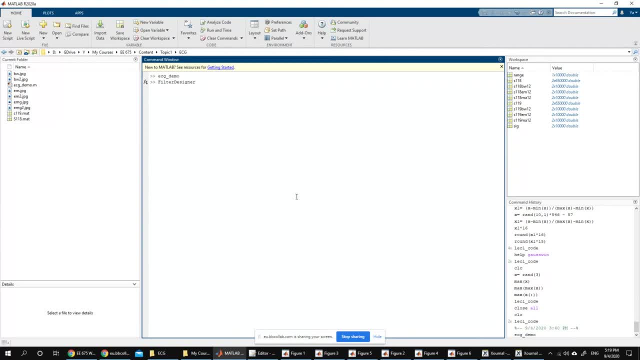 found it. I mean from other students. I'm not talking about going to a bookstore or something like that. you never gonna find in there. I mean from the other colleagues in the department on the program you've asked them. yeah, I should do a little bit. let me ask you a question. 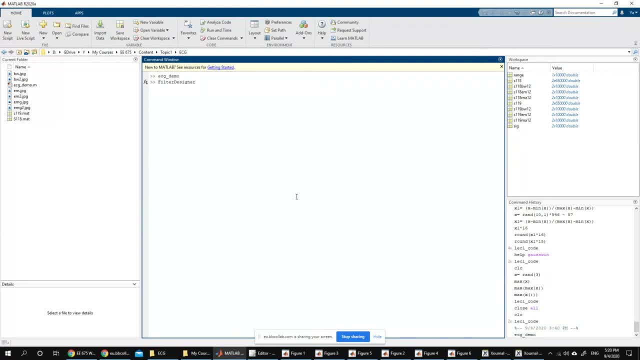 I have a copy of the 2013 version. 2013 will be a little bit old, but now Abdul Kareem will be 19 or 20. 13 will be old. not all of them will have it. that's what I'm worried about. 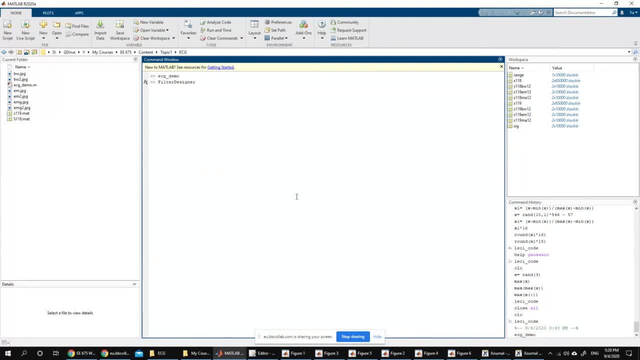 ok, ok, this is a major problem because actually I was hoping to get started on this now and you go home and or basically after the lecture, you repeat what, what I did. so I'm not really sure what to do. but I'm not really sure what to do, but let me get started with this. but 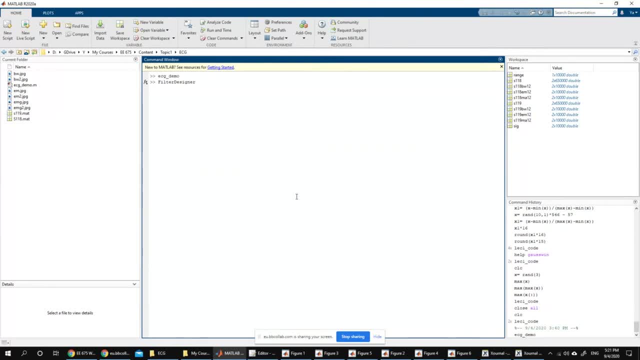 it's a big problem actually. yes, go ahead. yes, yes, what we're talking about is a cracked version. it's not a real version, not an official version, because basically we We have no way of obtaining an original license. I'm not sure about the student version. 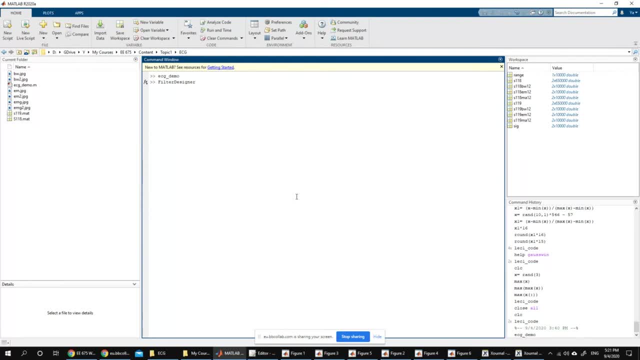 Some people said that you can get a student version of MATLAB for like twenty nine dollars, something like that. I'm not sure if you can get access to that. Reno was planning to do that. I'm not sure if he did or not. 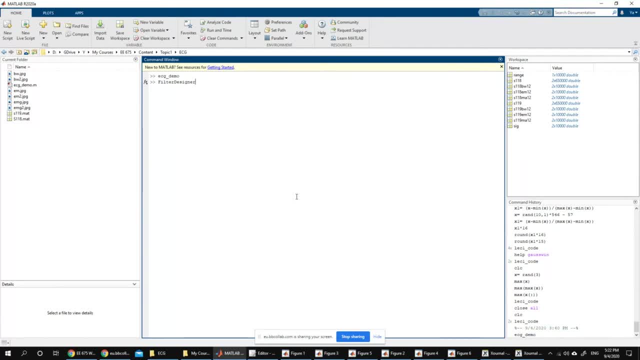 But you can ask him. The program is the same program with me. We exactly work on it last semester and the license of the same program. You know, I think I will be calling him if he gets that one by 20, by 30.. 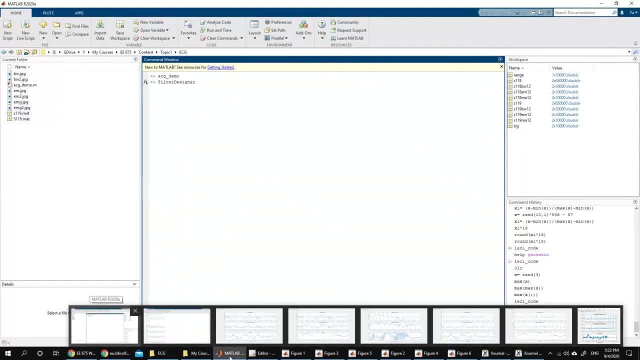 It's not matter, We can pay for it, OK, OK, OK, No, I mean, I mean the original version, the student licenses. This is very cheap. It's not not expensive. I tell you what. basically, I'm going to go over the MATLAB things. 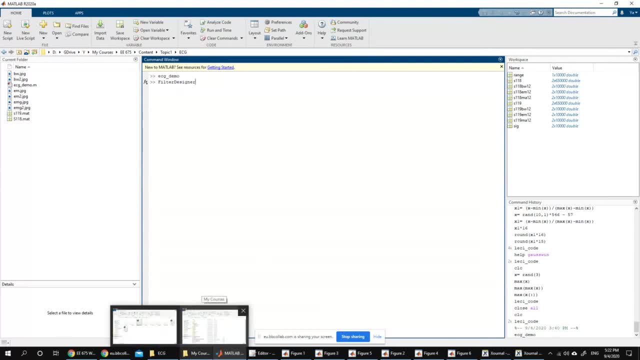 Maybe I can ask someone: can you, can you hold on for five minutes? I can call someone and check if he has a license or not. OK, can you hold on for one second? for five minutes? Just one minute? Yes, sure, I have a question. 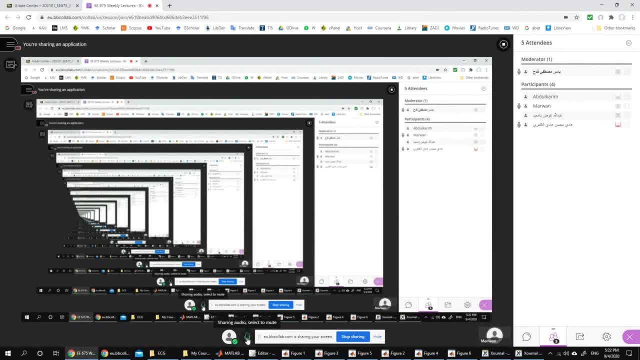 But the problem is it's About 20, 26 gigabytes. I don't know how to pass a copy to my my friends, So you have a copy of 26.. OK, It's very difficult to upload. You have to get it in person. 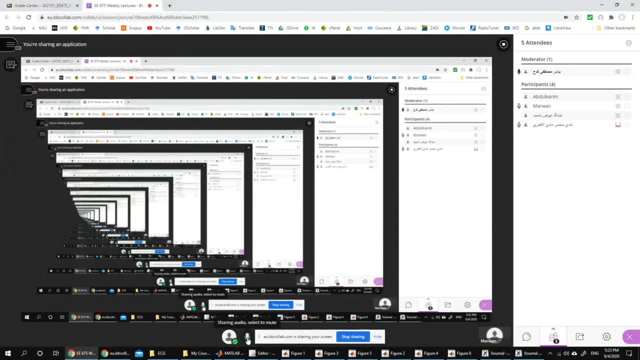 OK, let me. let me try, because actually I know of a version that's a little bit smaller than that And maybe we can actually post it somewhere. Just give me one minute, I'll call someone and get back to you. OK, just just hold on, OK. 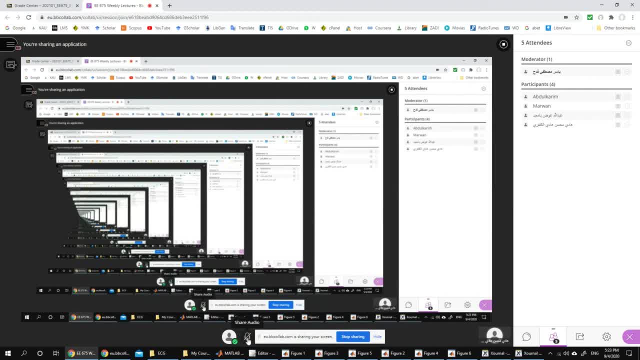 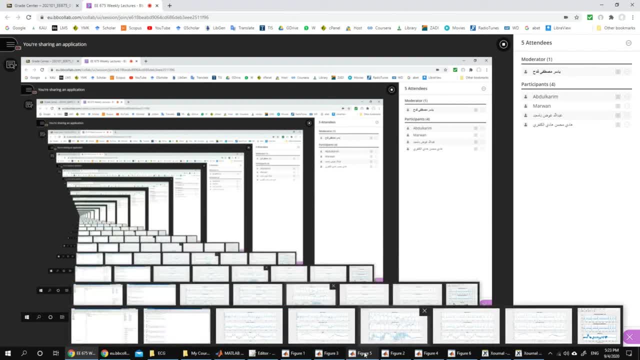 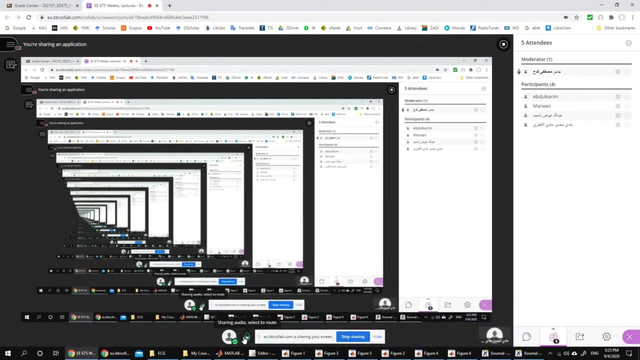 OK, OK, you, you, you, okay. I think we can get the 2017 version, for it's about 11 gigabytes, a little bit smaller than that. 26 gigabytes for the later version. okay, so 20 and 2017 should be okay, okay. so, basically, I'm gonna try to get that copy, that 2017 and basically. 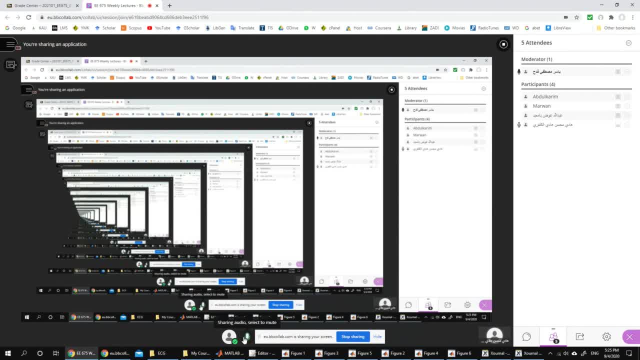 upload it somewhere and send you the link to download, and I'll remove it quickly after that if it doesn't work. maybe 11 gigabytes should fit within the Google Drive size, so basically it shouldn't be a problem for the 26. I think it's above the Google Google Drive limit, so 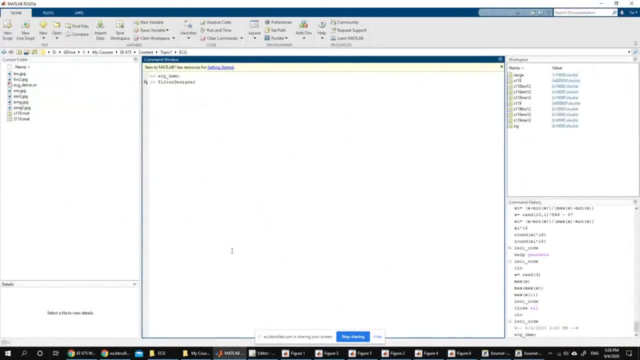 basically, hopefully this will solve the problem, okay. so basically, hopefully I'm gonna do that today, inshallah. okay, I'll send you the link and basically let me know if you have any problems. usually the link is in the, at least the one that I discussed with person. 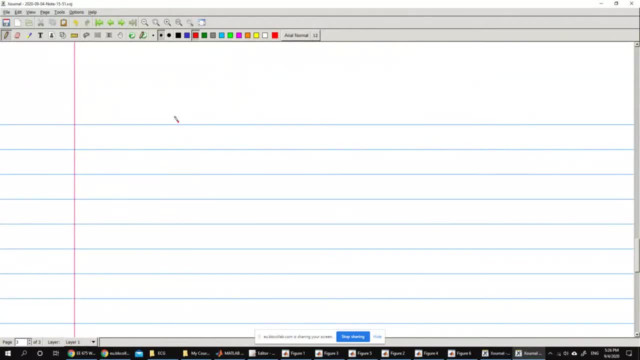 basically it comes dot ISO, it comes as dot ISO file. okay, dot ISO opens with WinRAR just like any archive. okay, so basically it has to two sides to. I basically is what you, what you make to basically burn on dvd, okay, so basically iso is the if you. 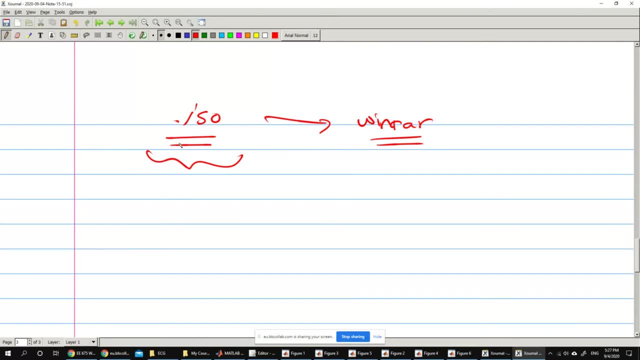 have a dvd, so basically you can actually put it in the form of iso and basically. so you have dvd1 and you have another one for dvd2. so what you would do usually is basically start with this one and you will have the installer there, okay, and then, when the installing program asks you for uh, inserts. 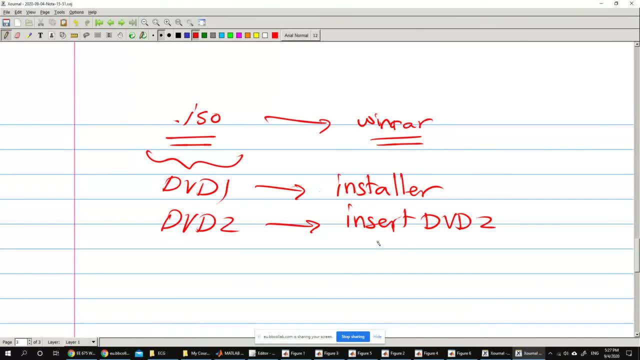 uh dvd2. you basically uh unzip this file, okay, or uncompress this file in exactly the same location as dvd1, okay, if you have any problem, basically look at the. there will be like a, a location where you see or an explanation on how to uh basically install that version on that same dvd1. 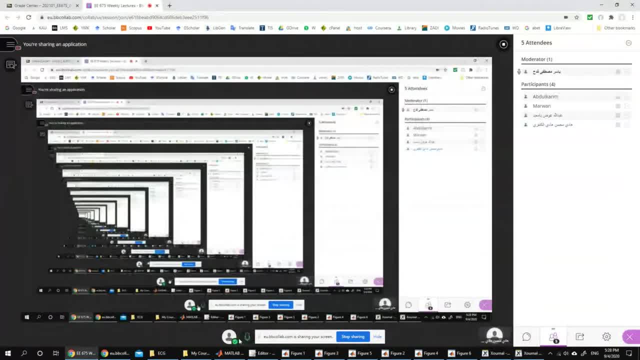 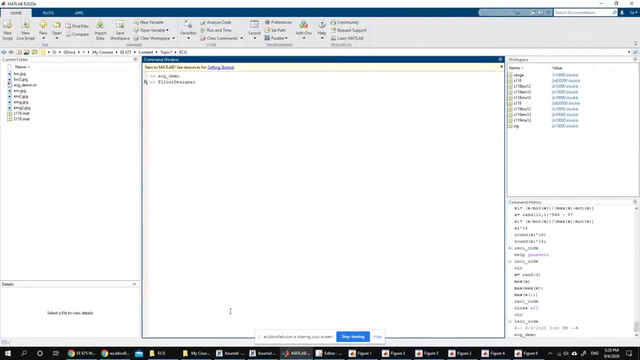 that clear? is that clear? yes, okay, yeah, okay. so now we're going to get started on, uh, the filter design and the simulation and then, hopefully, uh, by the time you uh basically get started on these experiments, by the maybe tomorrow or something like that, you'll be able to have the matlab and basically get started on repeating what i have here in the. 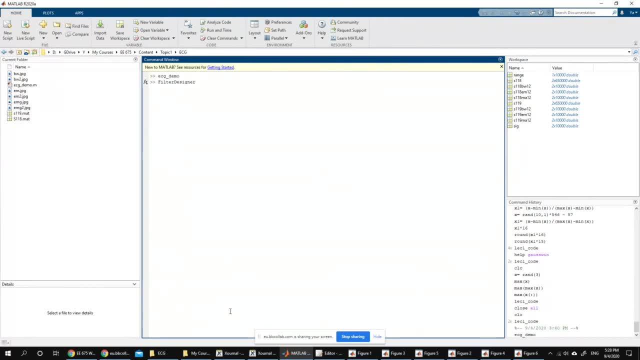 lecture, okay. so even if you have the matlab after two, three days, it's gonna be still okay. you can look at the video of the lecture and basically follow up on that later on, and i hope that was what i have there, okay, so i'm going to start with filter designer. sorry, filter designer. okay, filter. 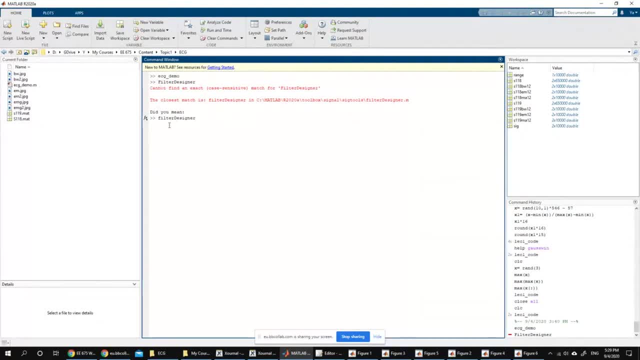 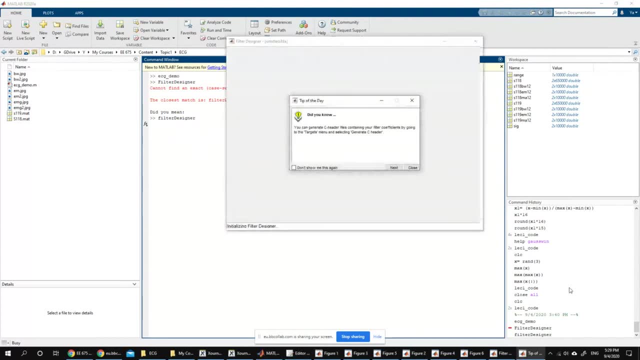 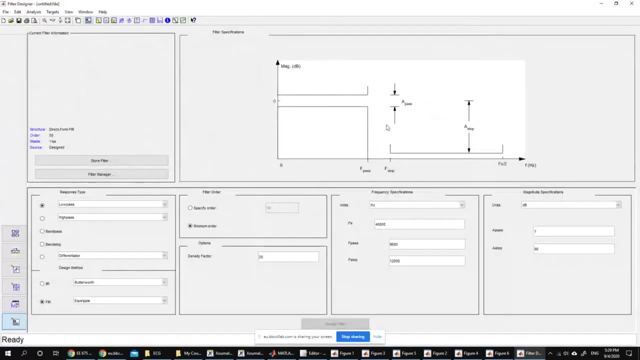 filter f: small. okay, you notice that. filter designer: filter f: small. okay, so filter designer: okay. close. you have an interface that would look like this: basically, the filter has certain characteristics. any filter okay, for a low-pass filter, for example. we're going to start with a low-pass filter. basically, whenever you select the filter type here, this is low pass, this is high. 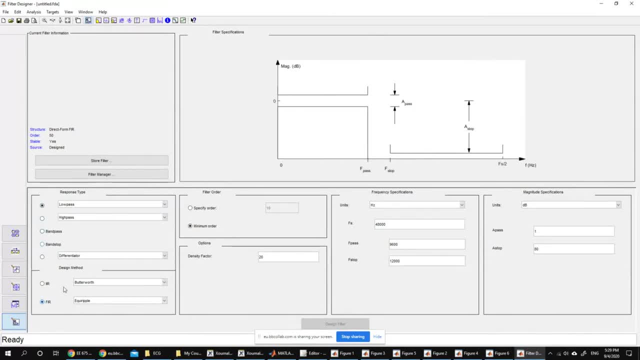 pass. this is band pass, this is band stop. and basically we have two different types of filters: fir and ir. what i'm going to do now is i'm going to show you a demonstration of how to design a filter and how to apply it to a simulated signal without getting 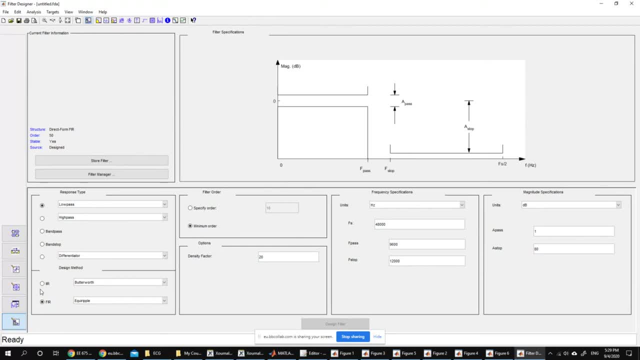 into the theory at all. okay, and basically, when we feel comfortable designing the filters without even knowing the theory behind it, i'm going to explain the theory and then you will feel that basically you will, you will know the theory much better when you actually try things and 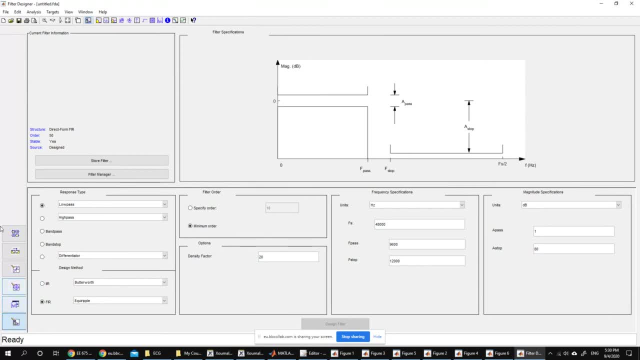 know how the outcome would look like. so in order for you to design a low-pass filter, you have to design- basically, you have to have a certain uh cutoff frequency, which is called fs, unlike the ideal filter that we talked about uh in the um. let me just uh. 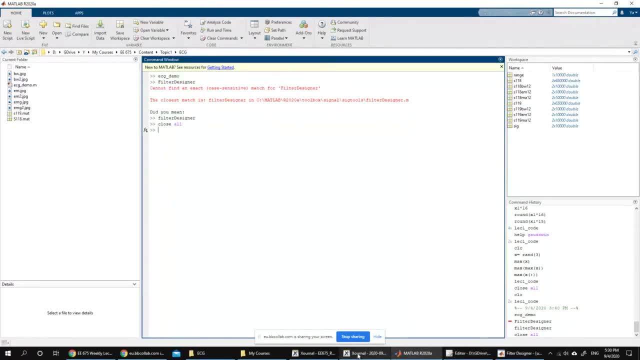 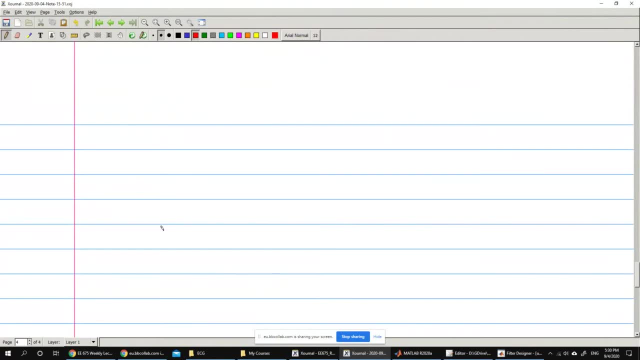 close all the um. basically, uh, unlike the part um or this, the, the design that we uh talked about in the theoretical uh context, like: basically, we assume that the low pass filter looks like this: okay, what you call brake wall filter, brick wall, like a, like a wall. basically you have. 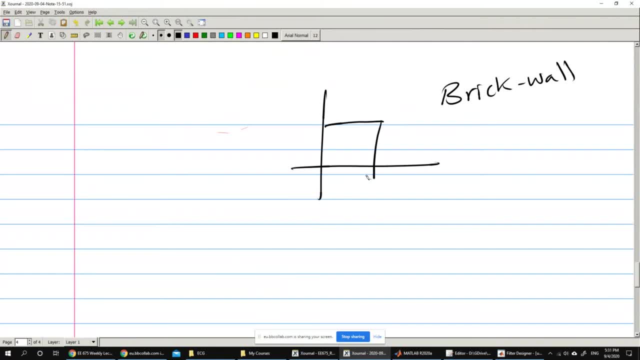 a filter that, uh, basically you have. if you have a frequency here, it would pass here. it passes here, it doesn't immediate after. so if you have a cut-off frequency of 10 Hz, then 9.9999979, 7.999999999999999999999999999999 tells you. the low pass filter looks like this: 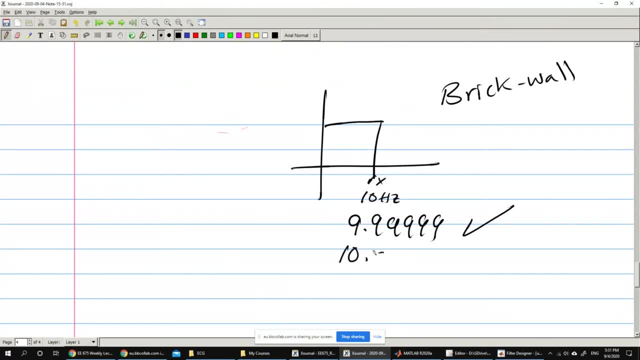 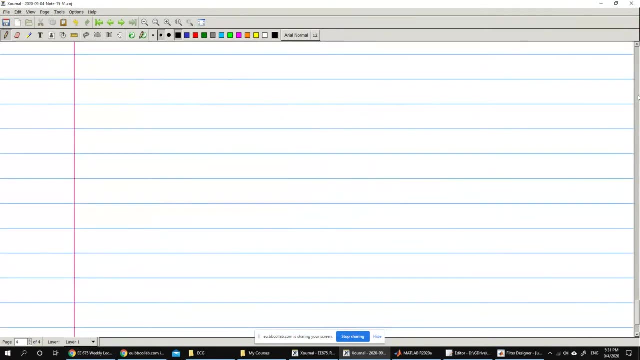 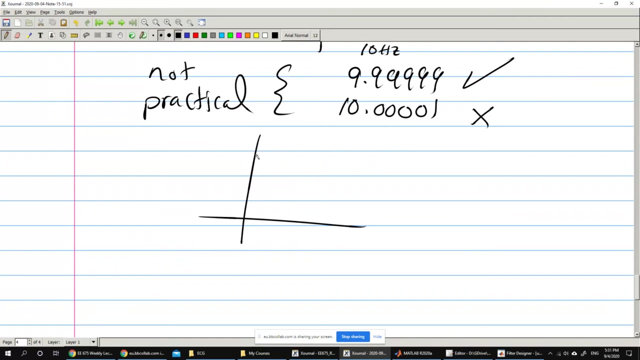 999 would be okay, 10.00001 would not be okay. Okay, This is not practical, Okay, Practical filters basically look a little bit different. Basically, they have a smoother transition from the pass band to the stop band. Stop band basically, where, basically, you remove. 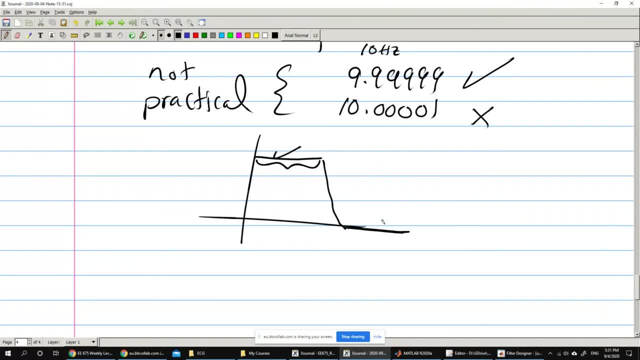 the signal Here, the pass band where the signal passes Here, the signal doesn't pass Here. basically, in the middle between the two, what we call transition region. Okay, Basically, it starts from what we call f pass here. We call this f stop, Okay, Basically. 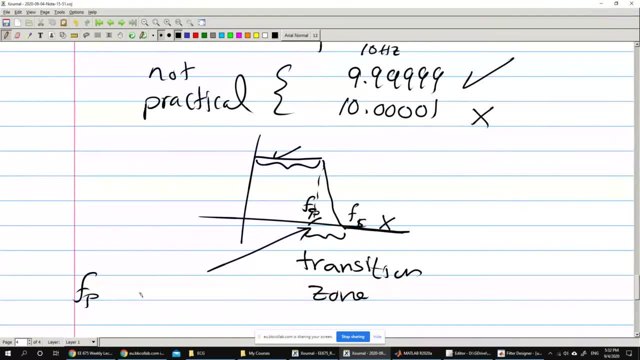 f pass. the first frequency is the limit of passing, The f stop is the start of stop And the transition zone here ideally will be zero. but it's never zero. In practical filters it's never zero, And I'm going to show you the effect of. 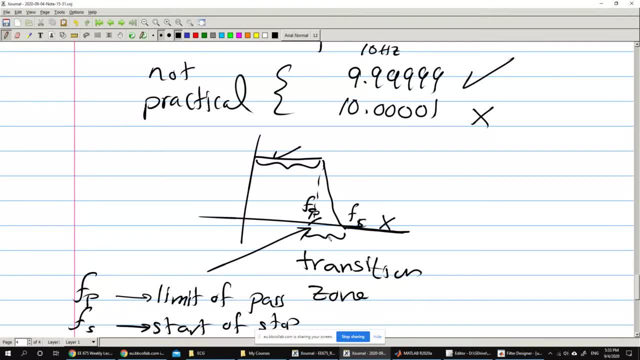 designing the filters to have almost zero transition zone. The second thing about the practical filter is that usually in the pass band the f stop is the start of stop And the transition zone here ideally will be zero. And it's never flat like this, It's never like one, It's never like this. It can actually. 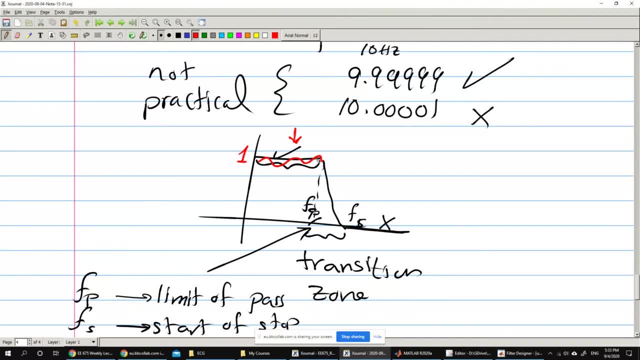 have some variations around one And basically, instead of having just one here, you allow it to change here within a certain limit. Okay, So you have. you allow certain range that is acceptable for the variations. For example, I can say that it's one plus minus 0.1, 0.01, to be. 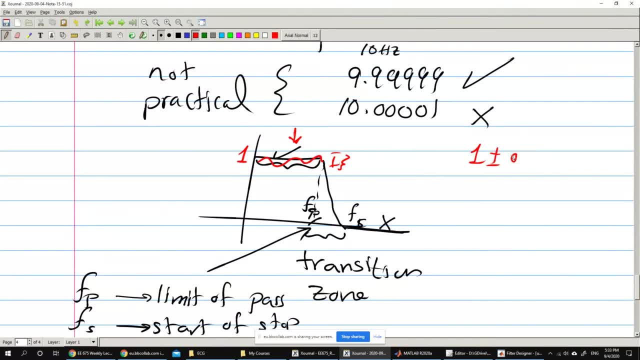 okay, we actually better, okay. so basically it's 0.01. okay, i'm accepting a tolerance in this one for the stop band. you actually need to define what's called minimum attenuation. so basically, uh, you have to have a, like, a certain level of depression or a certain level of suppression. 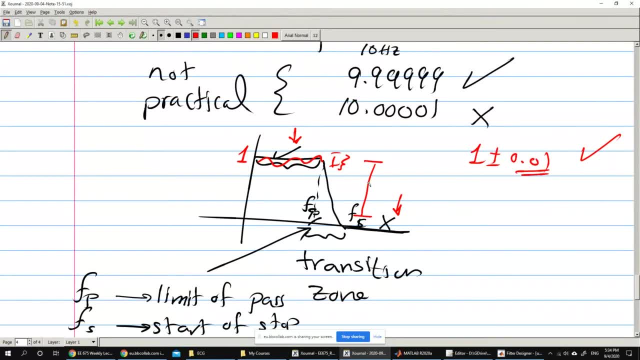 of the signals in this band. so basically, uh, i can say that all the signals in the stop band must be multiplied by at least 1 over 100 or 1 over 1000, okay. it means that if you have a signal, if you have noise, okay, in this range it would be multiplied by at least 1 over 1000, or at least. 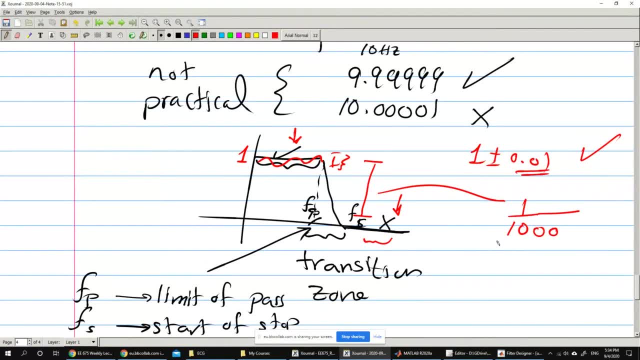 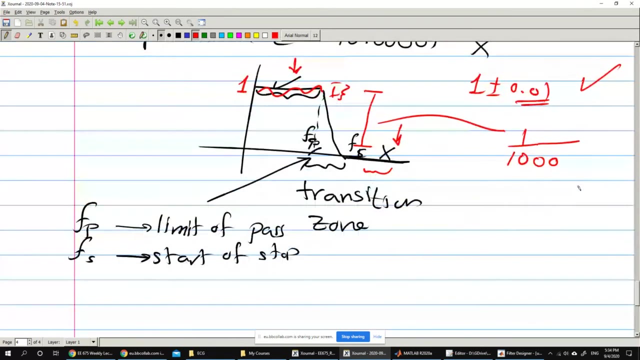 1 over 100. okay, so basically, in order for me to design a filter, uh, i have to have basically the f-pass, f-stop attenuation or the pass band tolerance and the stop band attenuation. okay, let's go and look at the filter design tool and basically apply that practically. 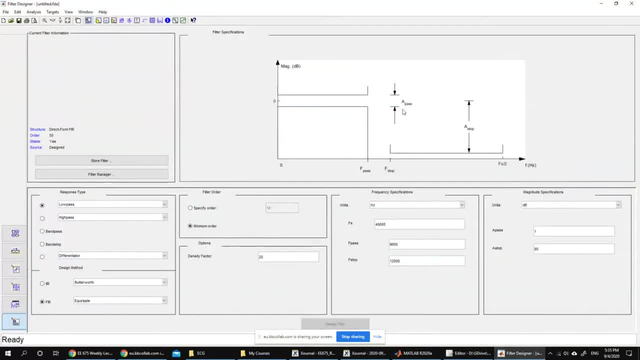 this is the filter design tool, filter designer. basically: here the tolerance of the pass band, here the attenuation of the stop band, here f-pass, here f-stop. let's assume that we're going to repeat example, just the example that we're talking about. we have two signals. one of them is 10 hertz, the 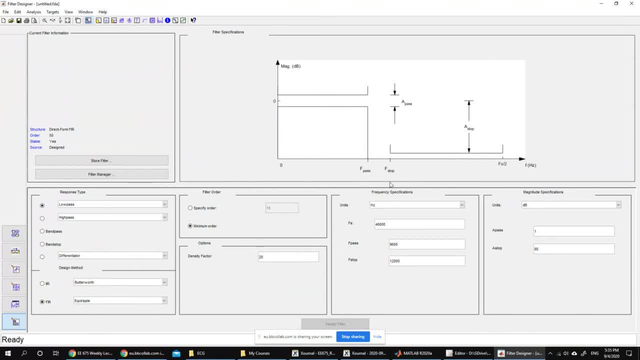 other one is um 30 hertz. i would like to separate these two signals, so i would like to design a filter with a cutoff frequency or a pass band frequency of 20.. so basically i'm going to start. first of all, you have to have a sampling frequency, otherwise it's not going to be. 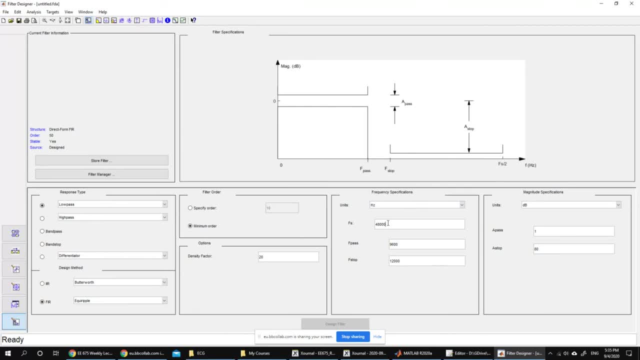 able to do anything. so, basically, let's assume that we have a sampling frequency of um, for example, uh 200 or 300, whatever 200, 200 uh samples per second, the f-pass- here i'm going to say that there will be 20.. okay, the f-stop. f-stop means that 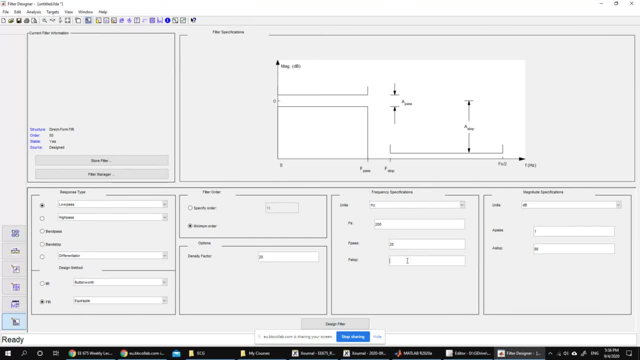 this is the level basically, at which, or beyond which, the attenuation that we are going to define will apply to all the input signals. so basically, i'm going to say, for example, um 25.. basically, after 25, including the 30 hertz that i'm going to want to filter, okay. 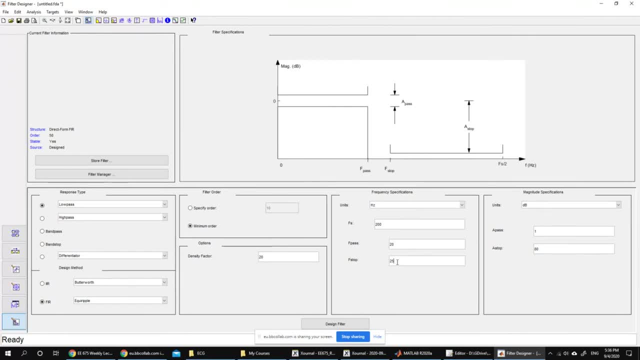 basically will be: basically will start at 25.. here i define the best band attenuation and best band the tolerance and the stopband at the affiliation. usually people in the filter filter community, filter, a digital filter community. they are used to decibels. so, for example, when we 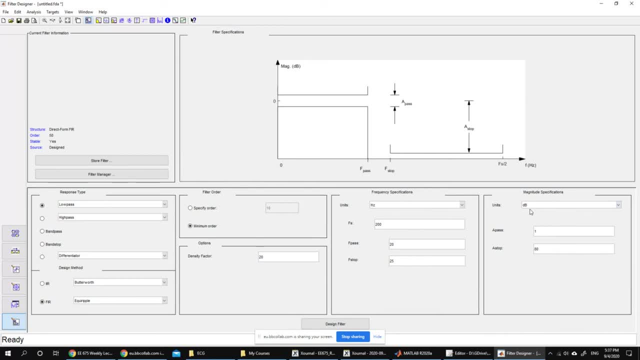 talk about the cutoff frequency, we say that it's a 3 db point, three decibels. okay, so basic decibels, but actually, if you want to have it in linear range, you can actually put it like this. so basically it's here, it's 0.1, which means that the signal would be 1 plus minus 0.1. 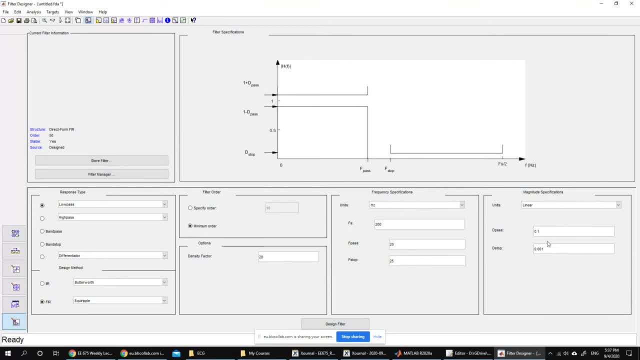 if you want to have it 0.01, you can have it 0.01. here the the stop band attenuation is basically 0.001, meaning that any signal with frequency in the stop band will be multiplied by at least 0.001. so 1 over 1000, okay. 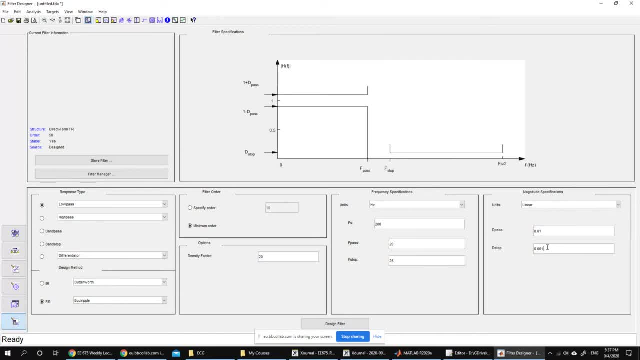 let's try to see what the filters, what this filter would look like, and basically then try to think about basically that, the different parameters here- and basically try to see if you understand what you're doing or not. so basically all i have to do is just come here and say design filters. 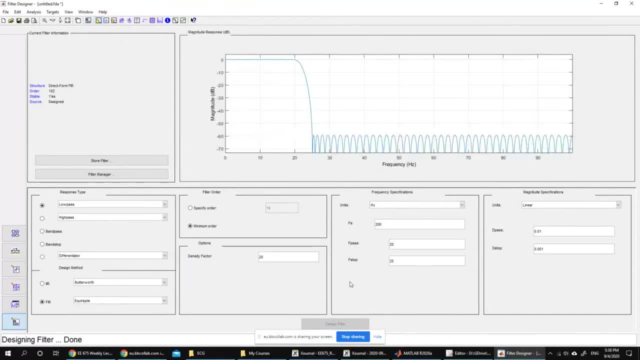 it looks like this is basically the characteristics of the filter. basically, you see here some very small variations. you see here variation, but actually all of them. basically, the magnitude here is decibel, decibel. if you have, uh, one over one thousand, it's minus 60 decibels. so here you. 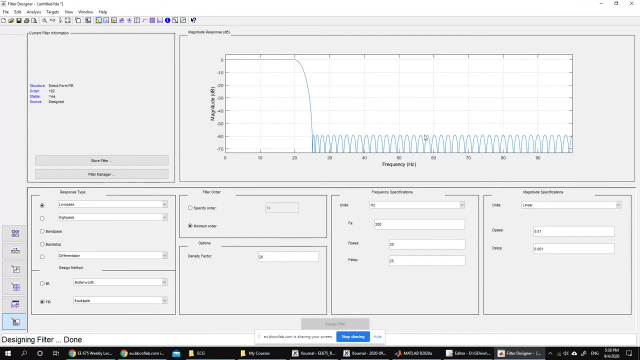 see that all the the parts in the uh stop band will actually be below uh 60 or minus 60 decibels. so if you have a filter that's below 60 decibels, you see that all the the parts in the uh stop band. 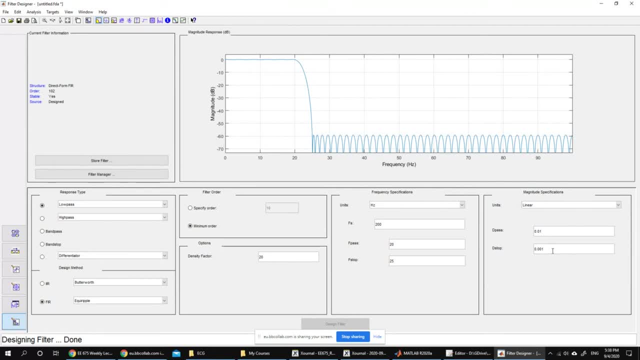 60 decibels, which basically satisfies this okay. so basically this looks like a good filter. basically you start with 20. here this is a cutoff frequency, 20 looks okay and 30 or 25, basically you start the stop band. so basically at 30 you're sure that we give you apply by at least 1 over 1000. 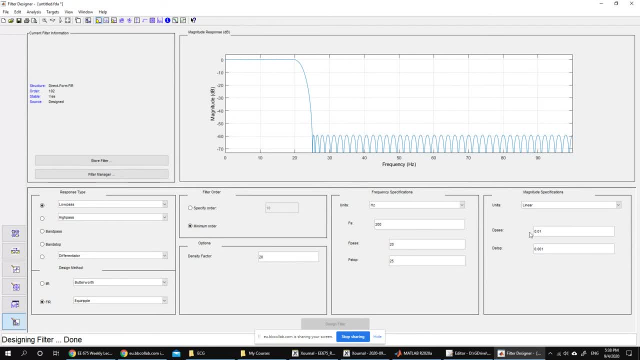 are these specifications the best we can do? actually? uh, no, because basically, the order here. if you look at this part here, can you read the text? can you read the text please? well, this one is basically the size of the filter, basically, and just give you an idea. 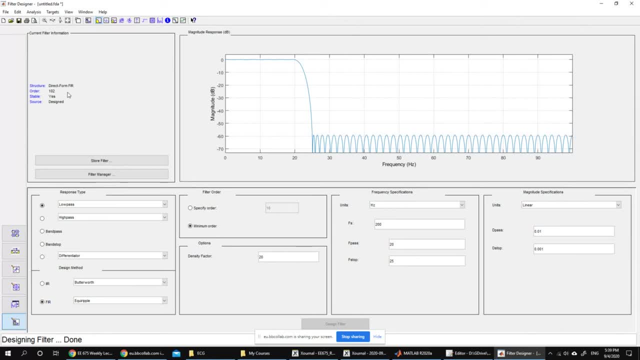 uh, if you're assembling a digital, if you're assembling an analog filter in the lab, if you have an rc filter- remember the rc filter- you have a resistance and capacitor. this is basically low pass filters. okay, the rc filter is an order, one filter in order for you to have. 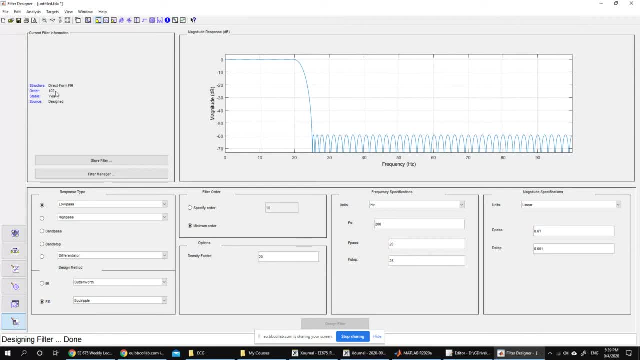 an order 102, 102. you have to have 102 resistors and capacitors and imagine that. okay, so this is a little bit large. so basically, uh, we're talking about a filter that would be implemented in the computer. so some people might might think that we don't really care, okay, but actually we're going to see. 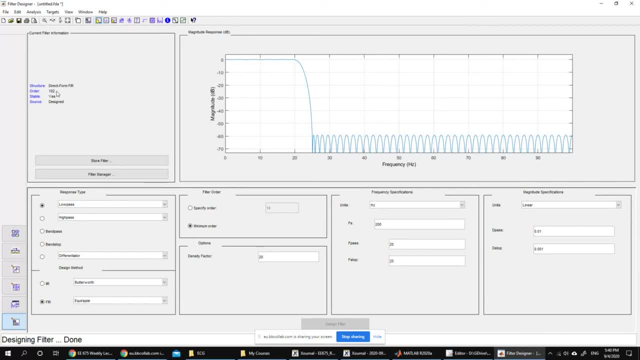 that this order will have some, basically some consequences and usually, in order for you to implement a filter with an order 102, you're gonna you're gonna have to do more calculations than a much smaller filter and basically, if you want to implement that filter to be a real-time filter that is basically working. 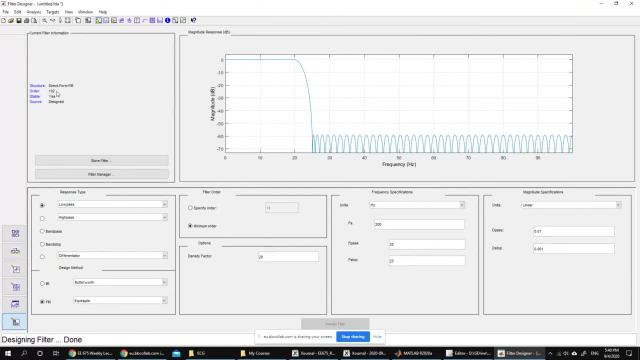 in real time. so as the signal is coming to the computer, you're basically processing and displaying in real time, then this would be a problem. okay, let's try to see the effect of each one of these parameters. so, for example, let's see, for example, if we make the f stop very close to f pass. so 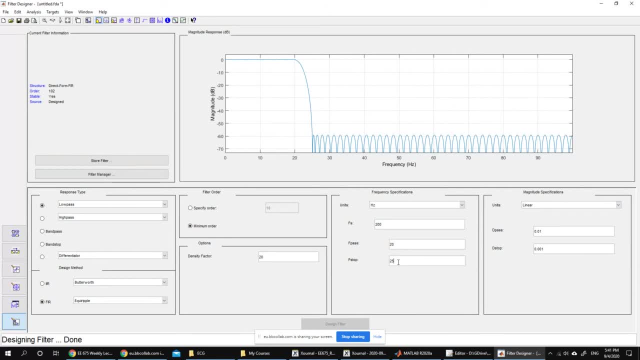 basically, we're trying to make the filter as ideal, as close to ideal as possible. okay, so let's have that as 21.. so this means that this part, this point here, will move very close to 20.. so, basically, you're going to become basically almost brick wall. basically you're going to have transition. 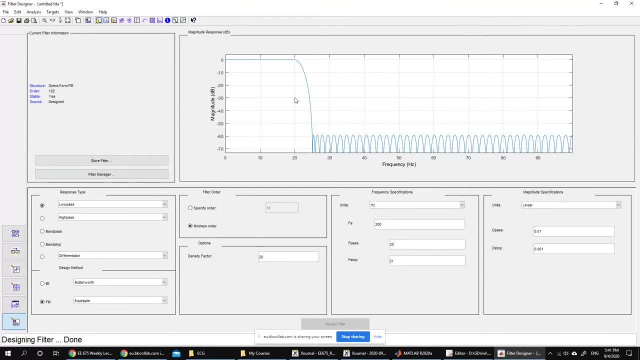 that is very steep between 20 and 21.. 20 passes, 21 doesn't. let's try to see. if we modify that, what would that affect the filter? remember that the order here is 102. see how it looks like now. the order now is 509. 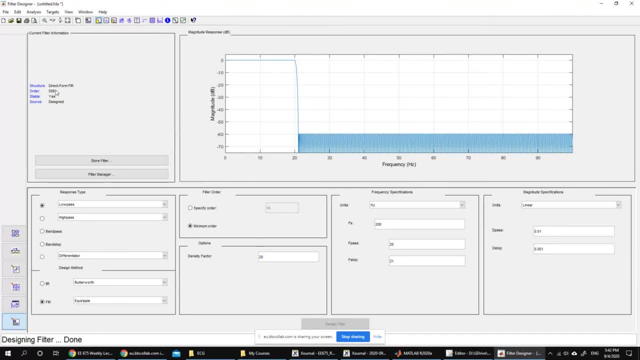 509. so basically it's just trying to get closer to the ideal filter, made the order basically explode. this is not a good thing. how about if you remember that we we would like to remove a 30 hertz signal? so basically we don't have to start the stop band from here. we can stop it at 29. let's try to have this as 29.. 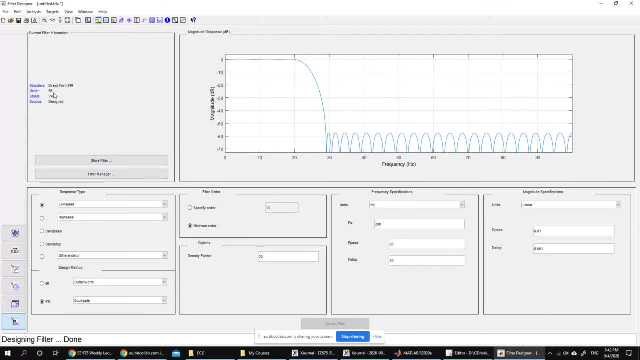 the order now is half what we started with. instead of having 102, we have now 56.. okay, and still, if you see, here, the 30 hertz will still be attenuated by minus 60 decibels, which is basically 1 over 1000.. okay, so basically, this would look like a much more efficient way of doing this. 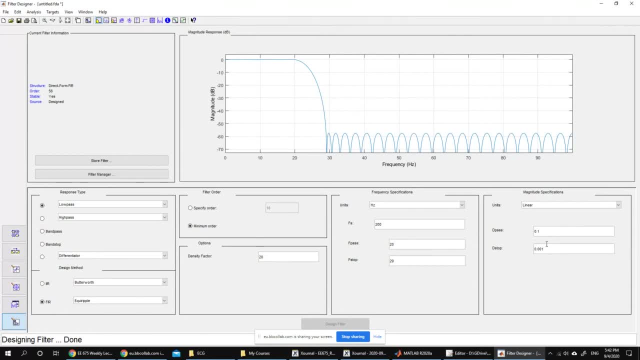 let's try to improve this. also, let's try to just change it to 0.1, like it was in the default value. okay, just basically. i'm going to allow variations here within 0.1. remember that the cutoff frequency, or basically that the magnitude, that the cutoff frequency. 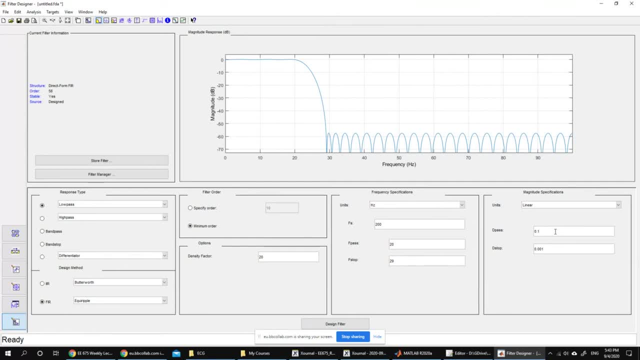 was 1 over square root of 2 of the actual signal. so basically it was like: basically it was definitely below minus 0.1 from the original one. so basically 0.1 should still be okay. let's see what that would affect, how that would affect the signal, basically here. 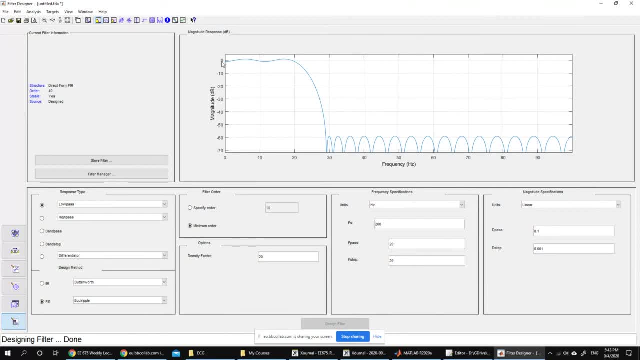 you have zero decibels. zero decibel means it's one, because basically decibel is a 20 log the value. so basically zero is 20 log one. so basically here in the bass band you have some variation but actually they seem acceptable. okay, if you look at the order here, you actually were able to instead. 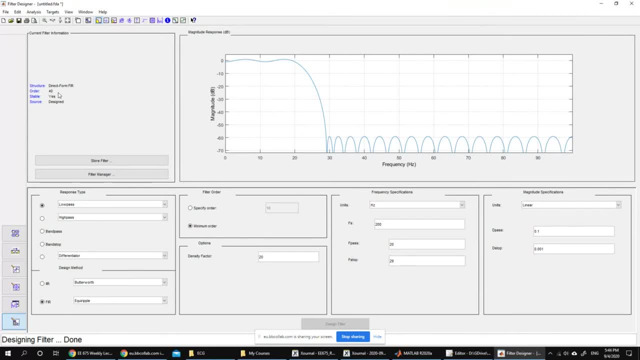 of having 56.. filter of 56, you actually went down 16.. so basically you have now an order of 40, which is really good. so basically these are ways of optimizing the filter characteristics so that you have the minimum order that you can get, because actually it's very important in some. 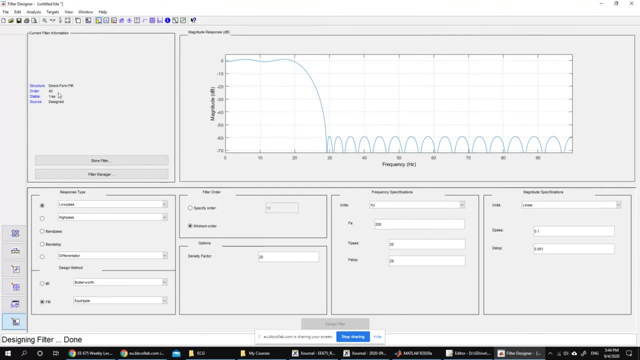 applications. actually, you have a limitation of the order that you can use because of the real time. if you want to calculate the output of the filter, you have to have it basically with very small order so that you can calculate the values very quickly and post the post them, or. 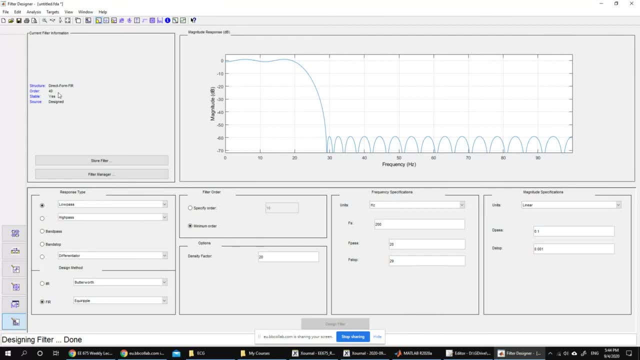 display the result right away, okay. so basically these kinds of things are the thing that we're going to be playing with, okay, and basically let's try this again with the, the decibel range. basically, in the decibel range, here you have one decibel and here you have like 80. 80 is like uh. 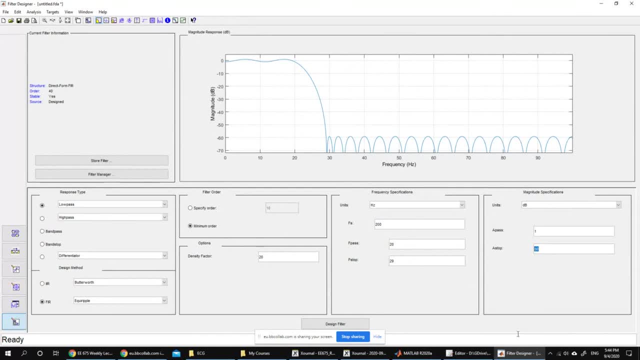 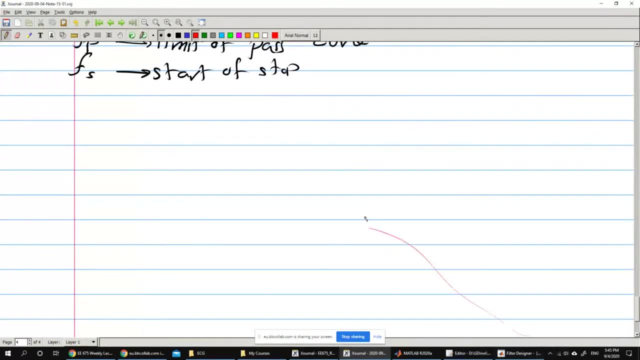 1 over 10 000. okay, let's go and discuss the decibel scale again. um, basically, uh, the decibel scale- sorry, uh, let me get that color here- the the decibel scale is 20 log amplitude. okay, meaning that if you have a one, have the amplitude here one over. let's just start with one. okay, 20 log 1. 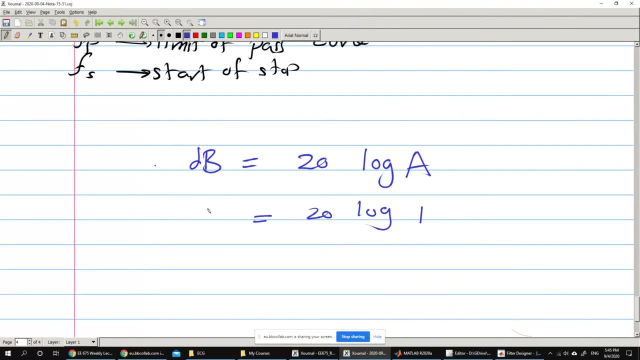 equals to what? 20 log 1? how much is log 1? log 1 is zero, zero. okay. so zero decibels corresponds to an amplitude of one. how about if we have 20 log 10.. one, okay, this is one. this is one time, so it's going to be 20 decibel. how about, uh, 100? 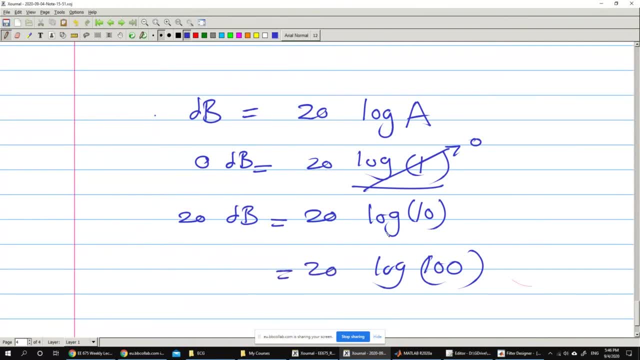 uh, it's become 20, 200. this is two, because basically log 100 is two. so remember that the log is basically 20. sorry, 10, log the number 40. the number is equal to a. okay, so basically log 100. yes, this is 40.. and the same. 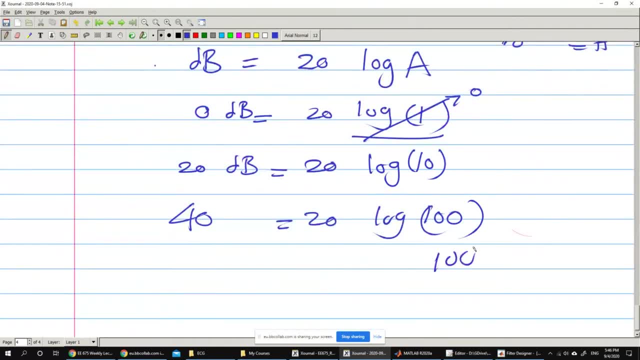 thing. you can actually see that the amplitude: when it's uh 1000, it's gonna be 60. when it's um 10, 000, it's going to be 80. okay, the thing is, if you actually uh instead of having the actual number here, if you have 1 over 100 or 1 over 1000 or 1 over 10, what's going to happen here? 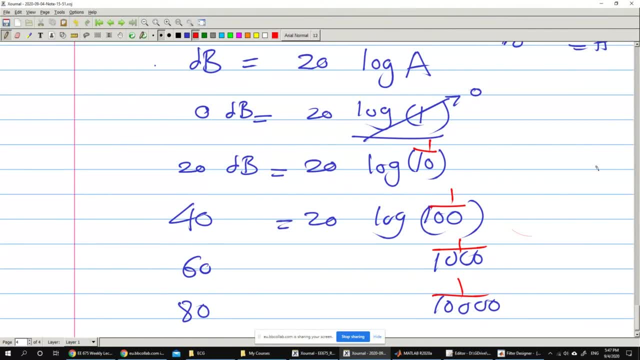 what's going to happen here? one over 10, it's become bigger than one over actually. if you just have, for example, uh, log y over x is equal to log x minus log y. remember that, yeah. so basically this will be log 1 minus log 10.. so basically this will be what minus. 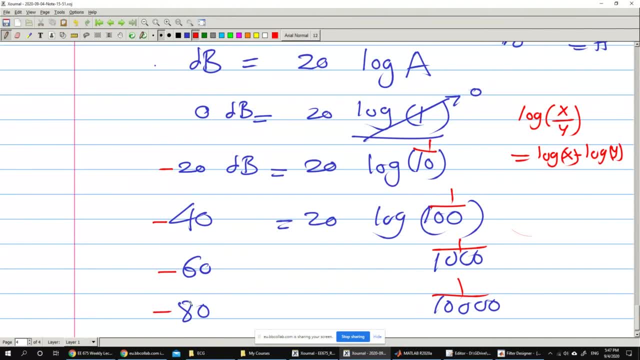 is that clear? yes, so usually in the filter context and digital filter context. if you look at a paper that talks about the filter, usually it talks about the specifications in terms of decibels, not in terms of linear scale, because actually this is much more commonly used. okay, so basically in what we saw, matlab, 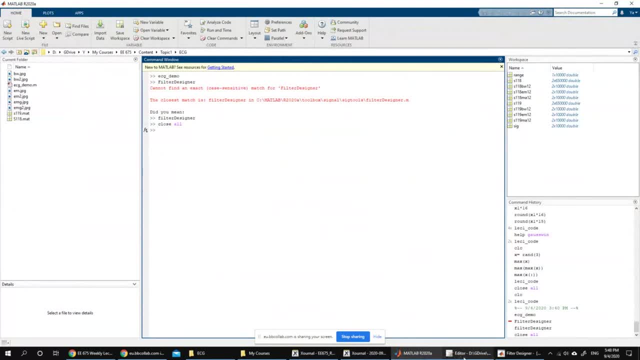 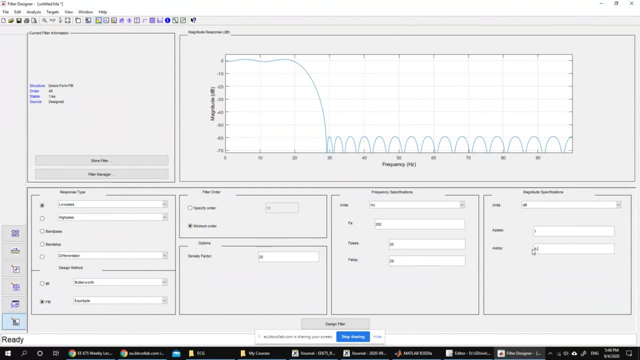 we're going to basically we can. we can actually do the same thing in matlab. basically, instead of putting here the, if i want, for example, one over one thousand, i can put here 60. and the one here is okay, i can also put a number that the one is. 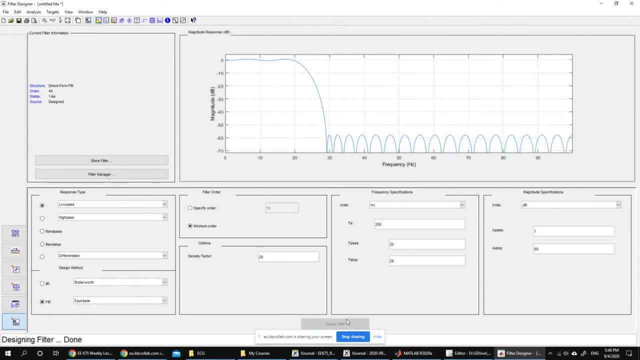 should be okay, because actually it's within the three decibels. so basically you have variations here for about one decibel and the 60, and the order is about 44, which is okay. how about if we try this? you would like to take this filter and use it? 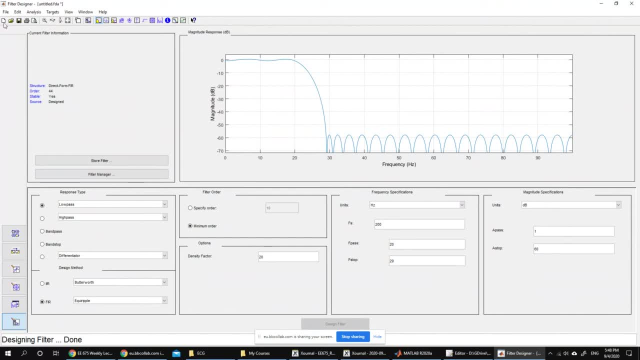 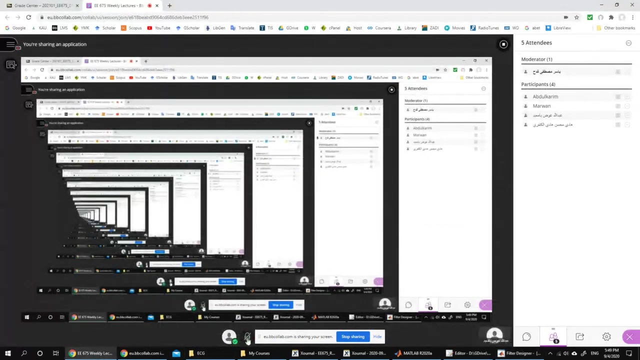 okay, in order for us to do that the simplest way, in the same exact filter designer, you have something called the automatic filter. in the same exact today, you will have something called export, basically export, generate MATLAB code. okay, you can generate the filter design function. okay, I prefer if you use that. okay, just second. just second. I'm sorry. 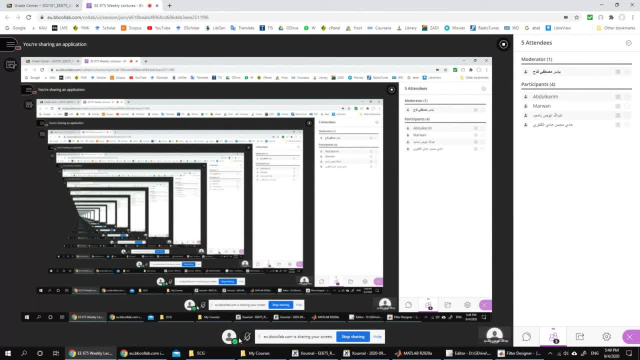 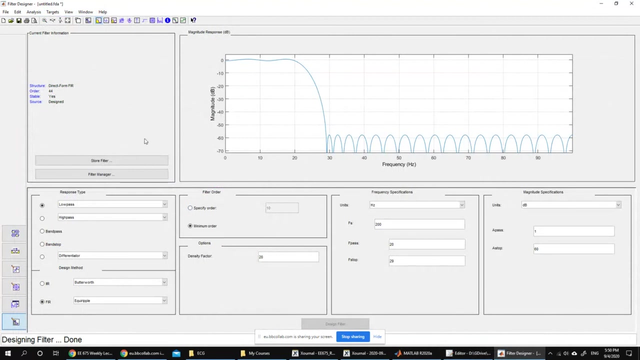 you doctor? yes, yes, you, okay, I'm sorry. so basically, what I'm going to do now is try use base generate the filter. just try to use this filter and basically simulate some signals and try to see if it works or not. so basically here, as I was saying, 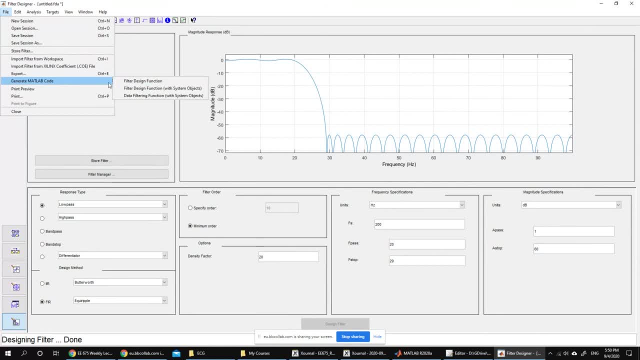 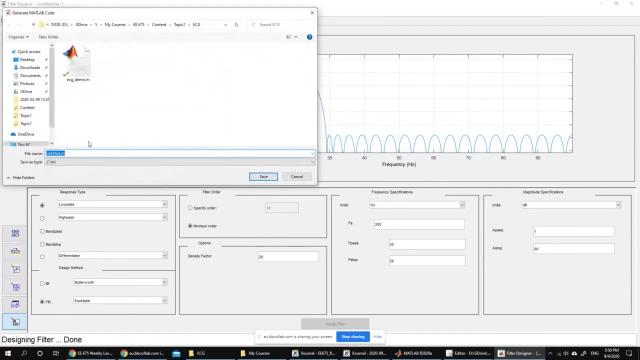 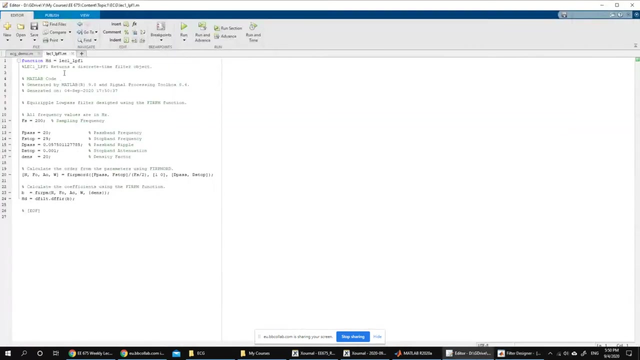 we're going to use, generate MATLAB codes and basically you say you select the selected filter design function and select any type of filter of your choice. I'm going to show you the interpretation of the code in general and which are the internet. so basically, I'm going to select that, I'm going to call it. 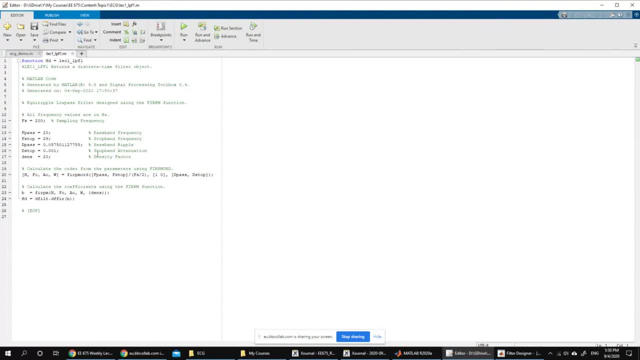 let's just call it lecture. when NP LP f1- okay, let's call it any name. okay, what happens is that is gonna open it for you like this gota. so, basically, in order for you to be able to use it, you can either use it as a function like this: 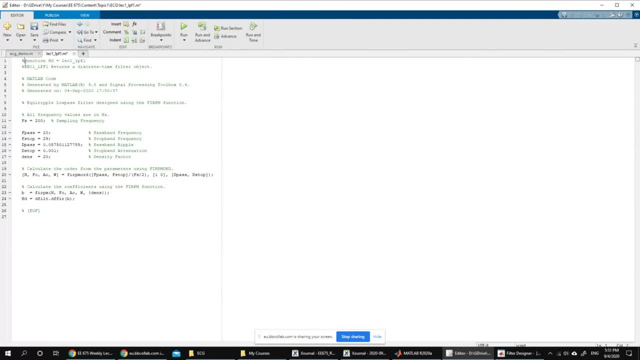 but actually the easiest thing is just comment this function and continue your code here. so, for example, here i'm going to generate two signals, one of them is 10 hertz and the other one is 30 hertz- okay, and then apply that filter to these two signals. okay again, i'm. i'm actually taking 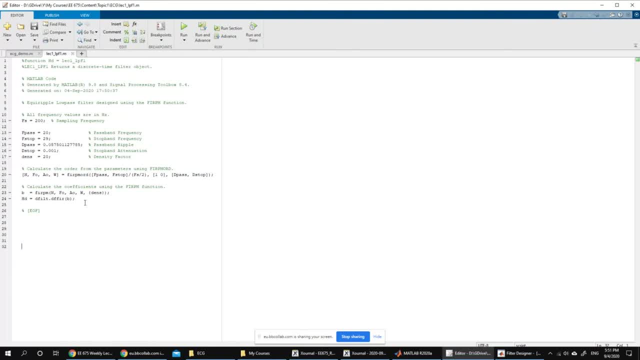 you quickly on over this. so so, basically, you can actually uh, uh try things yourself without understanding much of what you're doing, but actually you're going to be uh trying things, okay. after you try things, when i get to talk about the theory, you're gonna understand it in a much better way. okay, because actually you know how it looks like and you will. 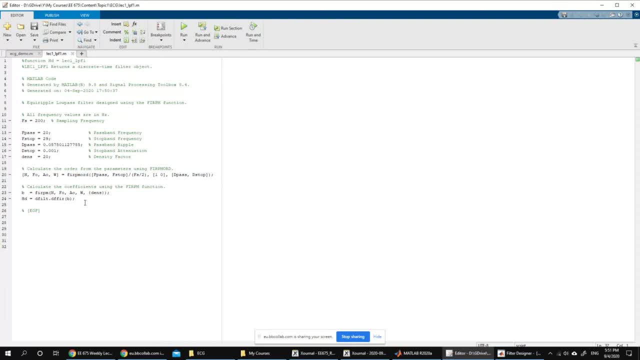 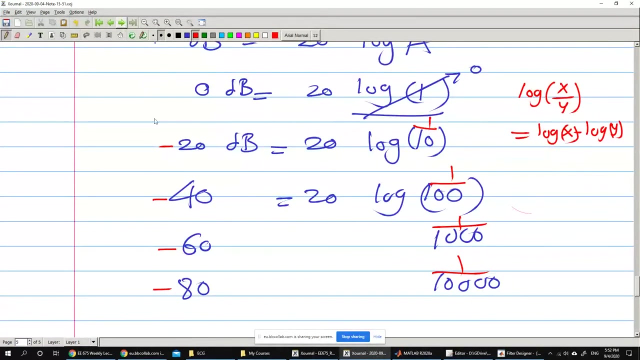 know that, uh, basically, what to expect or what, what you will need to know from the theory, okay, so, basically, i'm going to generate two signals now. okay, in order for us to generate two signs of the signals, let me go back to the editor, to the this part here. uh, i want to know how to generate 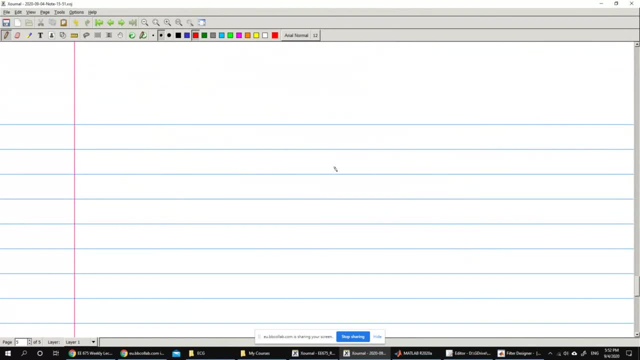 two signals, two signs of the signals. basically, the general form of any sinusoidal signal looks like this: basically, if you have a signal uh, x of t, maybe i should select a different color. so the signals are either sine or cosine, or e to the power or e to the minus, g, omega. okay, 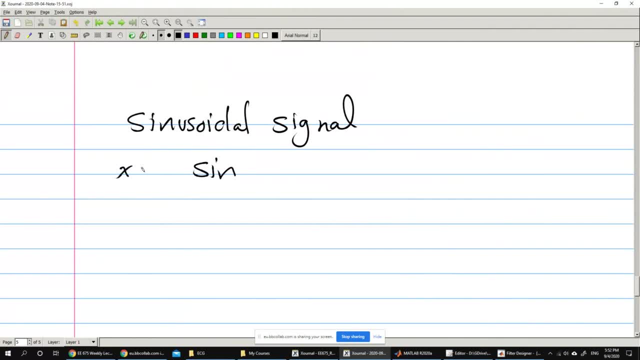 so basically they are all the same, but actually let's just take it as sinusoidal. okay, the general form is: twice pi, f times t. this is the time version of the continuous time version. if i wanted to get that into a discrete form, what i need to do is basically: 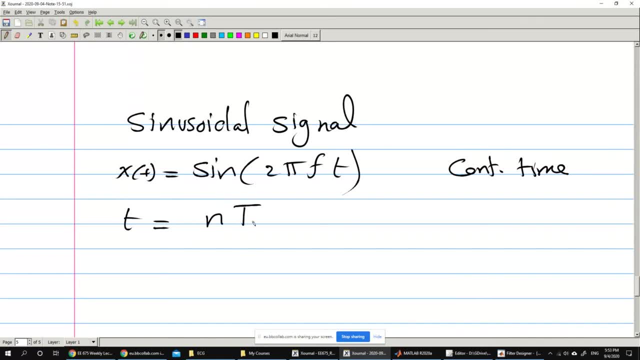 select the time points that are equal to n t s, where t s here is what sampling period is. so, basically, if you have a sinusoidal signal, you want to take it here, here, here, here here, take it in certain points, and actually each one of these points is separated by t s from the from. 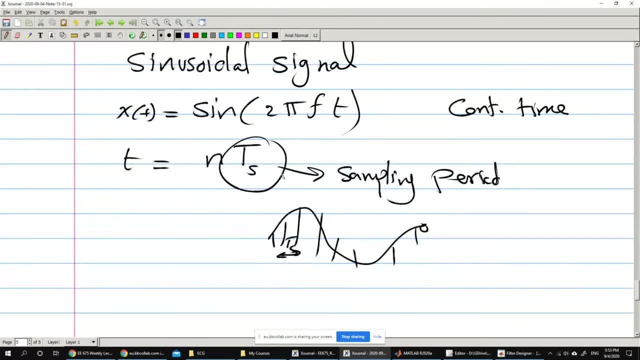 the next point. so basically, if i use n here the number, n for the, the n here zero, one, two and so on, okay, if i do it like this, if i basically substitute here by nts, then i'm going to get a discrete version of x. so basically, this is going to be x. 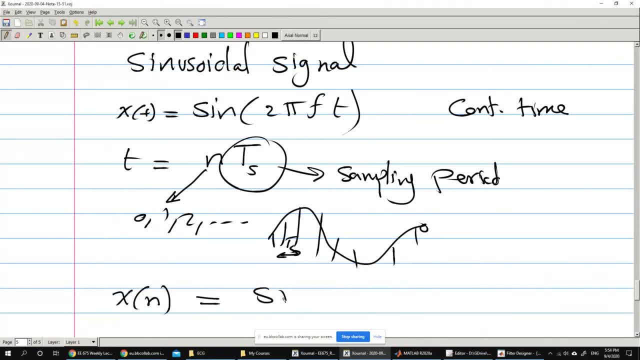 of n equal to sine twice pi, f, which is the main frequency, or f node. let's just call it f node. this is a frequency of the sinusoidal signal times, n, ts. okay, so basically all i have to do is just put f node with whatever i want and ts with whatever i want, and basically have n as zero. 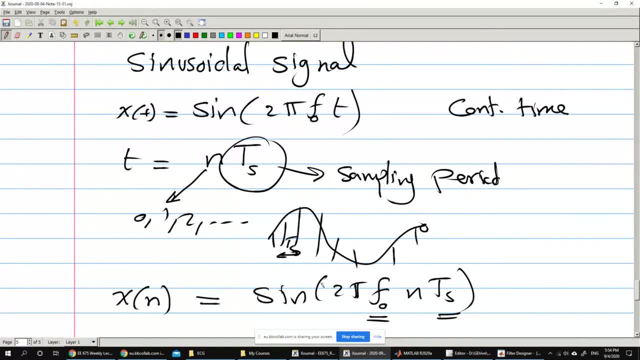 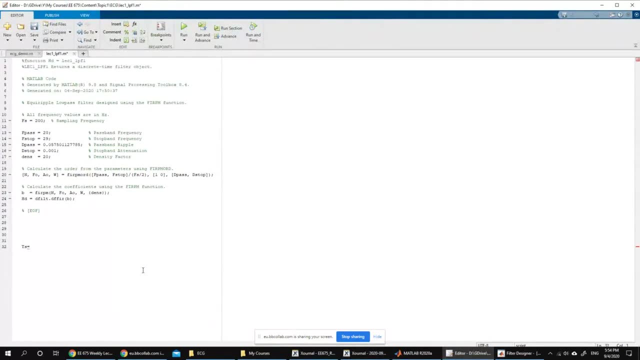 one, two and so on. let's try to do that in MATLAB and basically basically generate the signal and display it also, just to make sure that we did it right. so basically what i first will do is basically let's just put fs. the sampling frequency that we put in MATLAB was 200, right? 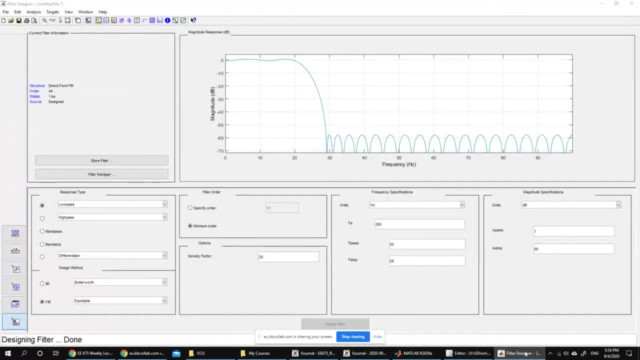 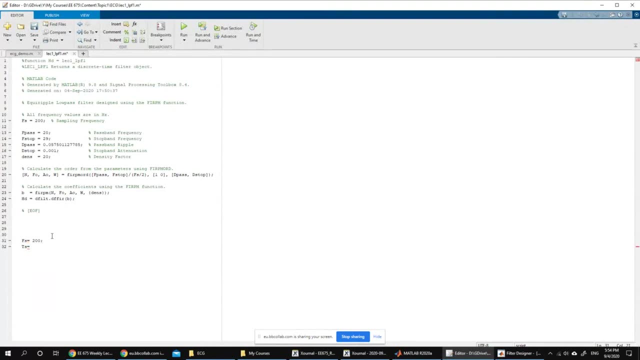 200, right, okay, so basically, this is the sampling frequency. i'm going to try to document the code that we generate here so that when you read it, when i upload it for you, you understand what it means. this is a sampling frequency, which is the sampling frequency, exactly the sampling frequency that we use here. 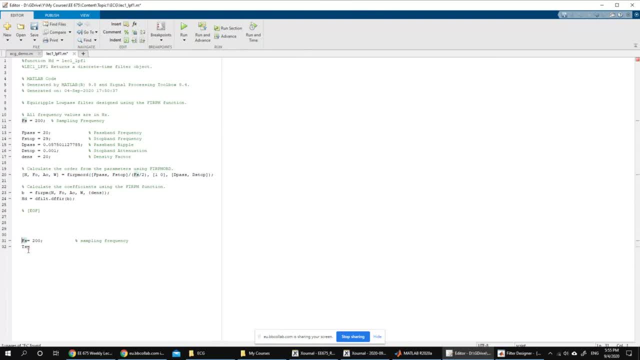 see here, it's already there. it's already there, so i don't have to put it actually already up here. okay, ts is basically one over fs. this is the sampling period. we're going to need that to generate the signal from nts. and let's take n, or let's take: a number of n is equal to, for example, 100. 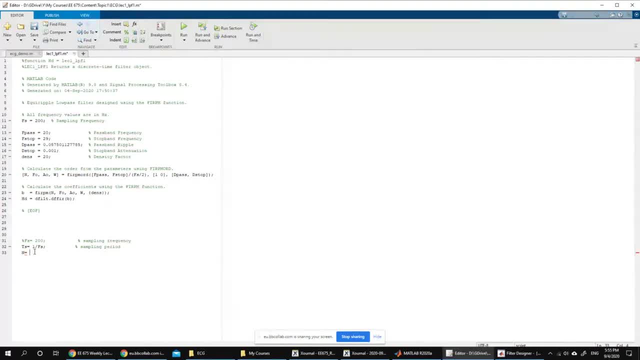 or maybe this will be 10, maybe 200- okay, and you can actually change it. this is the number of points, basically the we're going to draw the signal. so basically we're just going to take this number of points and basically generate them and change any one of these and basically n- small n, which is a time variable, that the 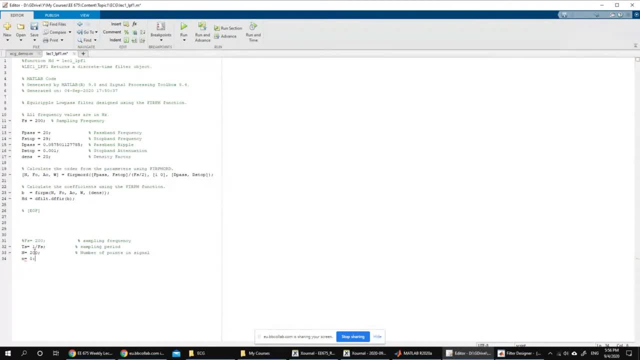 discrete time variable will be from zero to n minus one. this is the discrete time variable. time variable S1, which is signal 1, let's just call it signal 1, would be equal to sine 2 times pi. pi in MATLAB is pi basically times f. f we can select. 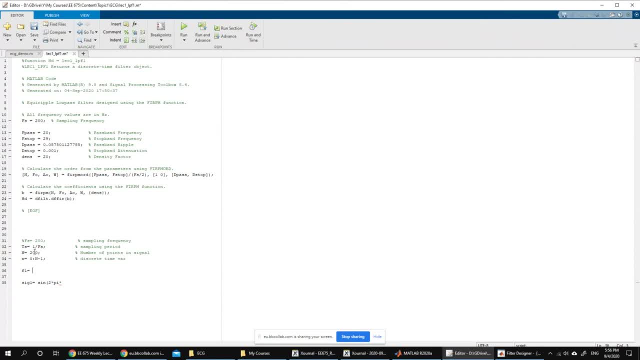 basically f1 for signal 1 equals to n, which is 10 Hertz. f2 is equal to 20 or 30, which is the second signal that we talked about. So signal 1 is equal to f1 times n times Ts, exactly like what we had in the last example. So signal 1 is equal to f1 times n times Ts, exactly like what we had in the last example. So signal 1 is equal to f1 times n times Ts, exactly like what we had in the last example. 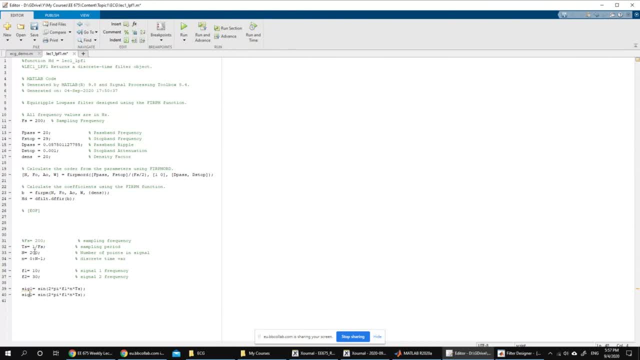 Basically you gotta do the same thing for signal 2, but just add, just change f1 to f2, okay, And then say that sig. okay, maybe sig x is going to be basically sig 1 plus sig 2.. Okay, let's draw these, Okay. so basically I'm just gonna generate a figure, and I usually 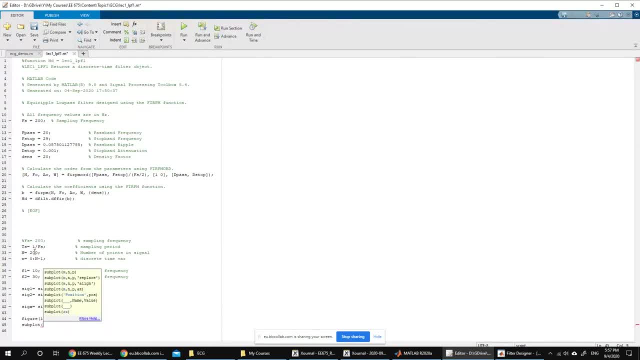 prefer to use subplots so that you have multiple plots in the same figure, so that you can see all of them. So let's consider that we have. basically, you're gonna draw the first signal, the second signal, the summation and basically you 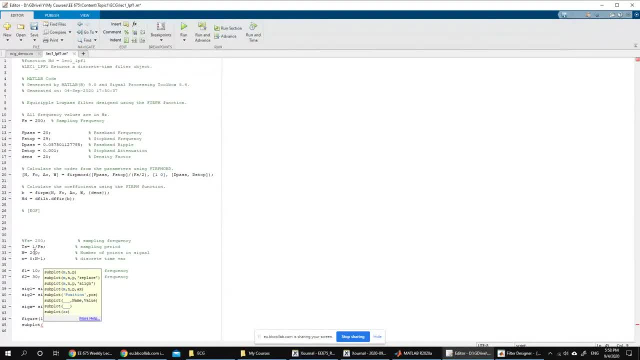 can have also the filter after we apply the filter. Okay, so basically in the subplot here we generate a matrix of 4 by 1 figures inside that figure and I'm going to draw in the first one, Let's say plot. 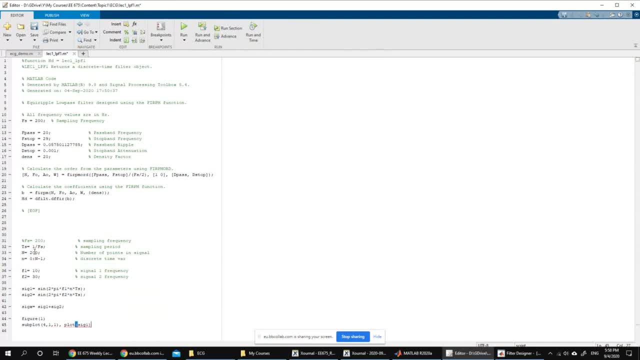 Let's say plot of sig 1. Usually it's better to just use n, because actually it's x and y basically for the plot. So n is basically the time variable. so I'll use it like this. So I repeat this. 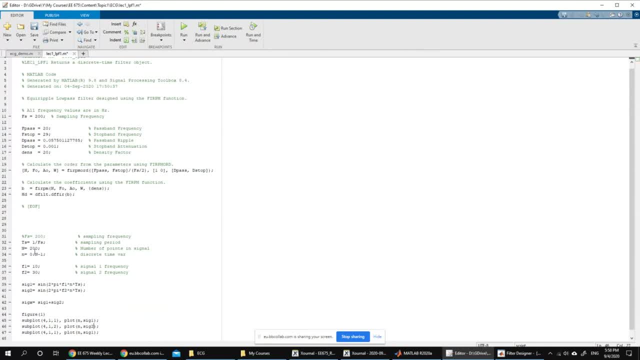 For the second slots, I'm going to draw signal 2, and for the third slots here, I'm going to draw signal 3.. That's the summation signal, Let's. let's just run it and run that and see what comes out. 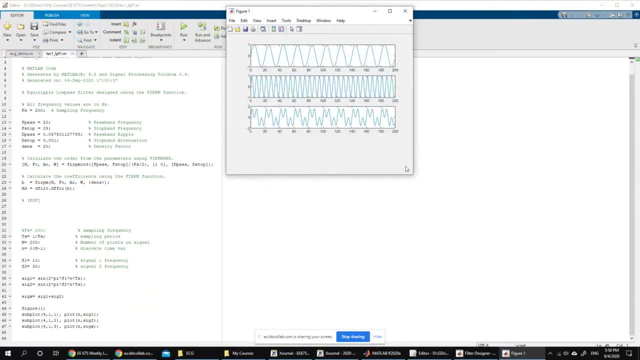 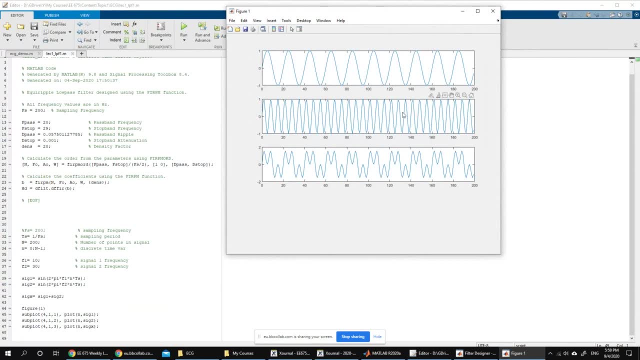 See, here Is it clear for you. You have the first signal, you have the second signal, you have the summation that looks like this: Okay, what we need to do now is to take this signal here and apply the filter that we designed. 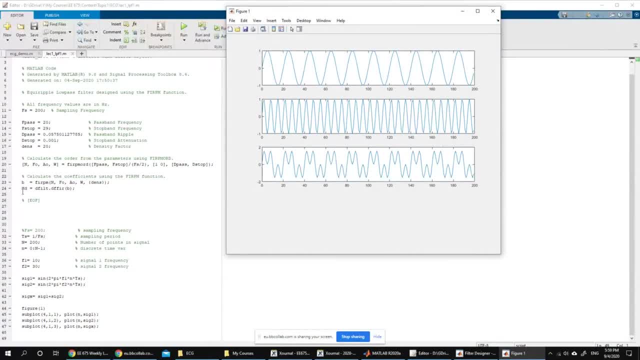 here out as hd. basically that's a format for the filter. we're going to talk about it when we describe the theory of the filters a little bit more next time. but basically we're going to need to take that filter here and apply it to the figure, to the signal, this signal here in the figure, and basically 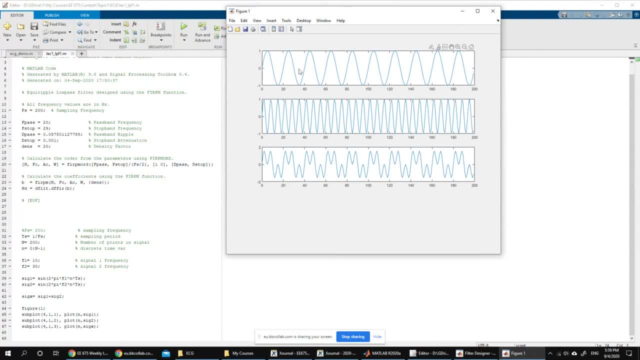 come up with a filtered version that hopefully would look like this one here, if you see that basically this is low frequency, this is high frequency, we have a cutoff frequency in the middle, so basically it should remove, completely remove this signal here and basically we get something that looks like this: okay, let's try that. in order for you to apply a filter. basically there is a 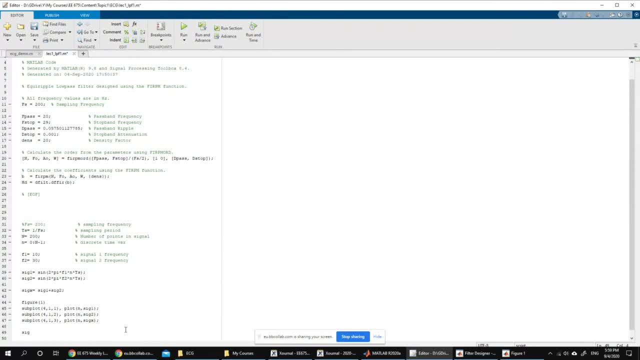 function called filter. okay, very simple. let's just say sigf, which is filtered version of the signal, will be filtered, and basically you put the filter that you designed and the signal. that's it, okay. and then what we're going to do is basically just draw it in the four slots. 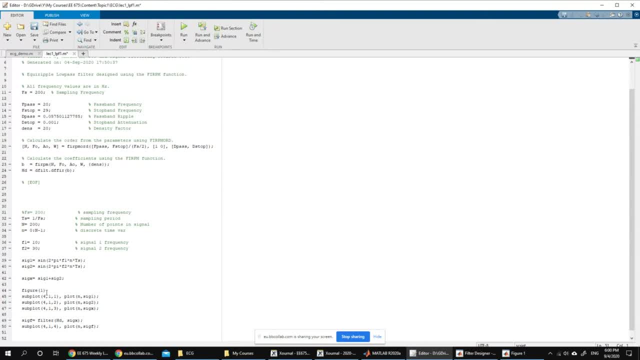 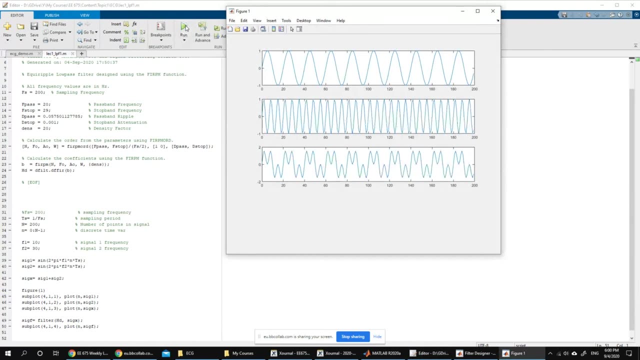 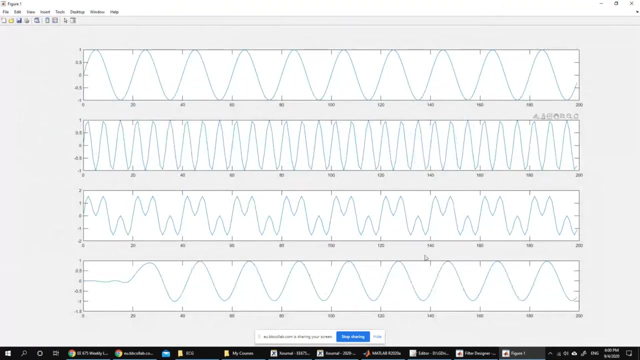 okay, let's try that. so basically here, in addition to just drawing the filters or the signal that i simulated, i basically i'll filter the uh summation and basically draw the filtered version of the summation. let's see how that works. see here. what's your opinion about that? any observations about the output? is it good? 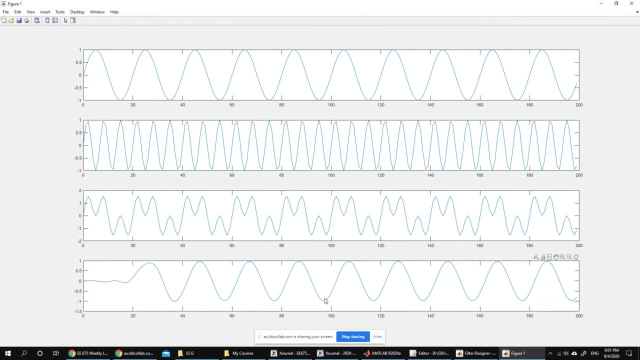 does it look good? does it look okay? does it look like what you would expect from a like this? the beginning from 0 to 20.. from 0 to 2: 20.. yes, exactly, this is actually. this is a transient. basically, if you have, if you remember, if you. 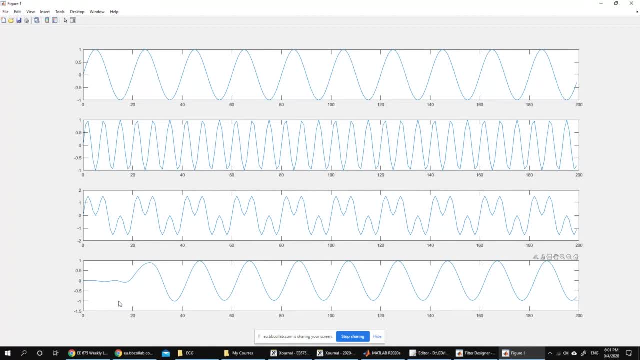 remember the circuit uh problems that you used to solve in your undergraduate you you would remember that you have two components of the response of a system. you have a transient response and you have the steady state response. the transient response is temporary and basically after a while it dies out and basically what? 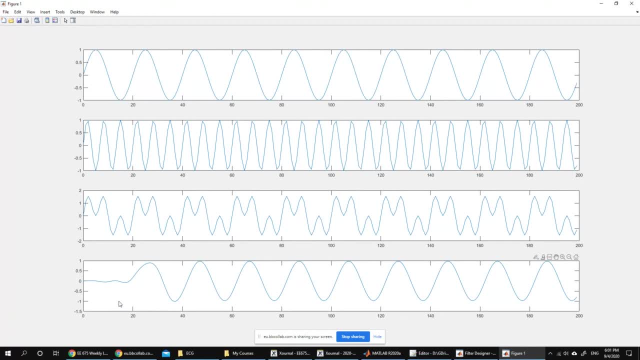 remains is the steady state response. what you will see together is that this transient response actually is relying or relies on the order, the order of distance, the what, any questions? okay, so basically, at least in this part it looks okay. so basically, the state part of the filter looks okay, but the first part. 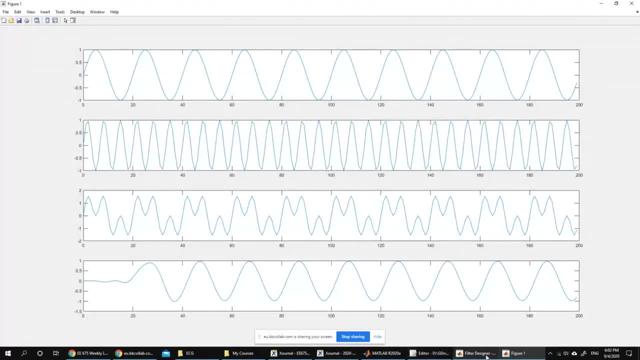 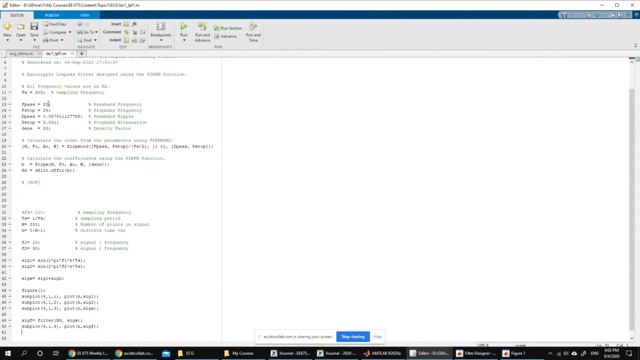 doesn't look okay, let's go back the advantage of using the filter design function here instead of just using a function. basically, you can vary if we can change the values here. so, for example, if I change, if you remember, if you we have 21, let's take a 25 percent, 25, okay. 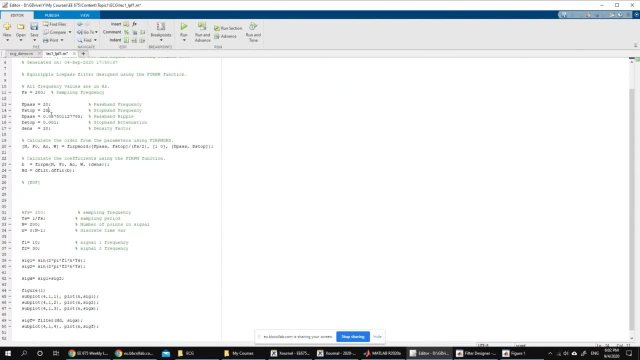 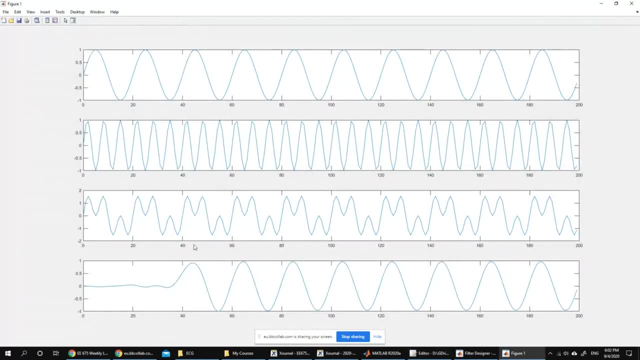 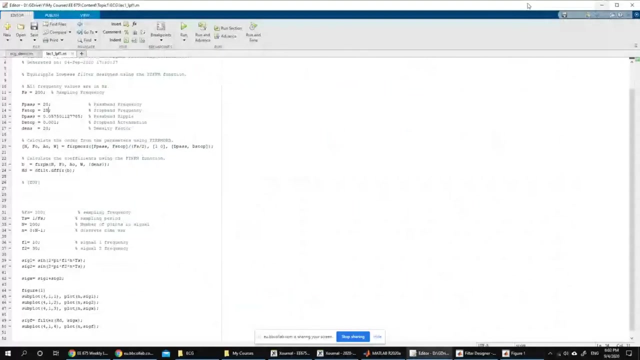 25. if you remember, the order of this filter was almost 100, right, let's try it like this. so basically, I change the stop band from 29 to 25, let's see what happens. it's become bigger. so this is imagine that. if I actually add it, if you make it. 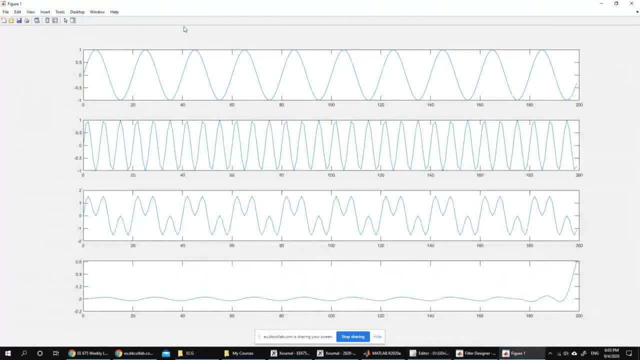 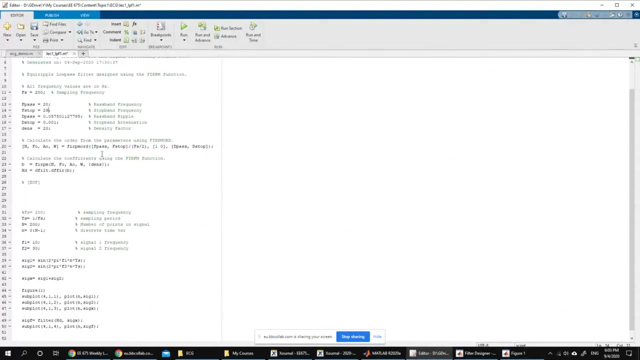 like 21, okay, like we did before. see what's happened here: actually see 200 points and basically didn't even reach the state within to the first 200 points. okay, changes a lot. okay, changes things a lot. okay, let's go back, make it like 29, like we used to have, okay, and just make sure that it's still okay. I'm. 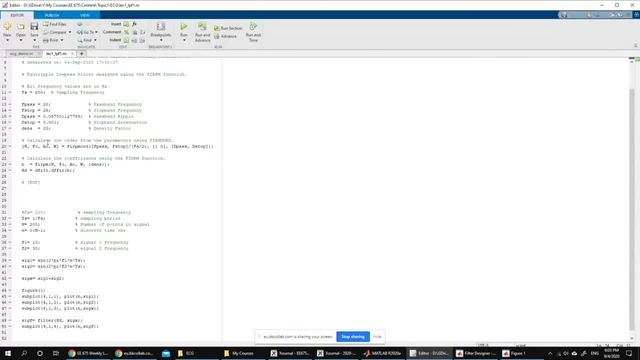 going to change now the part about the attenuation. let's just make it like 1 instead of 1. okay, point 016: enforcement. so basically let's actually I wanna. okay, actually here is old, or basically. I just wanted to change a little bit. maybe I can just write it here. all the way up doesn't really matter. no problem, cause actually this is basically the first layer, but you just have to wait for it to be shaped and then, once you donc tires, it's all right, good job, next workout, let me go back. maybe i should just go back to me so that I can actually use all the values on normal. 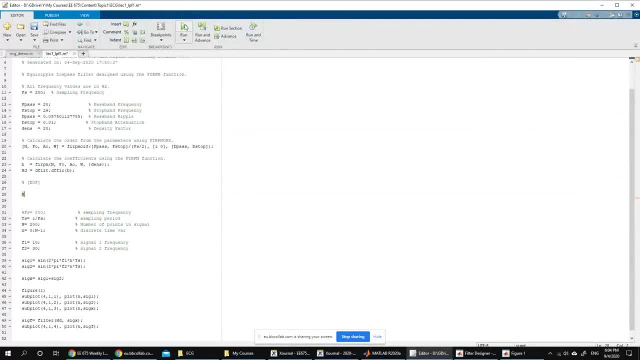 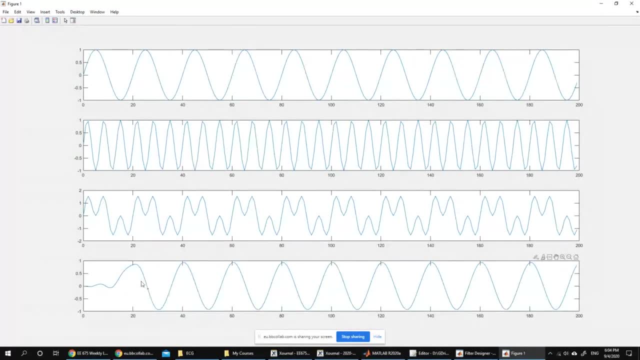 and just just to see the order of the filters. okay, so basically this is a filter. now it has some transient here, but actually do you see any variation? do you see any problem here? this is actually a much smaller filter. see, here the transient becomes a little bit smaller, if you remember. 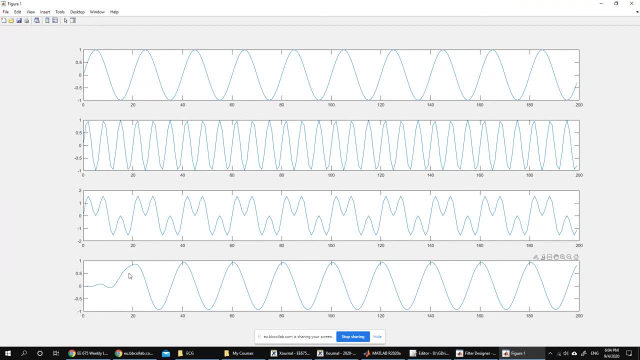 it used to be like here: start here. yes, right, right. so basically it started a little bit earlier. so basically the order of the filter is smaller now because actually i made the constraints on the filter, made the demands of the filter a little bit less. so, okay, what's? what's happening? 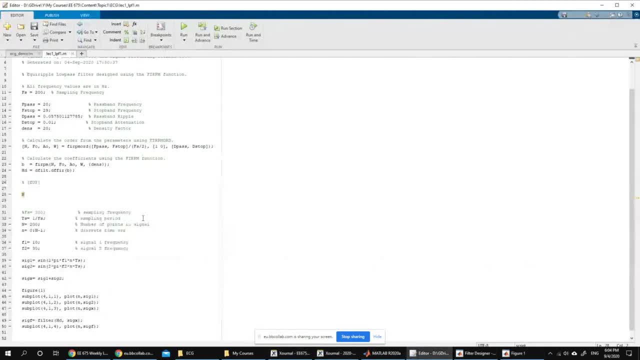 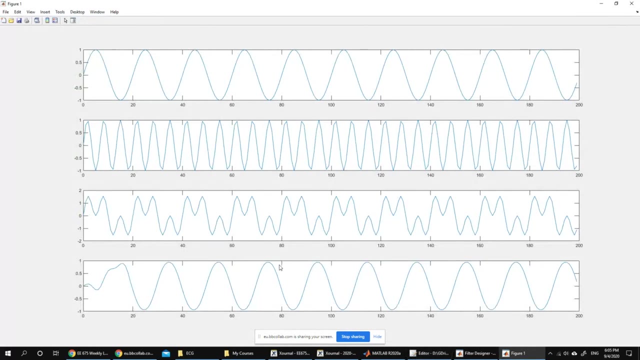 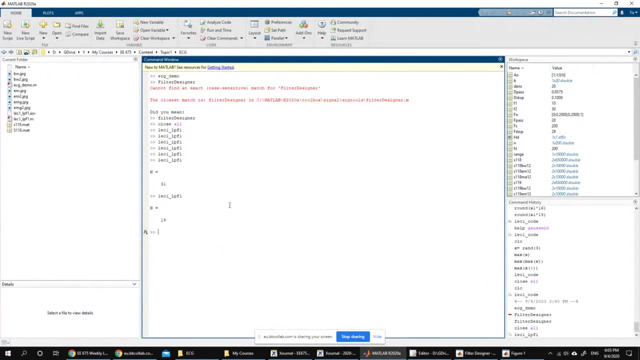 fine, but let's try to do that. okay, we can do that. if we make it 0.1, please stop make it 0.1. okay, this is 0.1. please stop make it 0.1. okay, but actually, let me just make sure. the order now became 19. 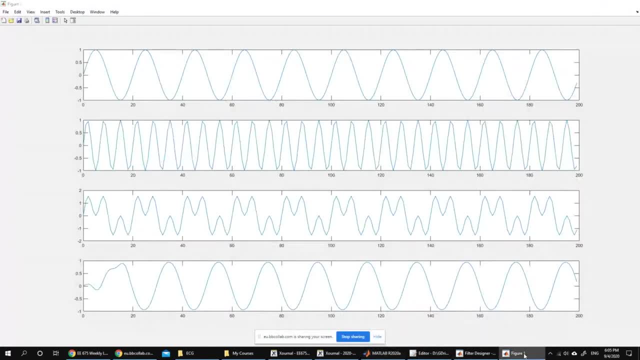 okay. so basically, uh, in the figure here you started from a little bit earlier, even okay than the one, the one before. but actually, if you look at this, if you, the signal actually looks okay. but sometimes, uh, when the artifact, when the signal with the artifact, is a little bit. 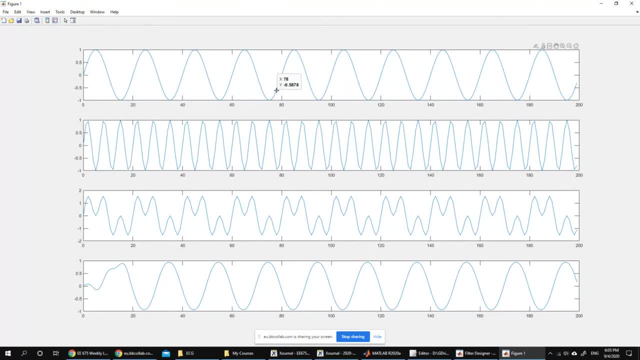 large, larger than the actual signal, like, for example, if you have emg, then you will have a problem with this because actually 0.1 of a signal, that is 10 times the actual signal, the true signal, would make a problem. but actually i have to justify or have to. 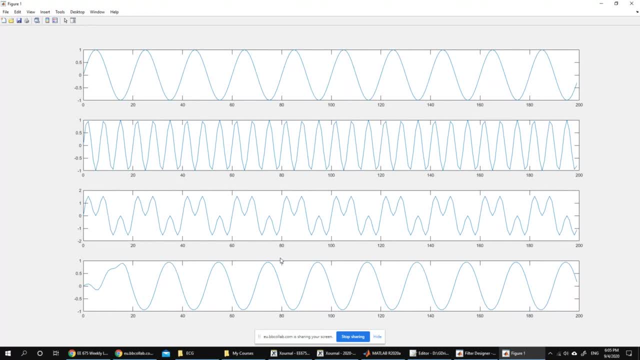 basically investigate that by experimentation. so basically i cannot say that all filters must be- must be at least 60 decibels, for example. no, you have to actually try and see if 40 would work okay, and so on. so basically it's, this is the experimentation part. so here actually we saw that we relaxed. 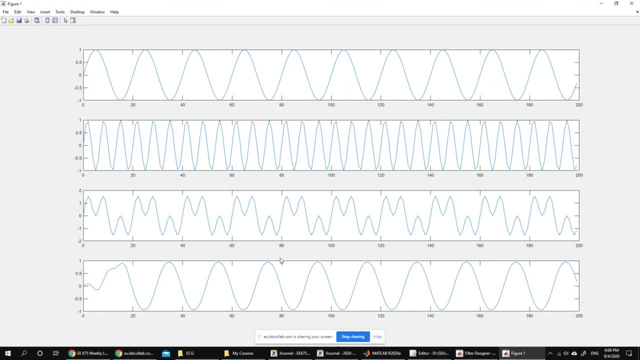 things a lot, a little bit, and we still have a very good signal, so this should be okay. so this is the the kind of experimentation that i would like you to do, and whenever we get started with this part, you will have a filter design function like this: 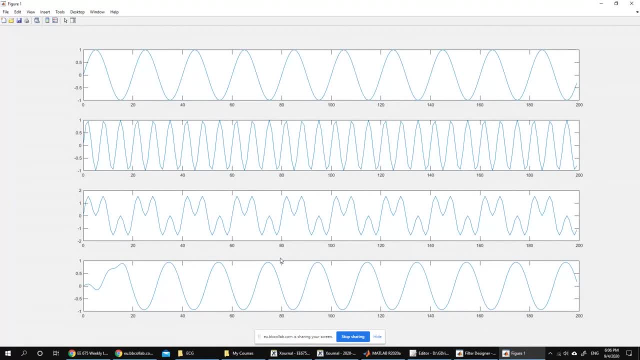 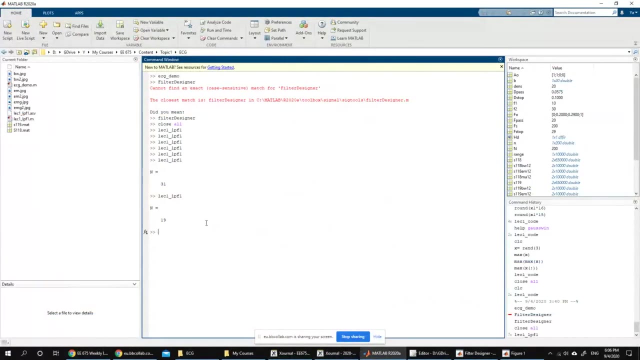 and you just keep changing the parameters and checking the output and making sure, uh, whether it's acceptable or not. so here for me, actually, this is very much acceptable. so, basically, instead of having a filter with 500, like the one that we we saw, that we designed from. 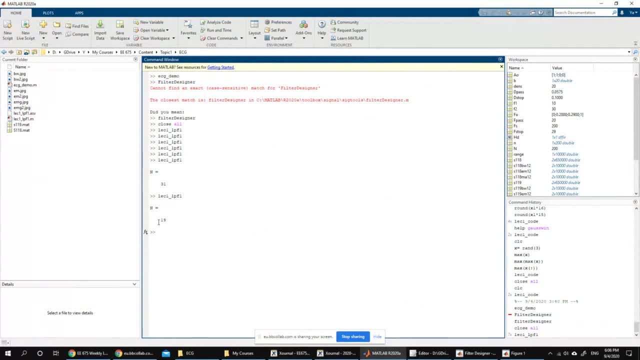 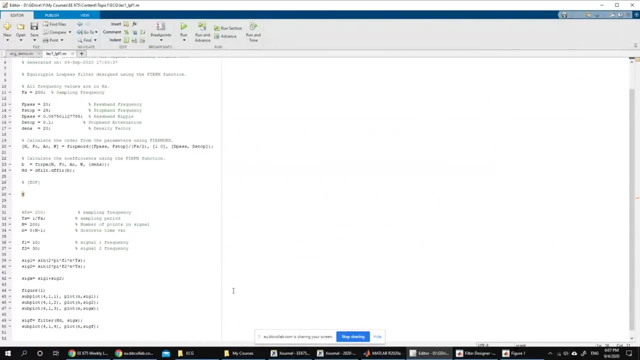 you know, a short while ago, we actually ended with something that is acceptable, with an order of 19, which is great, actually, okay. so basically what i would like you to do, just to make sure that you understand what you're doing. basically try to repeat whatever i did. 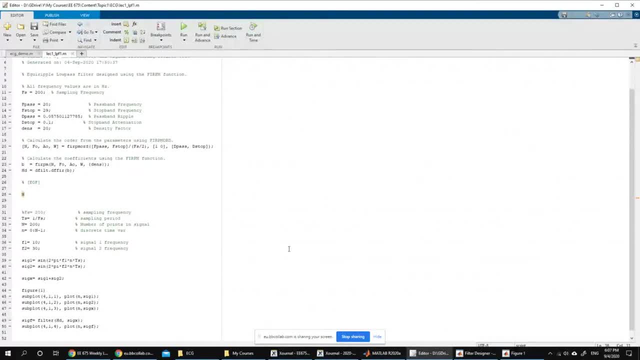 okay, okay, but i want you to actually do exactly the same, that basically go all the steps that i did and generate the design function and then basically try to play a little bit with these kinds of parameters and see what happens. um, you have any questions about how to do that? 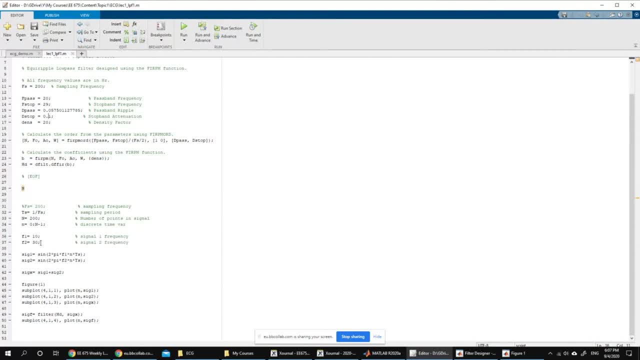 and basically you can use these two signals. basically i can. one of the things that we can do also is just play a little bit with these two signals. maybe you can make this like 20 and see what happens. one thing is 20 and the other signal is 30. okay. 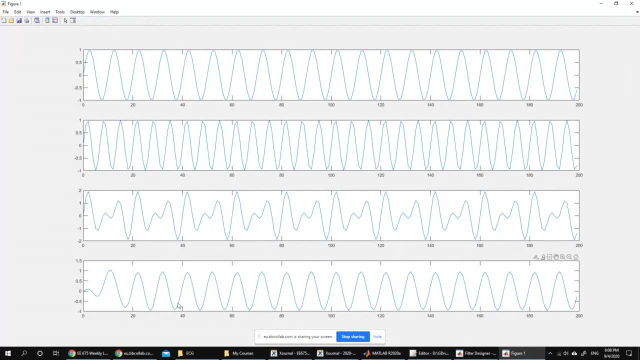 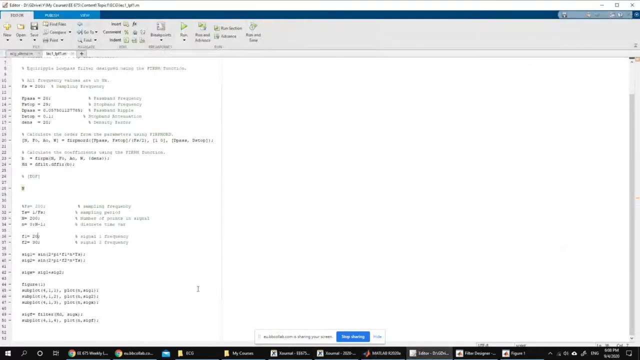 uh, it looks a little bit different because basically, you see, here you see some attenuation in some part of the signal, so it's not exactly the same. okay, let's try to have, for example, um, let's just take this back to 10 and basically put the other one here as 25.. remember that we have the, the f star at. 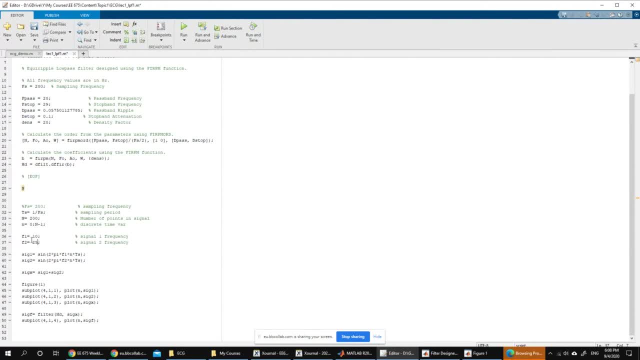 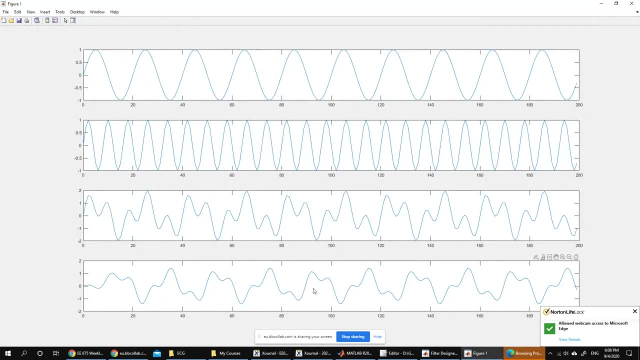 29.. okay, so basically this is before the step stop. so the attenuation of this will not be the what we put right there. it's not going to be 0.1, it's going to be a little bit less. see here how it looks like, because this actually the signal here actually was. 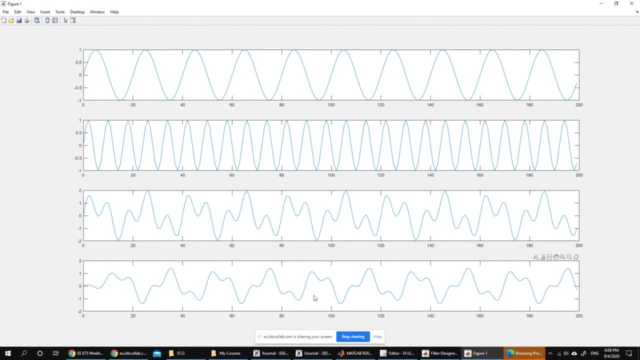 not, uh, in the stop band, it was basically into the transition zone. when you have something in the transition zone, you will have something that will actually uh, uh, not not get attenuated sufficiently to to be able to, uh, uh, do the proper filtration that you designed. okay, so basically, uh, let me change this back. 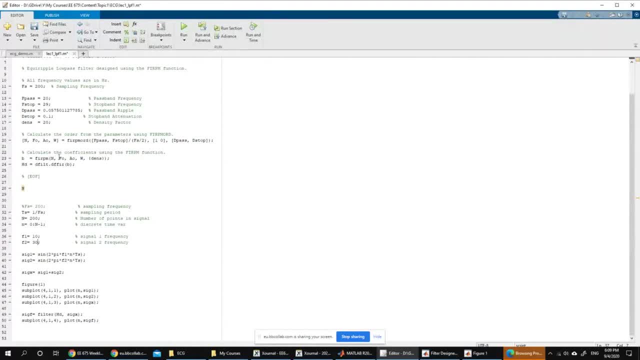 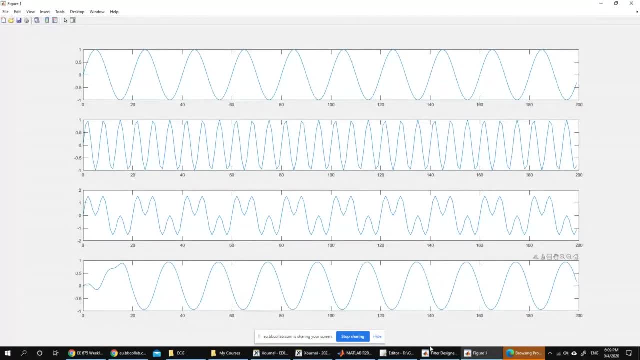 to 30 and uh, let's run it to make sure that it's okay, because this is the version that i'm going to post for you. so basically, this should be okay. so i'm going to post this version for you here and basically, uh, stop at this point this time and basically: 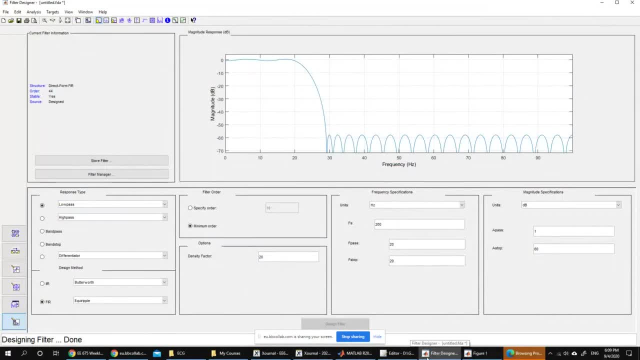 uh, start next time with some more experiments with digital filters, and i'm going to explain to you the theory of digital filters, okay, after you actually had the chance of trying things and basically imagining. uh, at least the part about the transient. it's very difficult to imagine if i talk to you at the theory of the transient. 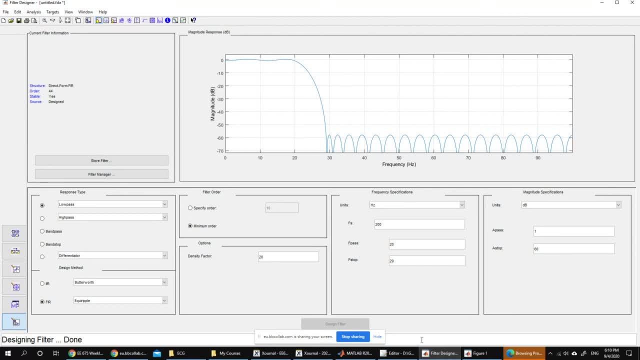 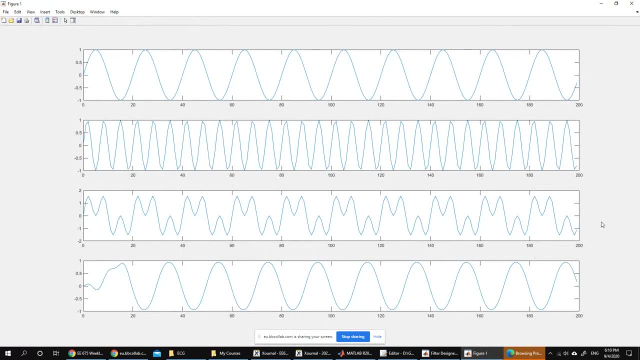 you will not know exactly what i'm talking about unless you saw it yourself. okay, so, basically, next time, what i'm going to do is, uh, do some more digital filtering and basically, uh, yeah, apply the theoretical analysis to whatever we had in the experiments. okay, so, please, uh, try to do exactly the same things that. 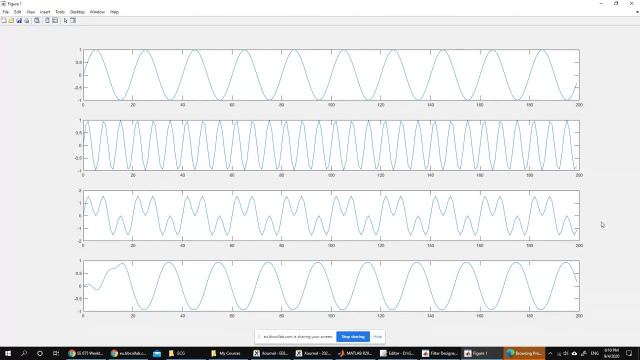 we did this lecture, uh, by yourself. if you have any questions, please do not hesitate to basically ask me at the beginning of the next lecture. we do not have a time schedule or a particular amount of material that we have to cover. the most important thing is for you to learn how to do things. 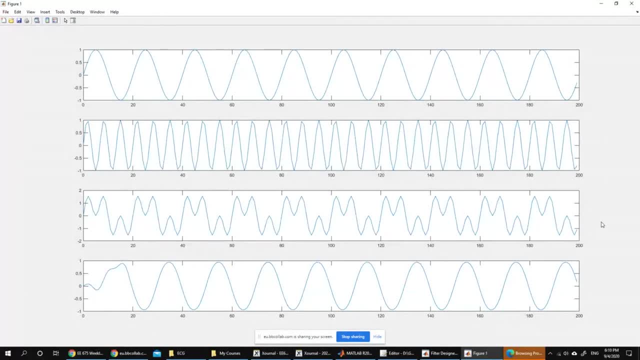 basically, if you just focus on one topic and learn through that one topic, you know a lot of tools. that would be sufficient. so, basically, we do not have to rush or do not have us to finish a certain topic within a certain amount of time. feel free to ask. 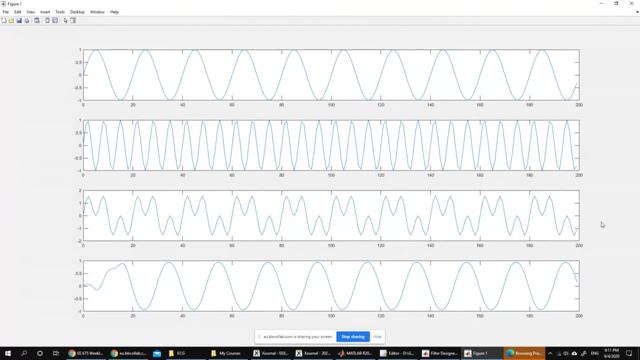 me. if you want me to repeat things again, it's fine, okay, so basically i'm not going to go much further this time. i just wanted to get you started on at least some experimentation with matlab and basically next time, inshallah, we will continue. i don't want to have too many things today without some. 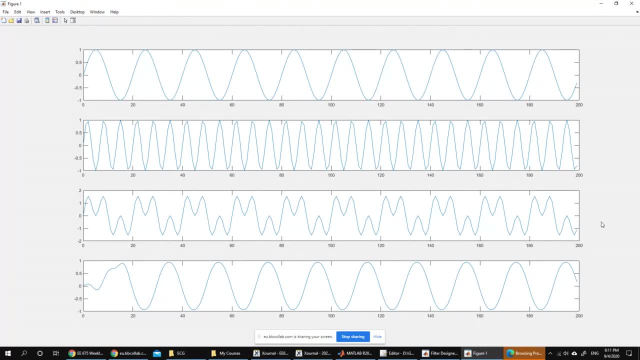 of you, with some of you don't have the matlab, and basically hopefully next time, inshallah, everyone will have matlab and basically we'll have the chance to go through the experiments so that we can continue to build, build on that a little bit more. okay, doctor, can i act, or something? 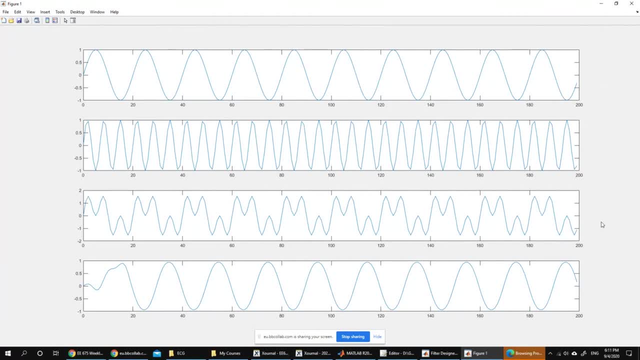 i can hear you. yes, this is objective. i haven't registered this because a 20- 20 minute conflict with another course. i have been told to change the schedule schedule of this course from audis. so if you don't mind- and uh, it's a chairman who can do that- i can't do that. 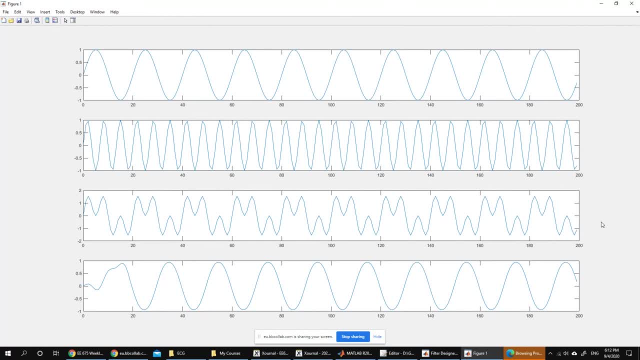 you have to talk to the chairman, you have to send to the chairman about this. i don't mind, because basically we have, we have our own schedule, okay, so put it wherever you want, wherever you want, but actually make sure that you don't have conflicts with other- uh, other courses. 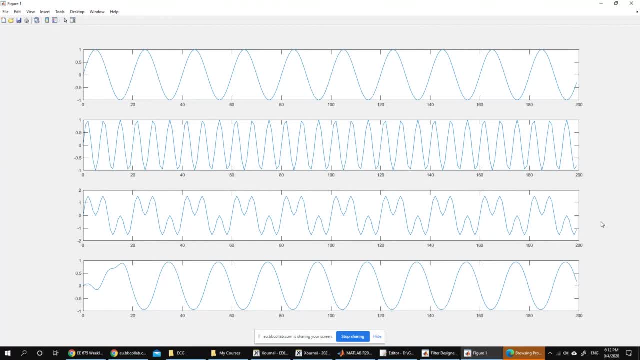 yeah, so that you don't cause a problem for for another colleague. yes, Yes, just as far away as possible. Okay, okay, just put it in the morning. Okay, just put a schedule in the morning so that it doesn't have any conflict. 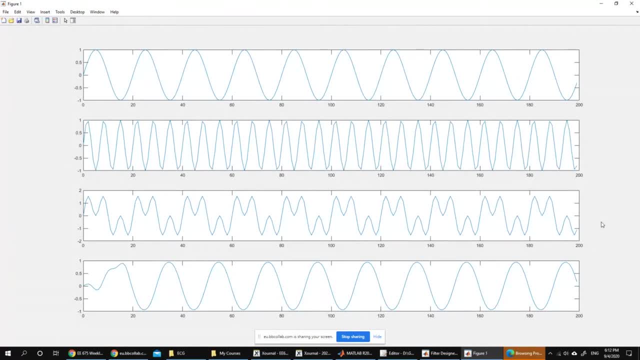 with any graduate courses. Okay, Okay, do you have any questions? If you have any problem with the pace, if you have any problem with how I explain things, any problems with the material, you don't have the background for we can actually at least give me the feedback. 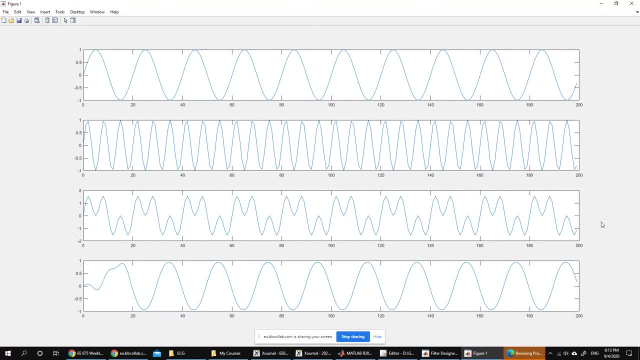 so that the lecture will be most useful to all of you, okay, So don't hesitate to let me know if you have any issues. okay, Can we find the this lecture with the blackboard? You have problems with blackboard? No, no, we don't have. 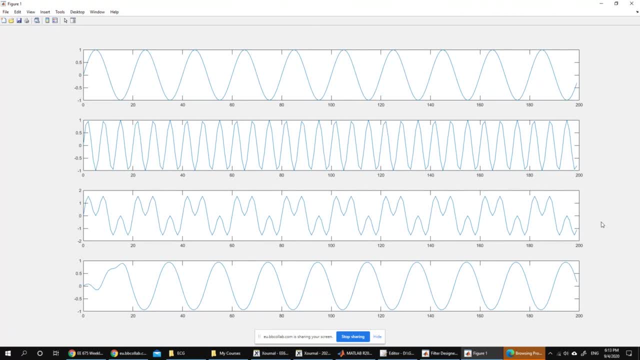 When exactly We will be behind this lecture. your explanation of the blackboard After you finish the lecture. I'm going to post it. I'm going to you mean the lecture itself. Yes, yes, Usually what they say, that is that after the lecture. 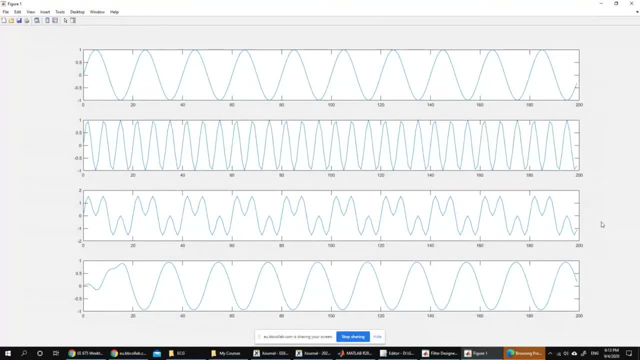 six hours after the lecture, the video will be posted, The material, the MATLAB, the MATLAB code basically within MATLAB, and some handwritten notes. basically these things are gonna be uploaded, maybe tonight, Okay, So, basically- Okay, thank you. So basically everything would be by the morning tomorrow. 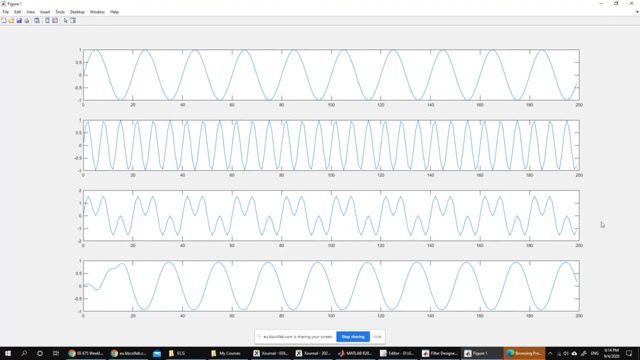 you're gonna have everything posted on blackboard. Okay, so- You can get the lecture and the material and the video. Okay, If you have any problems, just let me know also, okay. Okay, Simon, Did you get to the blackboard directly, or what? 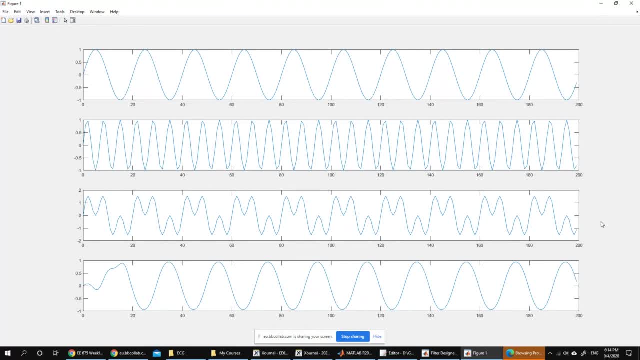 Yes, everything is on blackboard. So, basically, whenever I ask you, whenever I will ask you to submit an assignment, there will be an assignment on blackboard so that you can submit, okay. So the thing that I tell you, like today, I tell you to experiment with some things, okay. 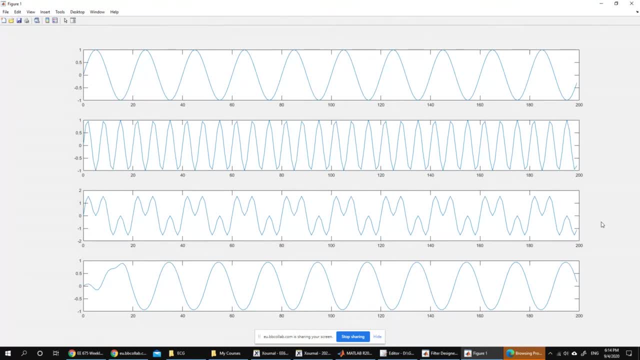 You do not have to submit them, okay, Just ask me if you have any questions. Whenever we have to submit something, you will find an assignment where you can submit that particular task. okay, So everything will be through blackboard, Okay. 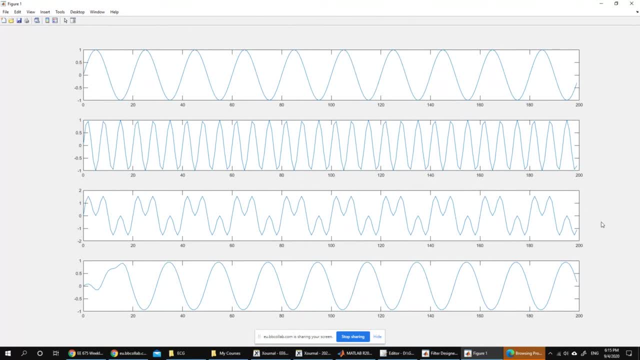 Okay, Okay, sir, Okay, So I'll inshallah talk to you again on next Friday. inshallah, okay, Thank you very much, Inshallah, Thank you, thank you, inshallah, inshallah. 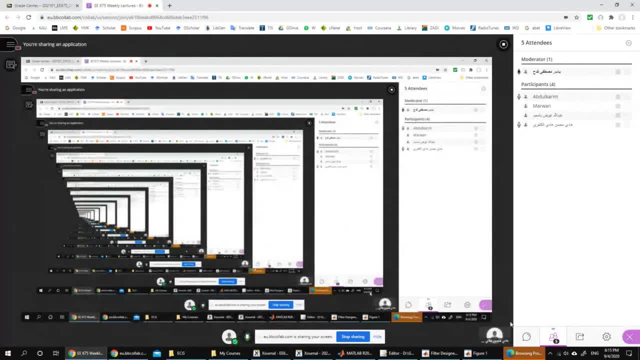 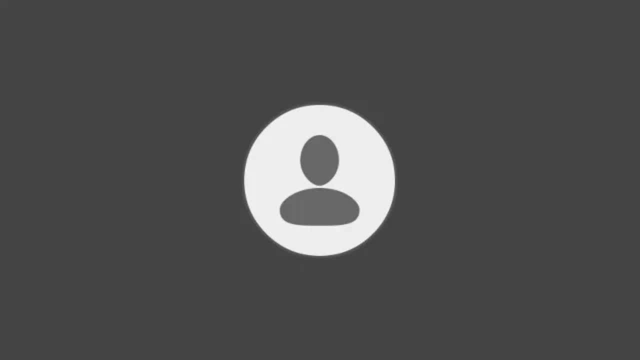